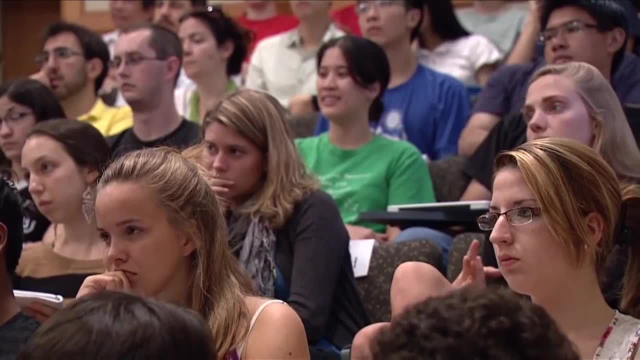 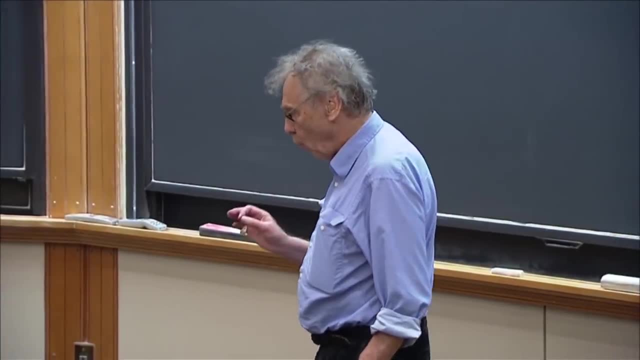 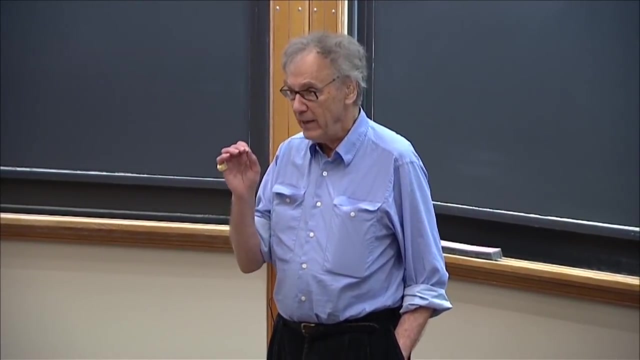 Regardless of whether that would be 1 inch or 0 inch in length. if this was saleable, then the probate would only be 1 inch long. In 1911, the English physicist Robert Rutherford demonstrated that almost all the mass of an atom was located at its center and was 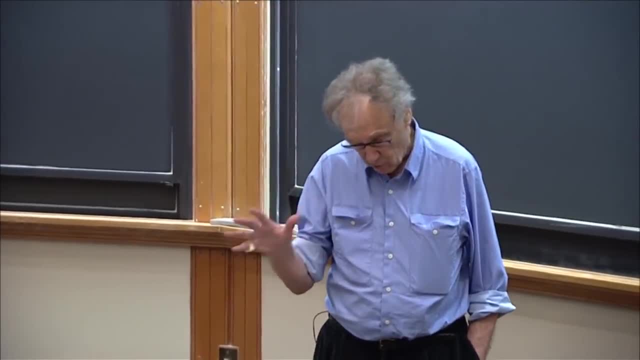 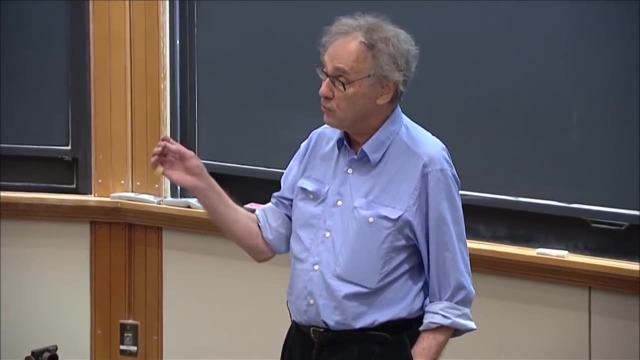 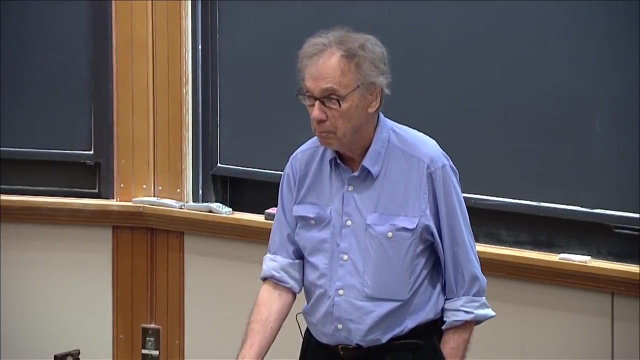 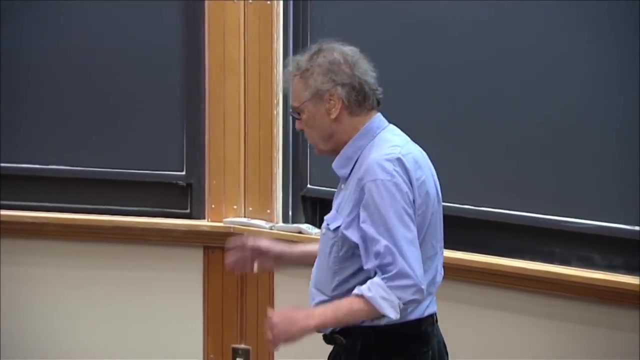 extremely small And there are electrons that appeared around it, The nucleus, which is positively charged. negatively charged, the nucleus is 100,000 times smaller than the size of the atom. If I suppose, for the time being, by scaling up this room- and I assume that this is the 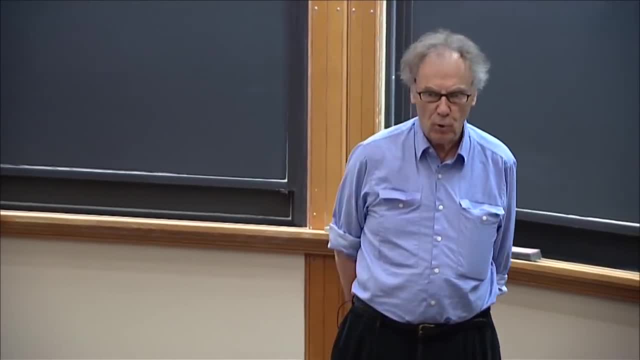 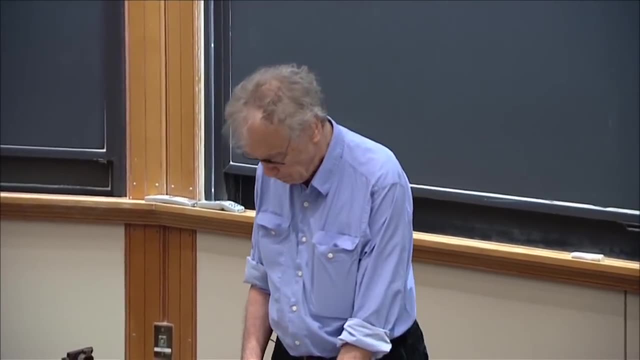 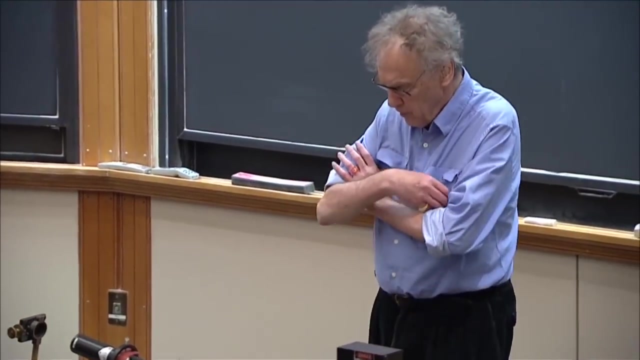 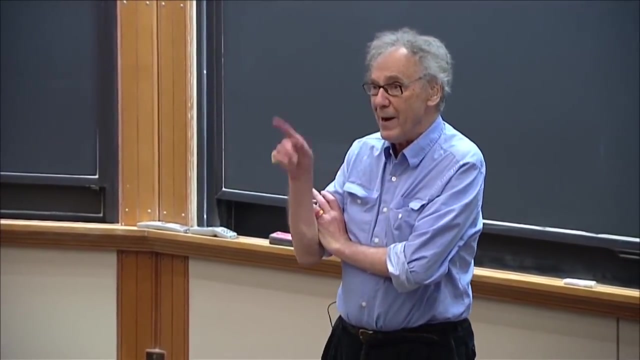 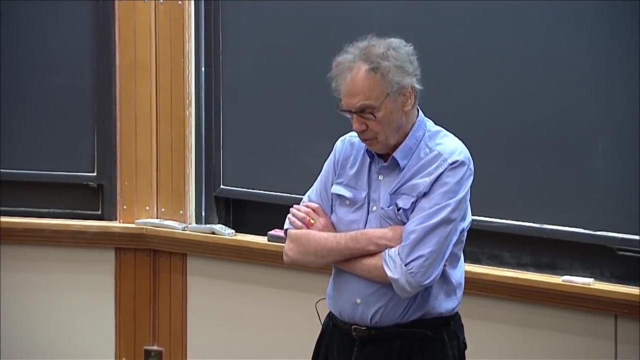 size of an atom, then the size of a nucleus would be about a grain of sand. That gives you an idea of the ratio 100,000 to 1.. According to Maxwell's laws of electricity and magnetism, the negatively charged electrons should spiral into the nucleus, which is positively charged, in a minute fraction of a second. 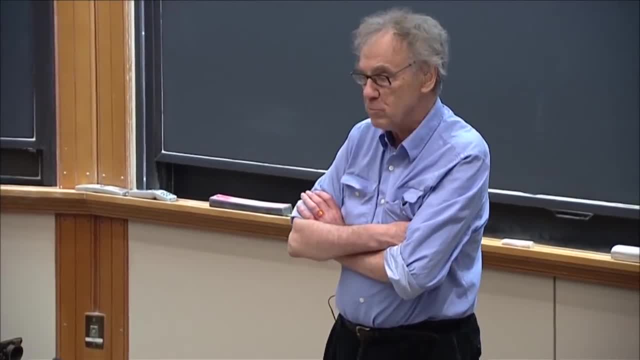 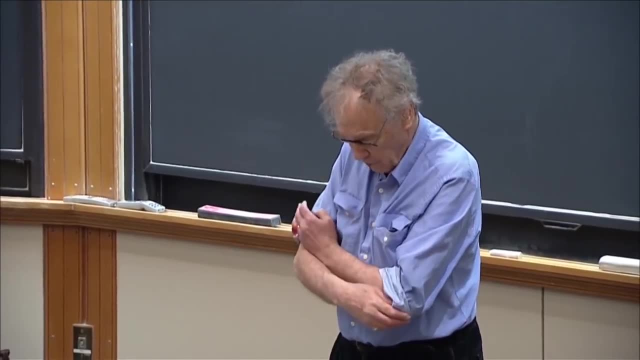 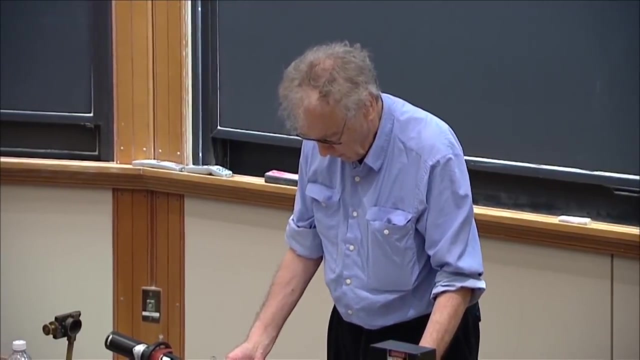 And clearly that's not what's happening, Because atoms do exist, And if they would spiral in the electrons, they would not exist. And so the Danish physicist Niels Bohr, in 1913, came up with the idea that the reason 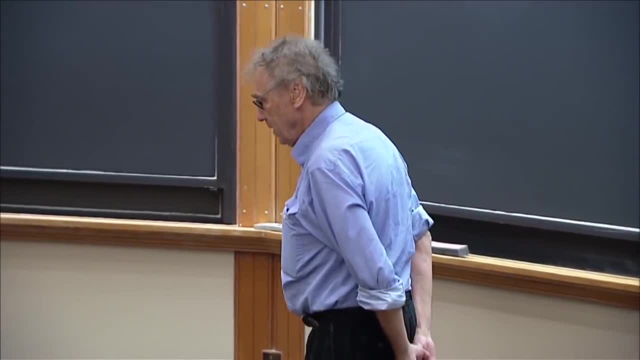 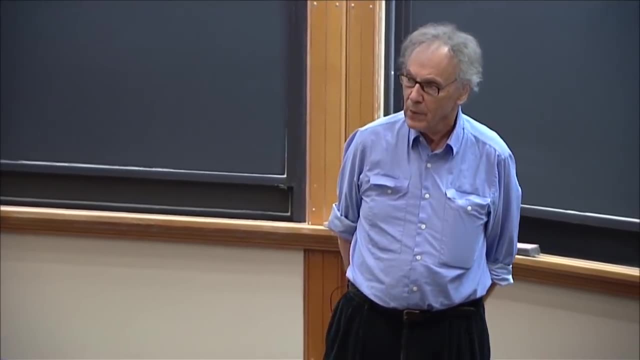 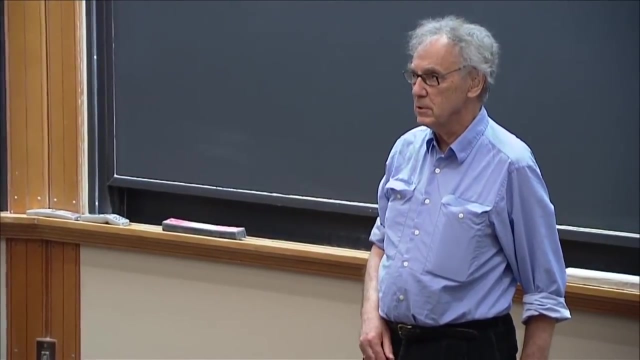 why the electrons do not spiral in is that only discrete energy levels of these electrons are allowed in the atom, And they cannot have energies in between. They can jump from one energy level to another, but they cannot be in between. So there's no way they can spiral down into the nucleus, because then they would slowly. 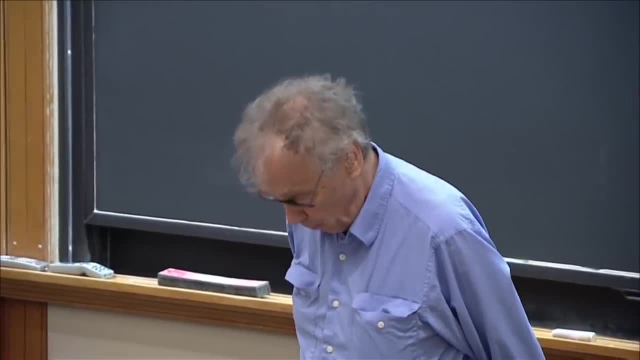 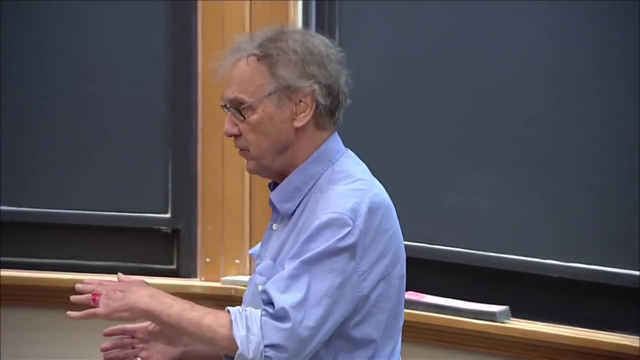 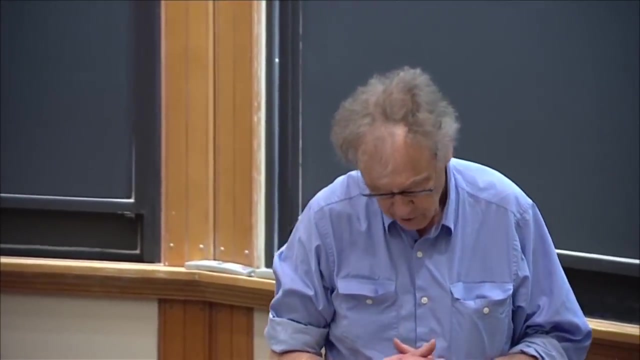 lose their energy, And that is not possible, or at least that was Niels Bohr's idea, And so he introduced the idea of the quantization of energy, Specific energy levels, and they are quantized, And in between electrons cannot exist. 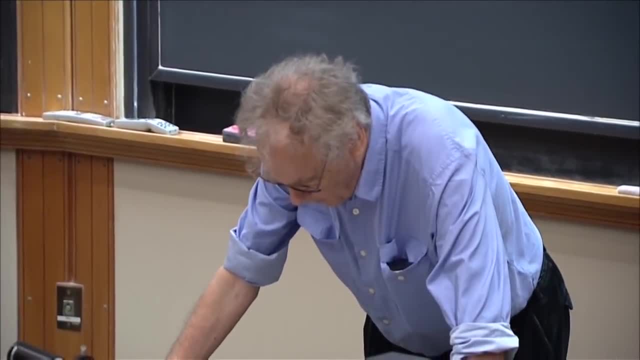 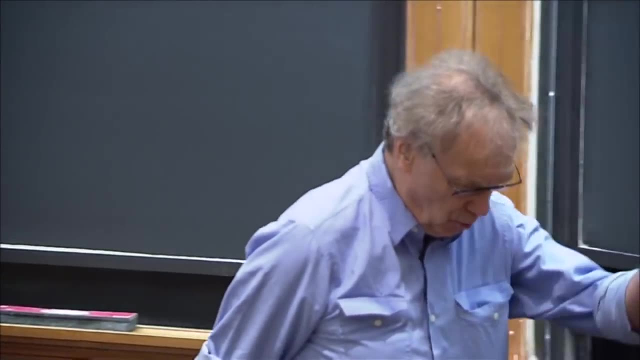 Now, Bohr's suggestion was earth-shaking And it would also imply then, when you come to think of it, that if you had a tennis ball and you would bounce the tennis ball off the floor, that it would not be possible in principle. 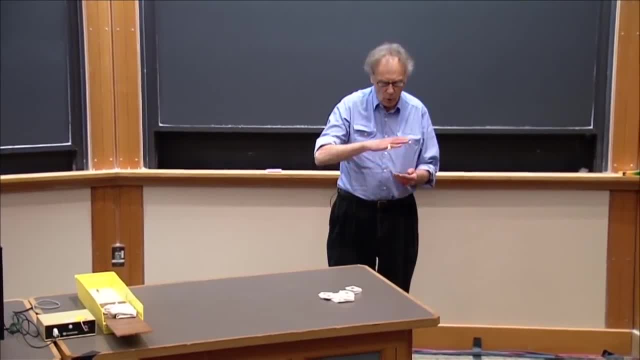 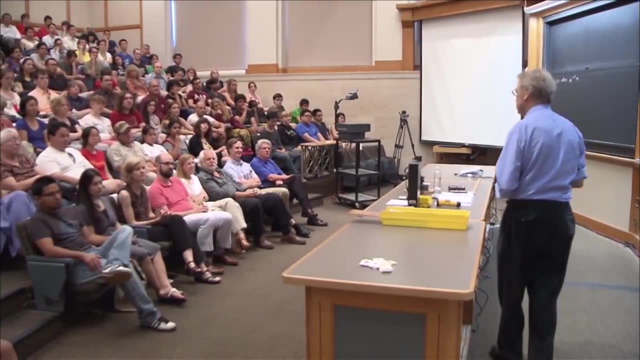 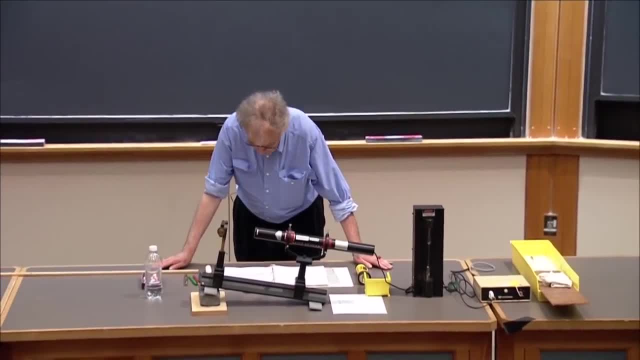 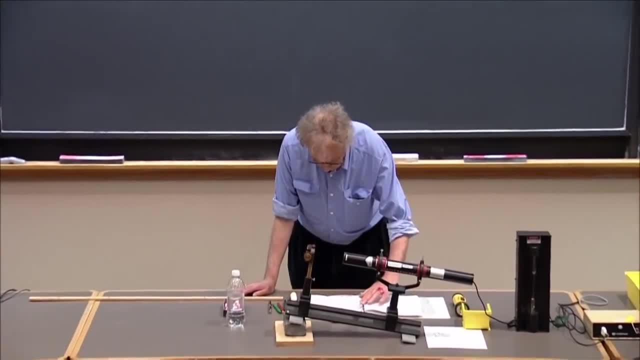 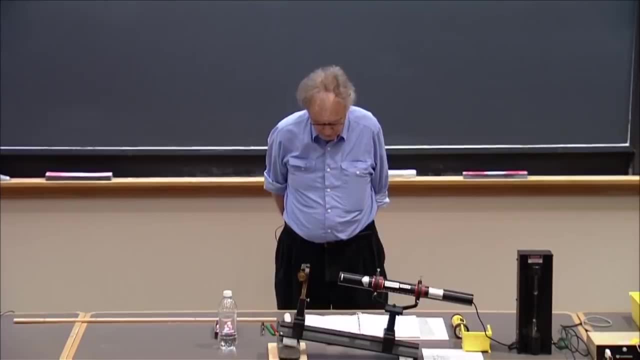 We know that tennis balls do not have these discrete levels. Now, before you dismiss the idea of quantization of allowed levels of tennis balls, keep in mind that the difference between these allowed levels, energy levels of tennis balls, that's not a big difference. 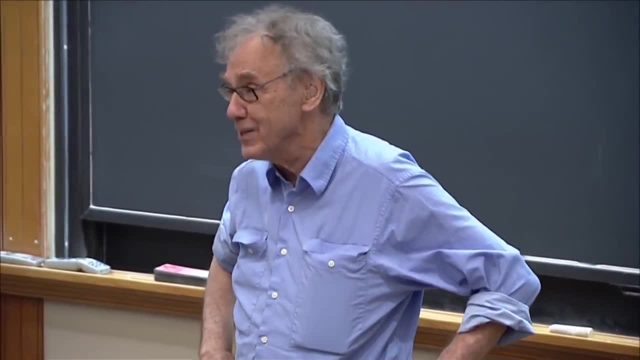 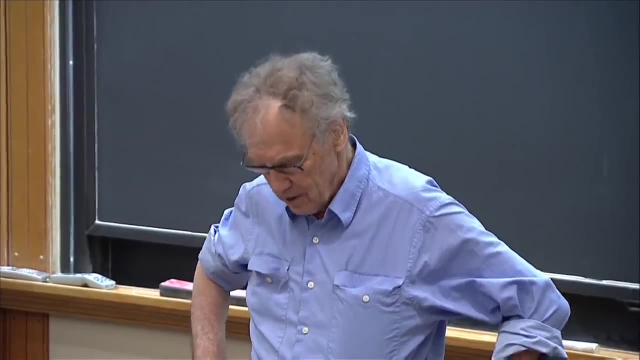 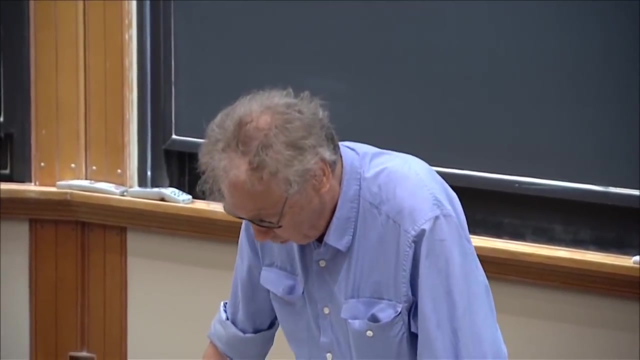 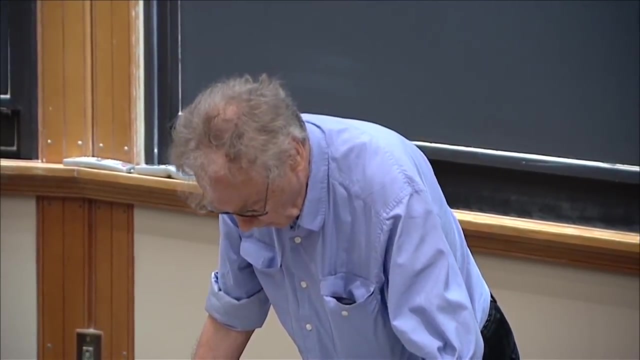 Right, are so ridiculously small that no one could ever measure them, so it's meaningless. So what it comes down to is quantum mechanics has no place in our macroscopic world of tennis balls, but it's all important in the world of atoms and electrons. 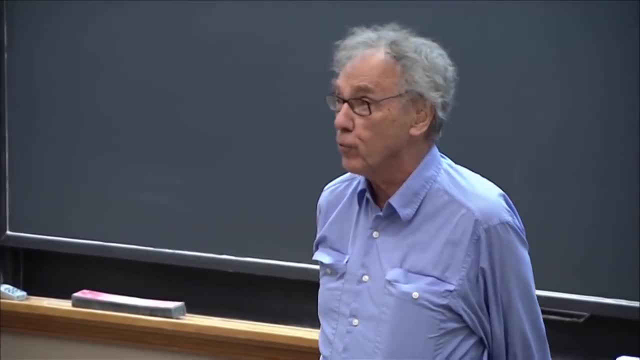 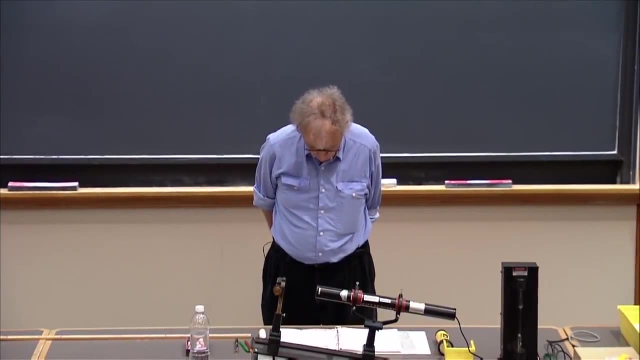 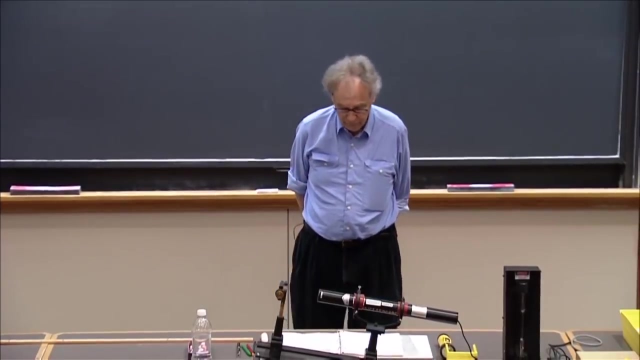 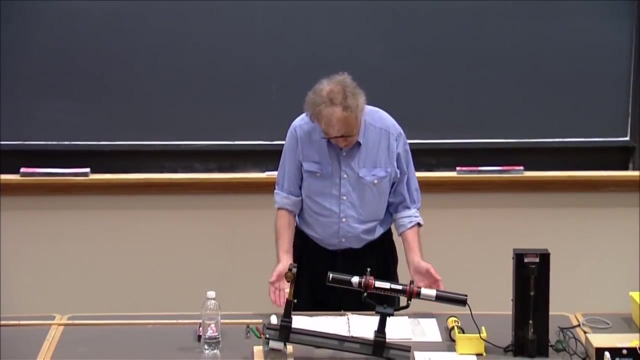 So, before we continue, let me repeat, then, the cornerstone of quantum mechanics by Niels Bohr: The electrons in atoms can only exist at well-defined energy levels. They cannot exist between these levels. Therefore, the energy levels are quantized. The lowest energy level could be E1, and one level up could be E2.. 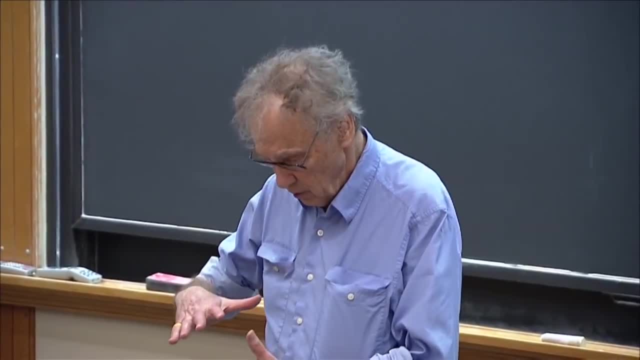 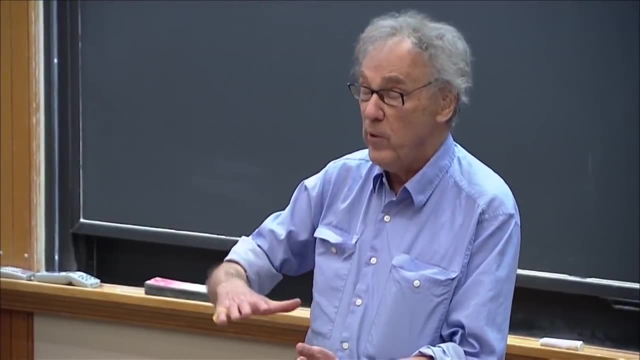 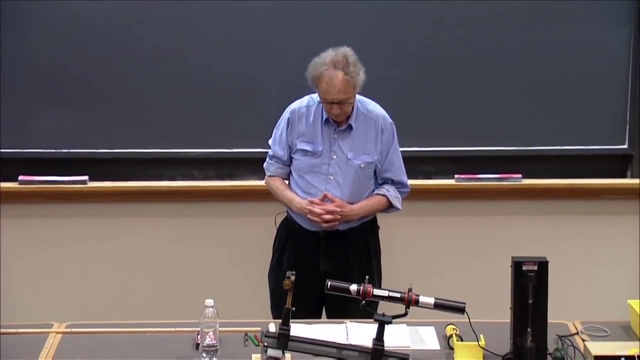 And when I heat. When I heat a substance, electrons could jump or move if you want it from, for instance, E1 to E2, or they go from E1, they could go to E3. But always quantized steps. 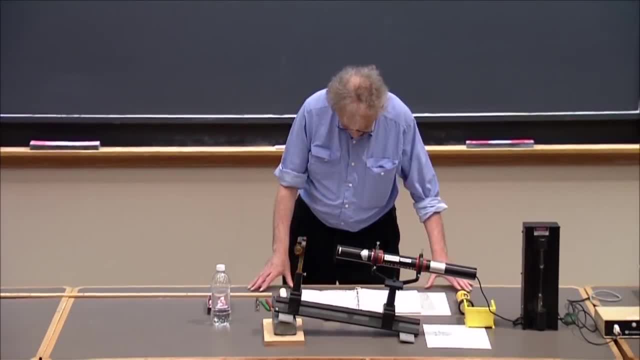 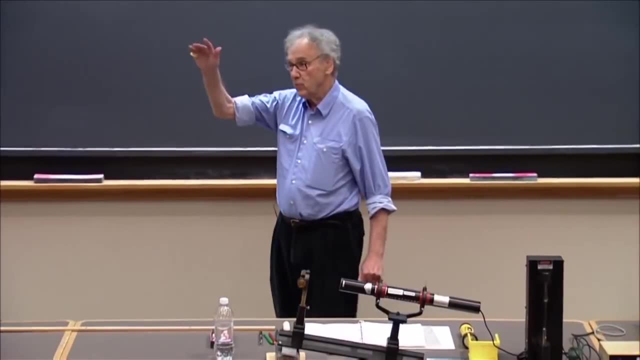 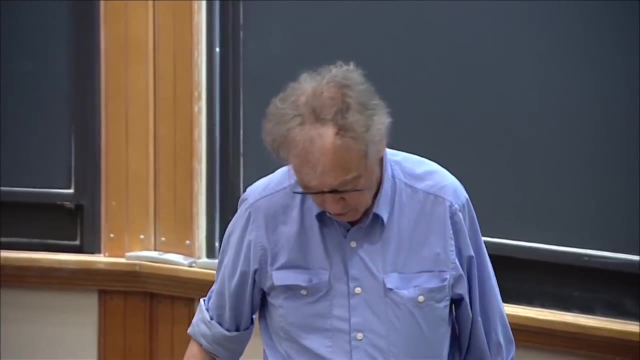 So an electron that jumps to a higher energy state will spend there some time and then it will cascade. It will take down to the lower energy state where it came from, And this cascading down it can do in many different ways, which I will shortly show. 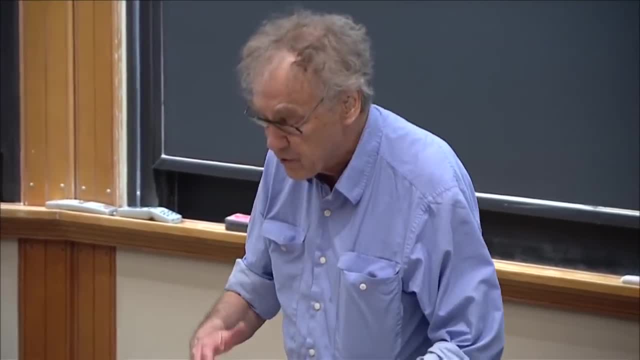 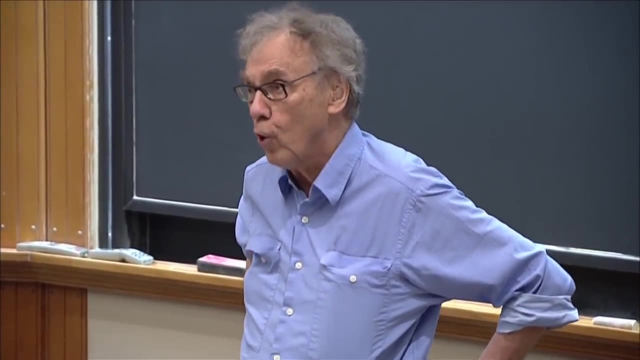 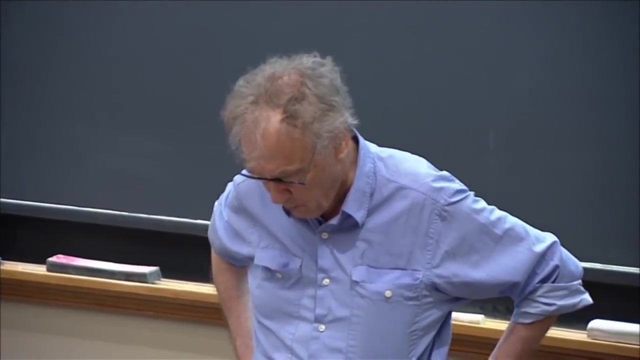 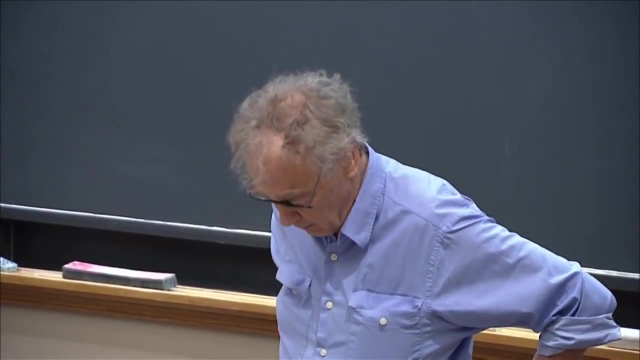 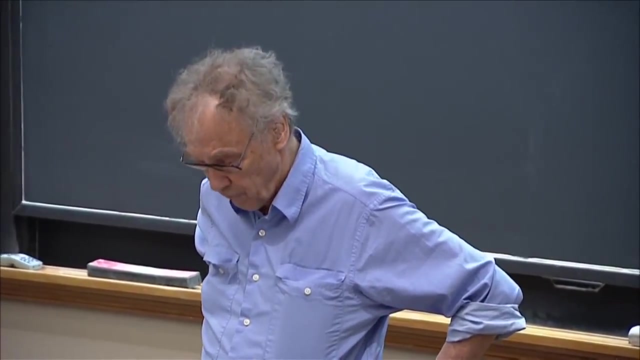 you. These discrete energy levels are often represented in high school and college books as circular orbits. They compare the electrons going around the nucleus with planets going around the sun in well-defined orbits. That is a misconception. It is virtually impossible to envision the very complicated trajectories of electrons. 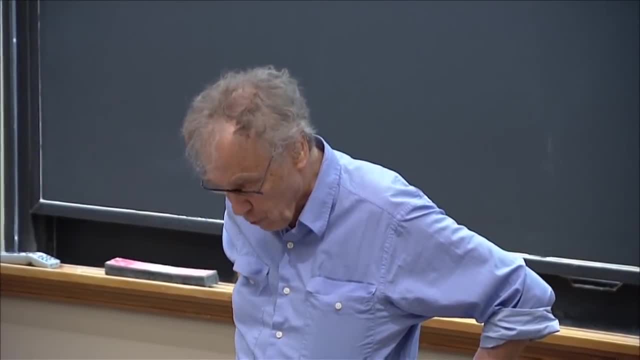 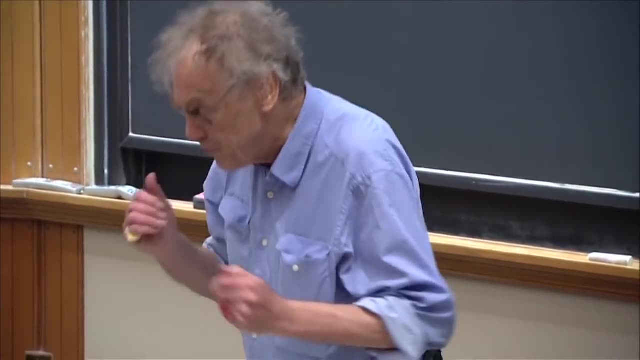 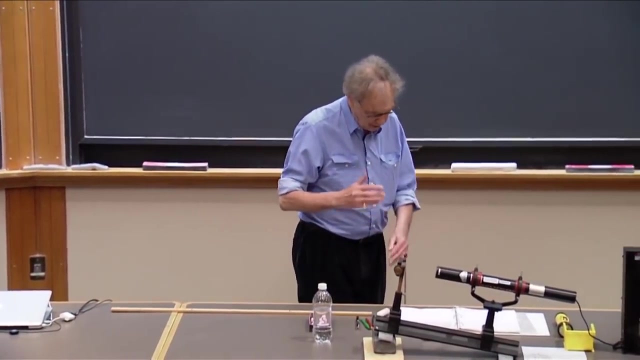 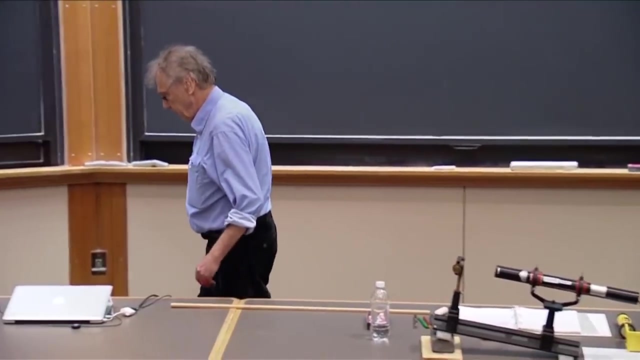 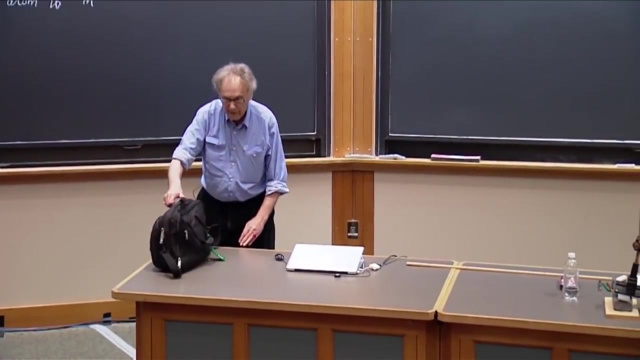 around the nucleus? For sure they are not orbits, But this is not important for me. I don't want to talk about trajectories of the electrons. I want to talk about the energy levels, the quantization of the energy levels. I have here a bag and in that bag is a laptop and I can put it up here and when I do that, 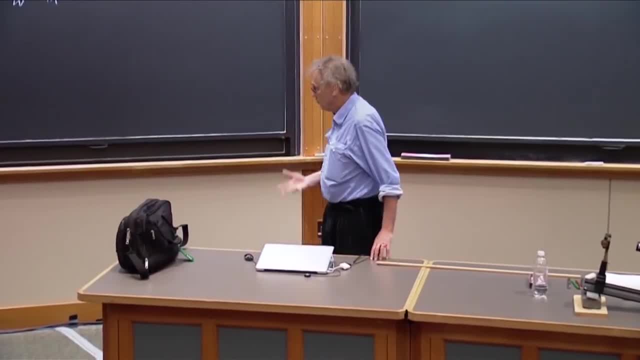 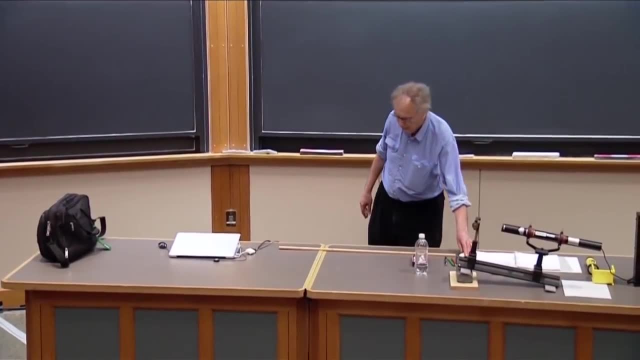 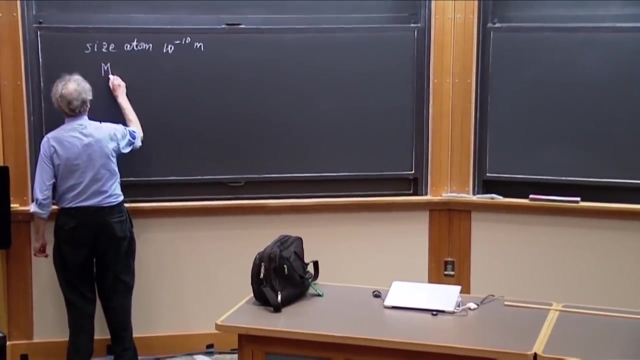 I have to do work. I have to put energy in. We have discussed that several times. The energy that we have to put in is what we call gravitational potential energy. You may remember this from one of my first lectures here. That energy that you have to put in is mgh. 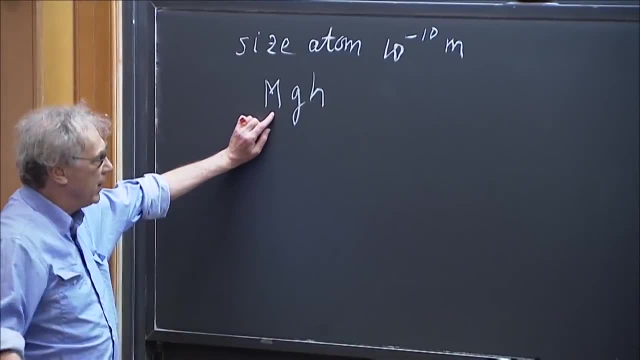 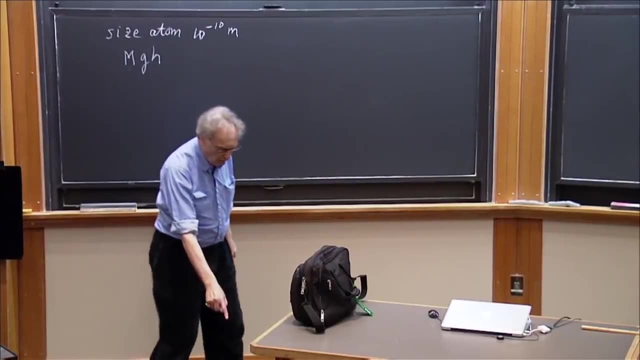 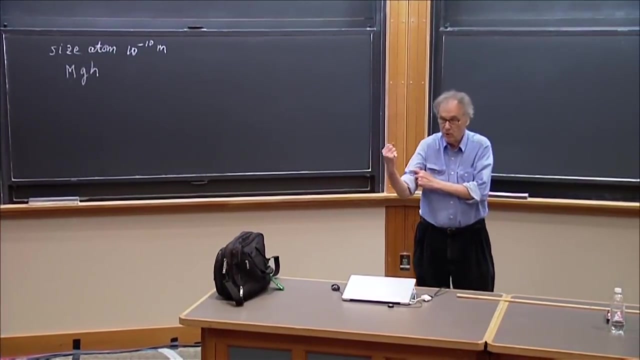 m would be the mass of the bag in kilograms, g is the famous 9.8, and h would be the height in meters from the floor to here. Now that energy that I've put in there with my muscles is not lost When I do this. 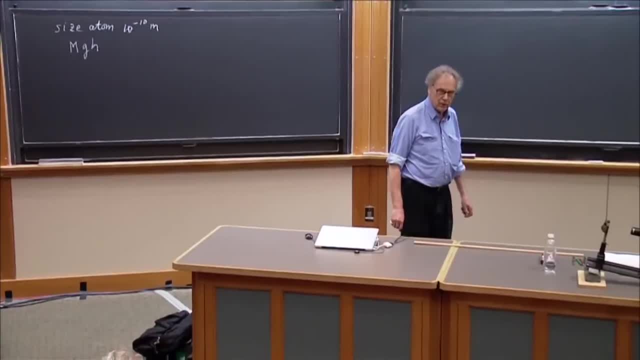 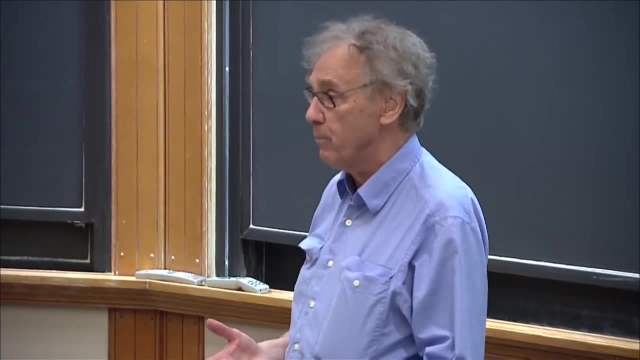 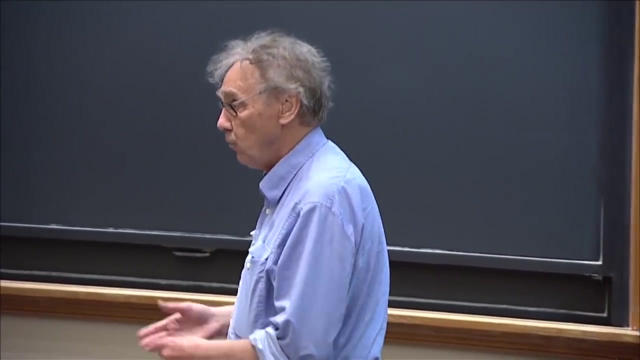 It converts back to kinetic energy, It picks up speed and then the kinetic energy at the floor disappears. For one thing, it probably broke my laptop, which takes energy. There is some friction with the floor, which produces heat. There was some sound, which is also energy. 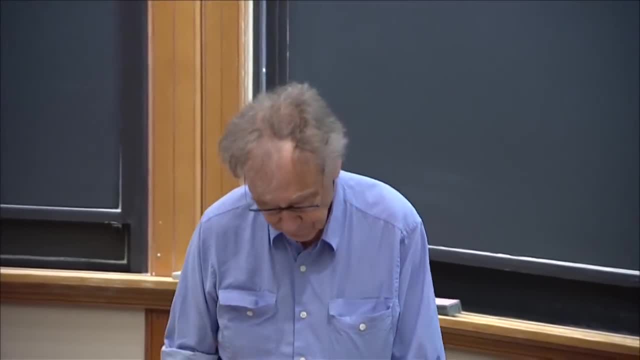 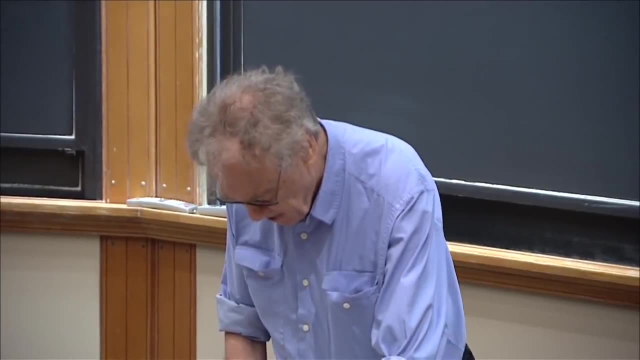 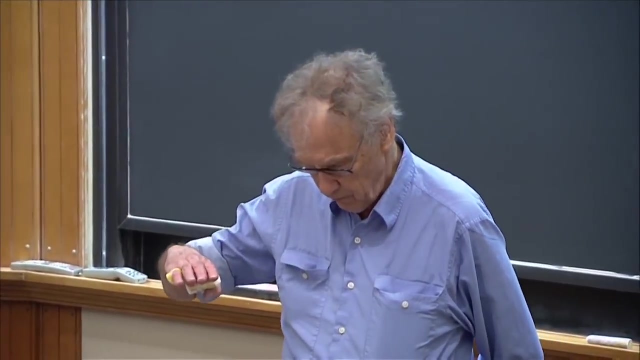 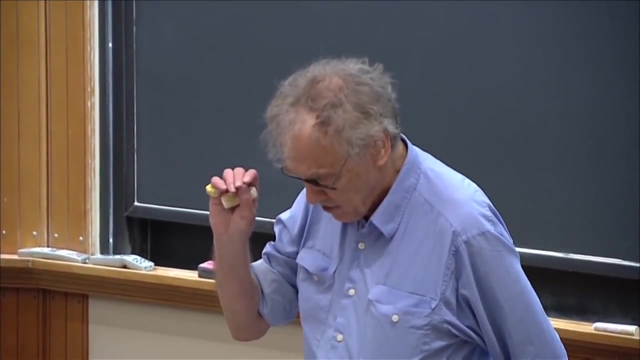 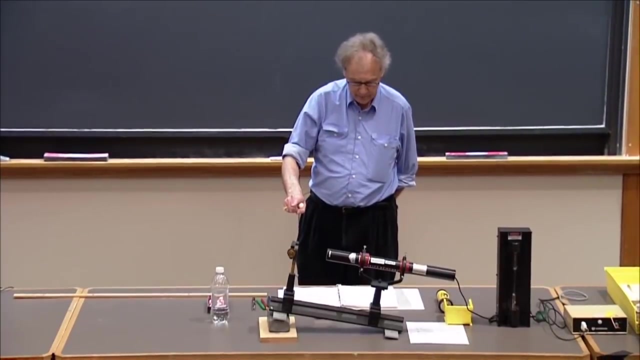 So energy is conserved. In a similar way the energy that was needed to bring an electron from a lower energy state to a higher energy state. in a similar way that energy is not lost When the electron moves back to a lower energy state. the atom emits the energy, not in the 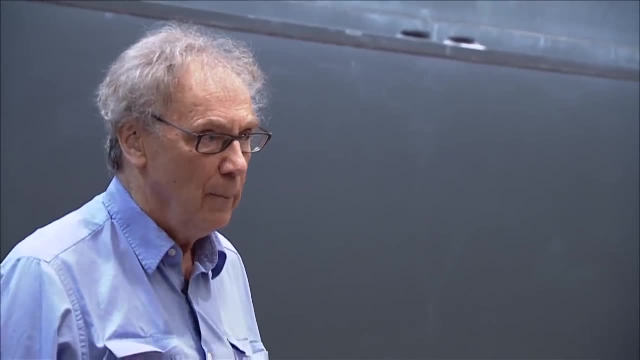 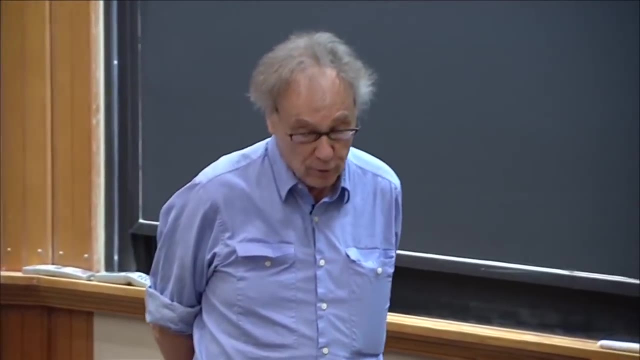 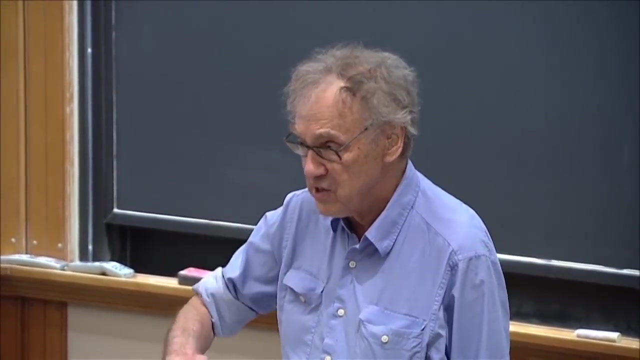 form of kinetic energy, But it does that largely in the form of electromagnetic radiation. could be x-rays, could be ultraviolet light, could be visible light, could be infrared, could be radio waves, But the energy that is necessary to bring an electron up when that electron jumps back. 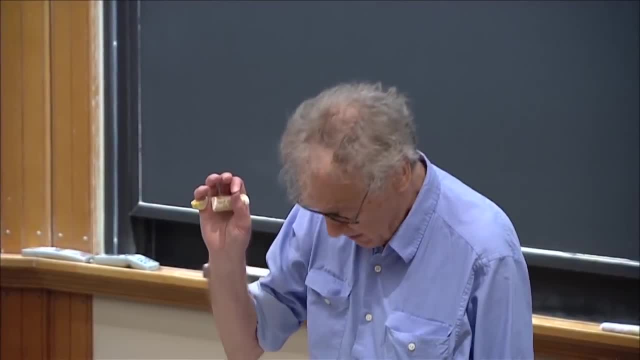 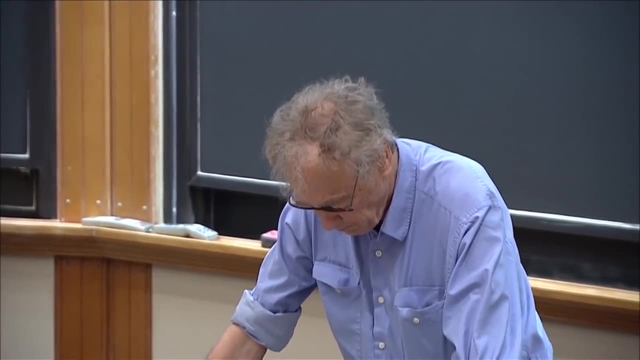 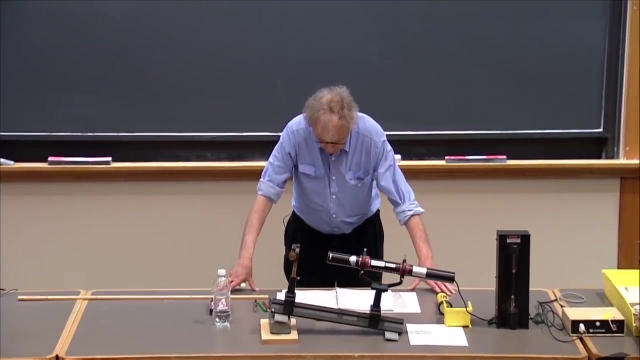 to where it came from. the same amount of energy is again released, of course, because that's the conservation of energy. In physics, it is the conservation of energy. Light has energy. It was Einstein who showed that the various colors of light each represent a different. 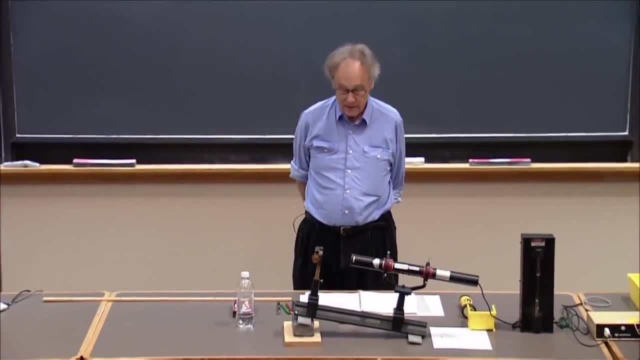 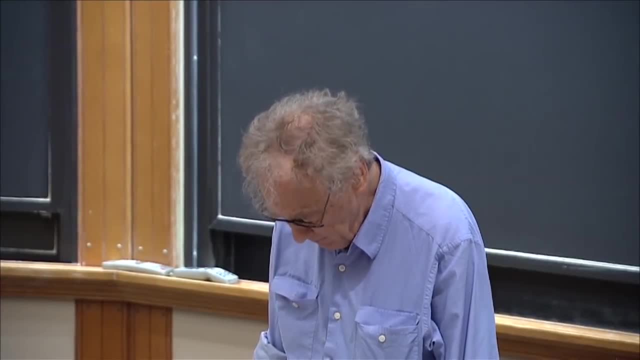 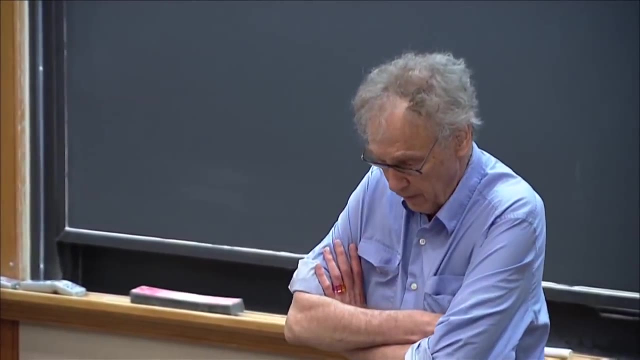 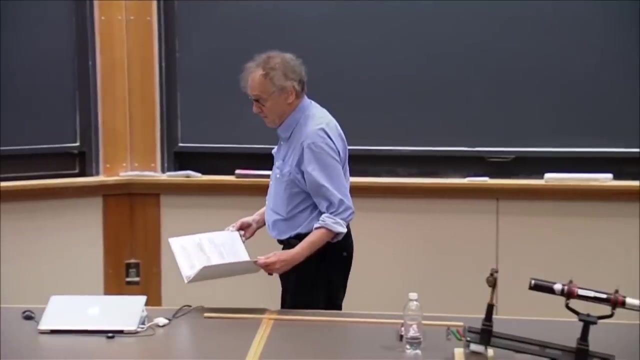 but well-defined amount of energy, and that's when the name photons was introduced. Light is a form of electromagnetic waves. When we have waves Right have a frequency, as you have seen with sound, and then you have a wavelength, And I will choose, more or less at random, the color green because that's in the middle. 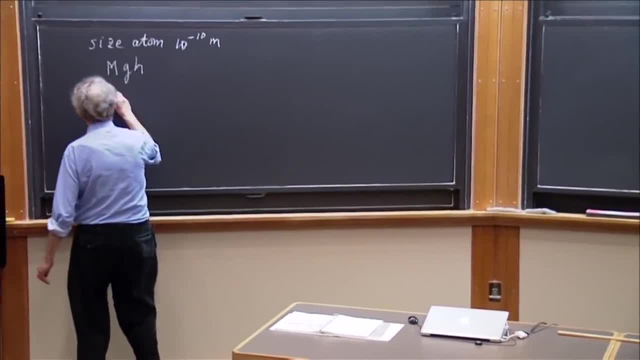 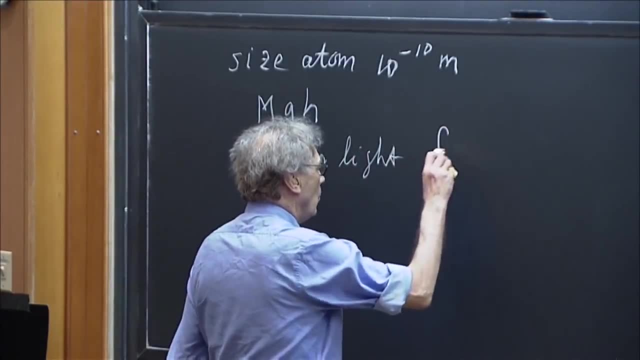 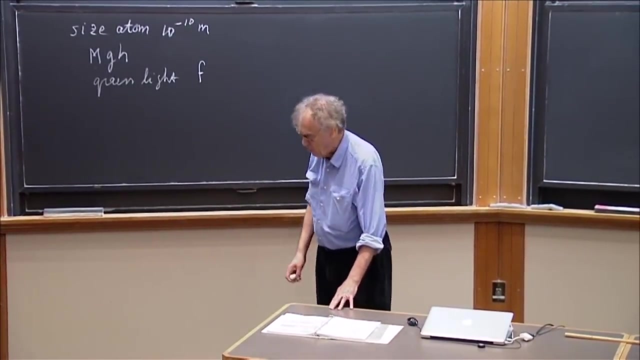 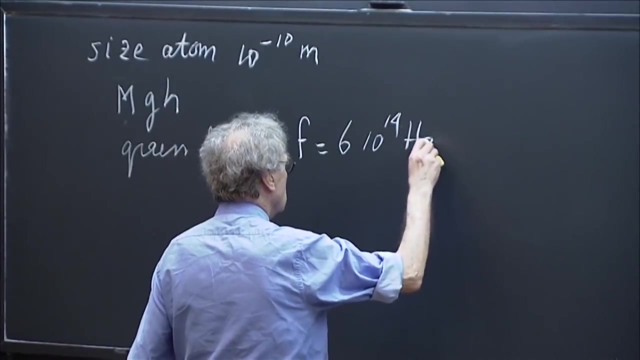 of the spectrum. So what I'm going to tell you now holds for green light. The frequency of the electromagnetic radiation of green light is about six times ten to the fourteen hertz. Six times ten to the fourteen hertz. Remember, with sound we were talking about hundred hertz, thousands of hertz. here we're. 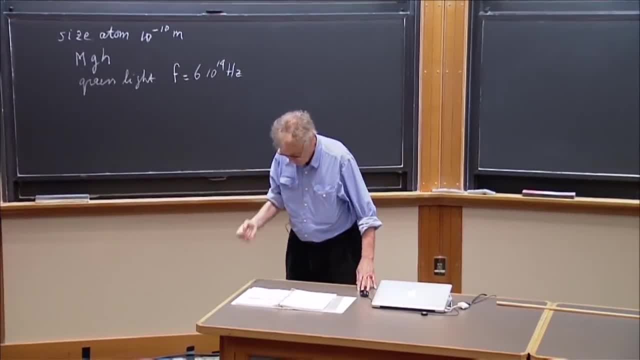 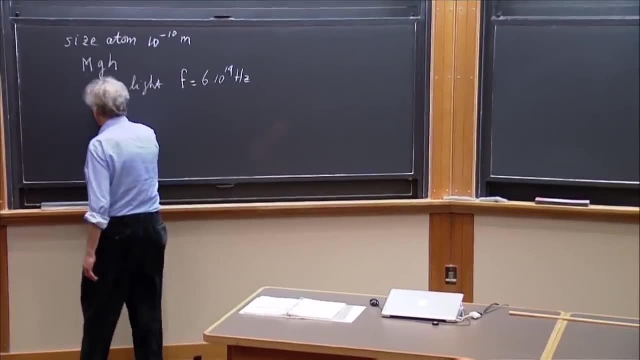 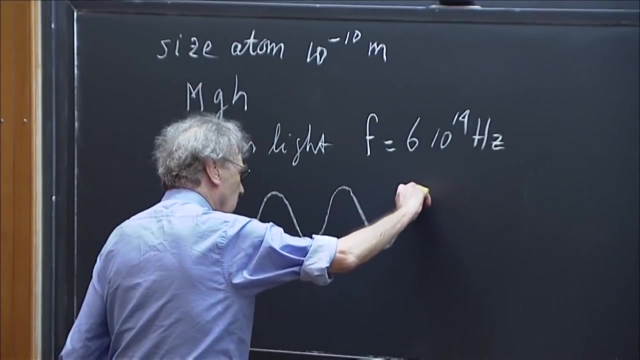 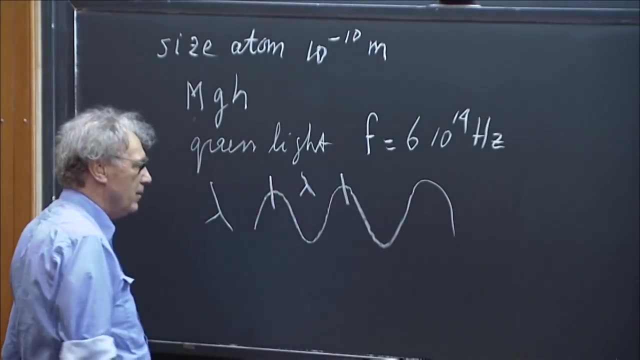 talking about ten to the fourteen hertz, The wavelengths for which we normally write the symbol lambda, and the wavelength is as follows defined: If this is the wave, as you have seen last week In strings, then the separation from here to here is what we call the wavelength lambda. 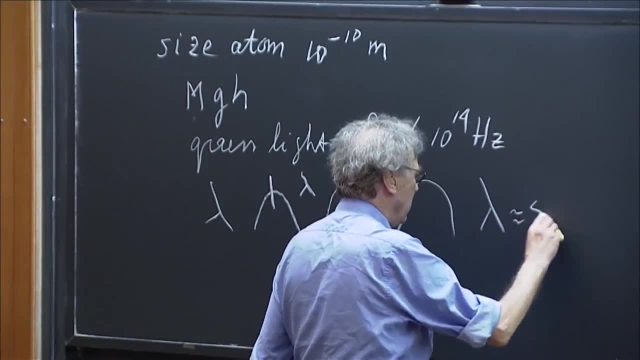 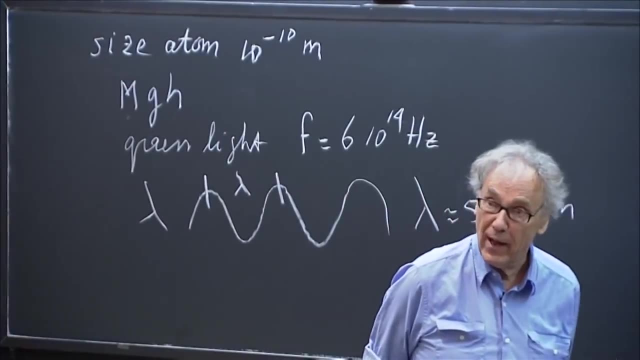 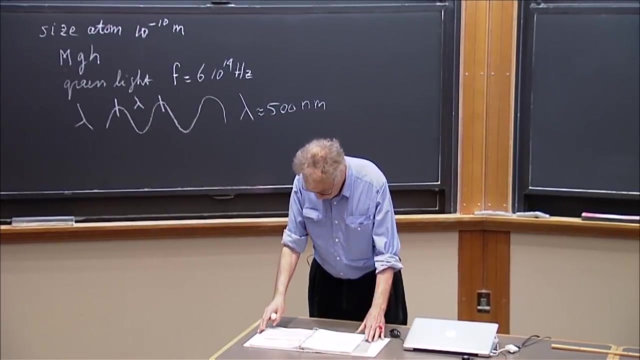 The wavelength lambda for green light is approximately five hundred nanometers A nanometer. a nanometer is ten to the minus nine is one billionth of a meter. It's also half a micron, if you like that, If you. 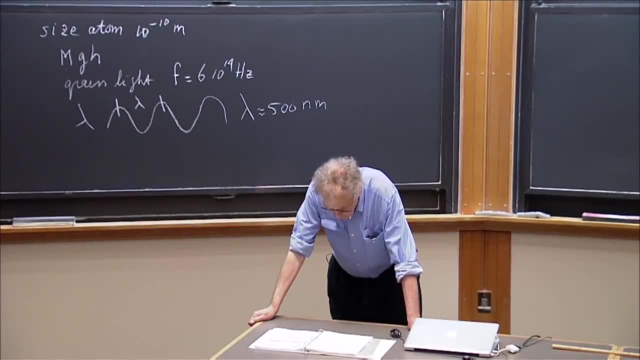 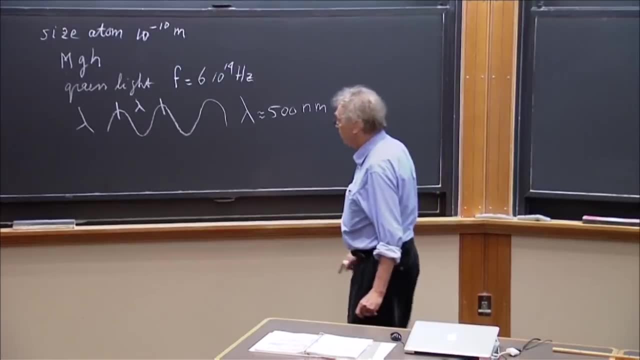 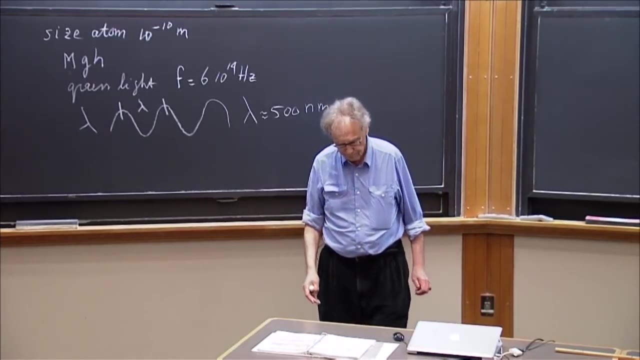 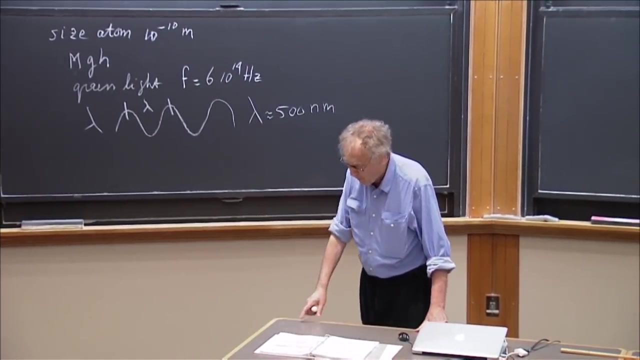 take red light, then the frequency is lower and the wavelength is longer. And if you take blue light, then the frequency is higher and the wavelength is shorter. Einstein showed that the energy of a photon E and a neon 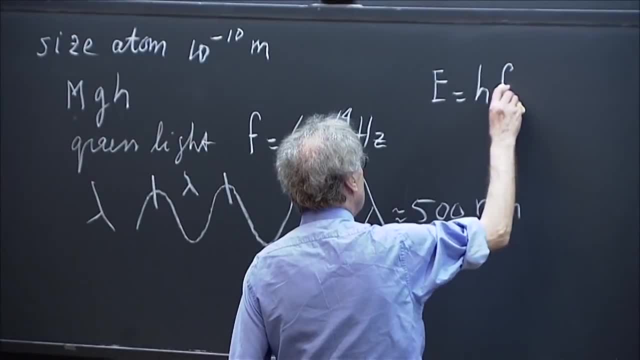 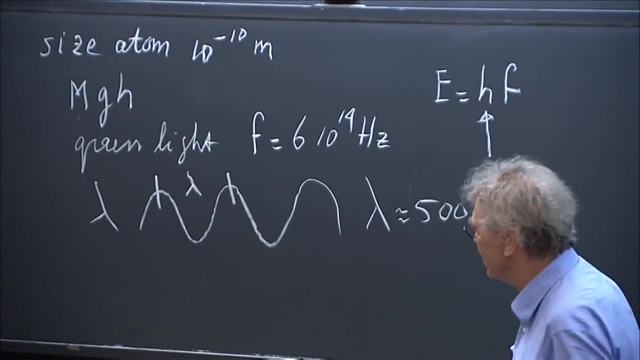 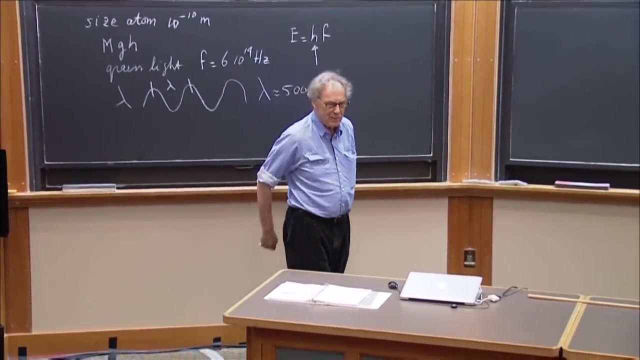 equals HF and that H is what this lecture is going to be all about. That H is not this H. this H is in meters. that H is Planck's constant, which is at the heart of all quantum mechanical calculations. 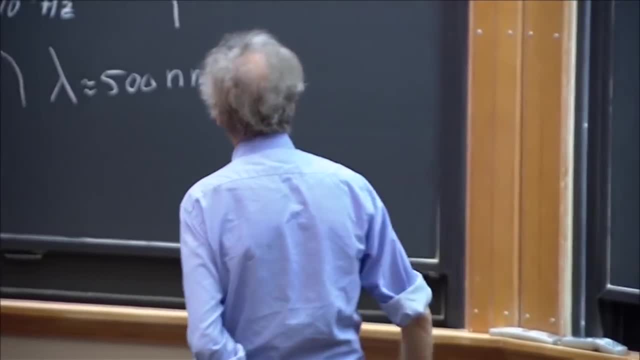 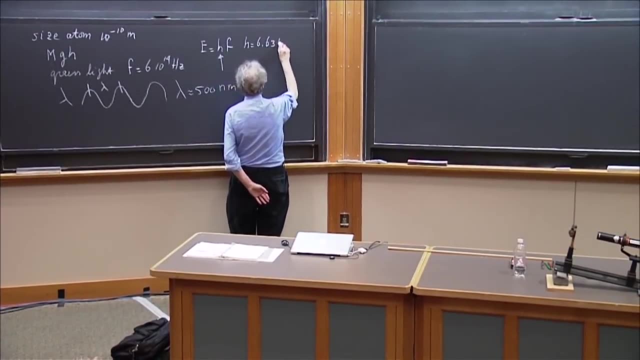 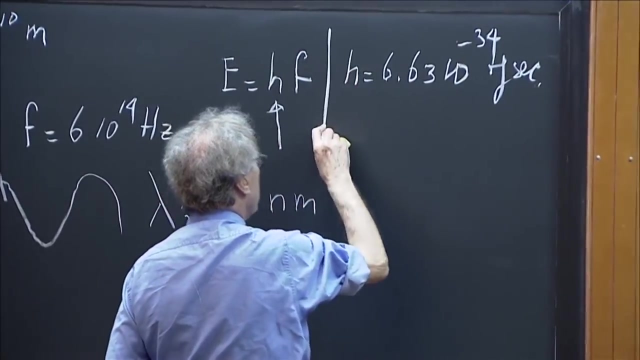 reason and H. I will give you what it is. it is 6.63 times 10 to the minus 34 joule seconds, And we're going to see it again and again, and again today. So now that you know, 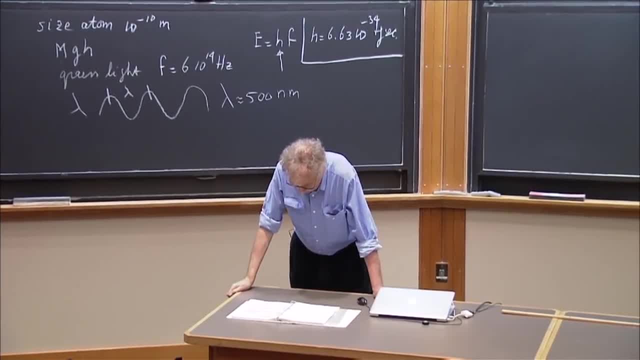 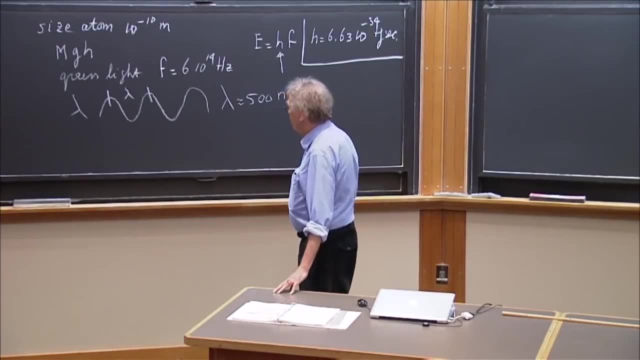 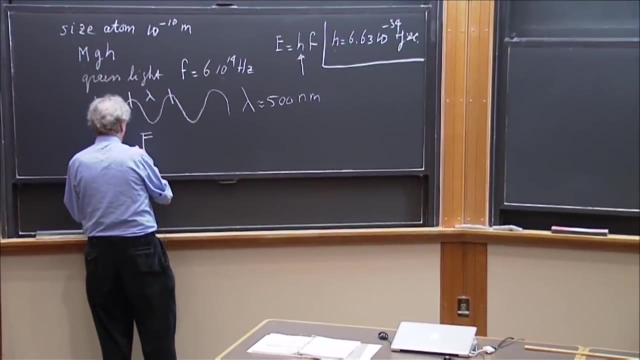 that the energy of an of light is H times F. you can calculate for green light now what the energy is, Because you take H and you multiply it by this frequency, and so then the energy of green light- I have to check that that I have the number right- is 3.6. 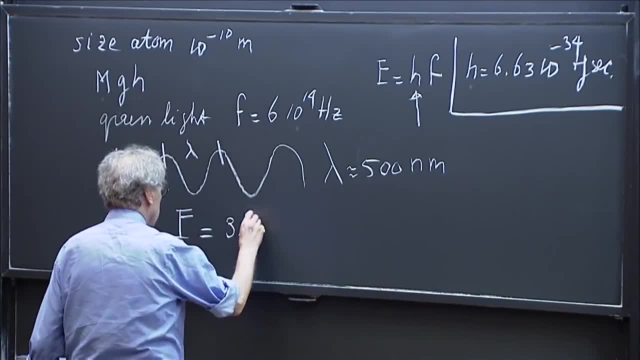 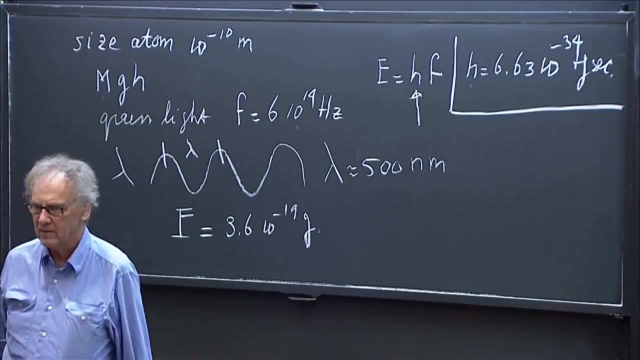 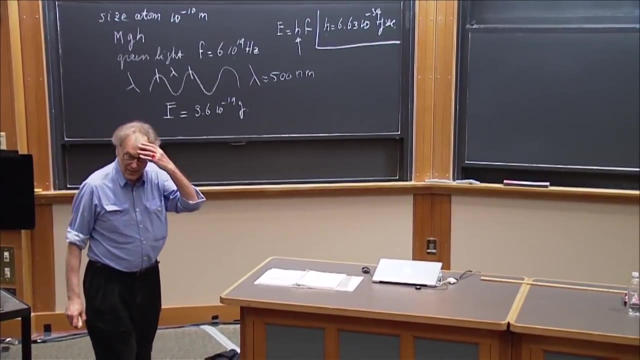 times 10 to the minus 19 joules. 3.6 times 10 to the minus 19 joules. No physicist would ever say that It's correct. I cannot even imagine what the energy of green light is, What 3.6 times 10 to the minus 19 joules is. I cannot. I have no idea what it is. Therefore, 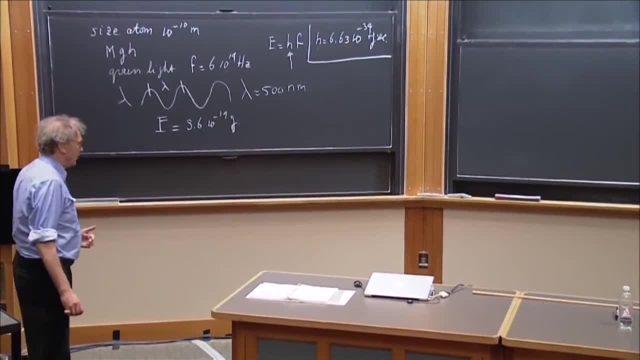 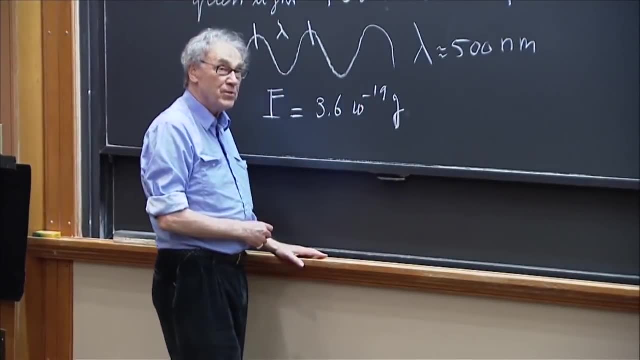 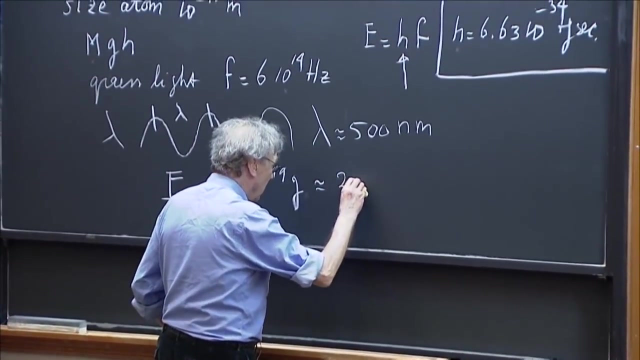 we have introduced a different energy scale, which almost all physicists use, which is which takes care of these ridiculously low numbers for which you have no feeling, and that is an energy in terms of electron volts, and this, then, is roughly two electron volts. 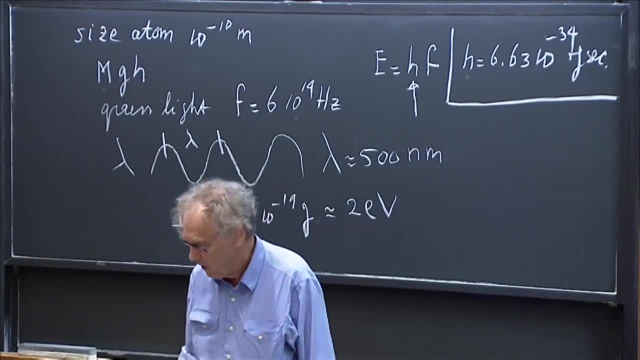 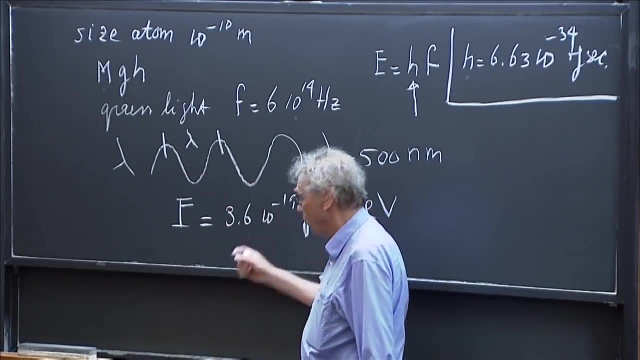 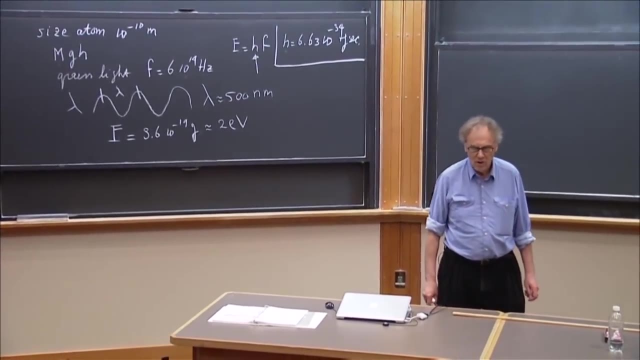 And that's much easier to think in terms of electron volts. If you're neither used to think in electron volts and you're neither thought used to think in terms of 10 to the minus 19 joules, then simply remember that the amount of energy of one green photon is 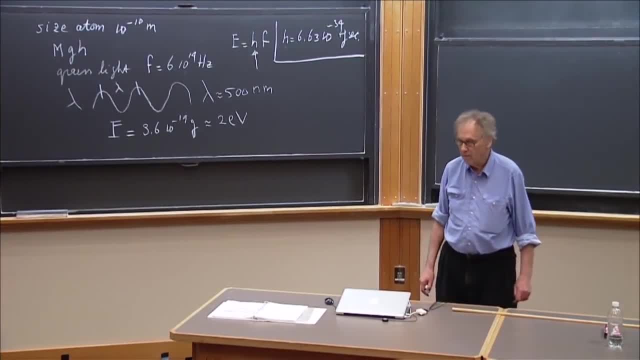 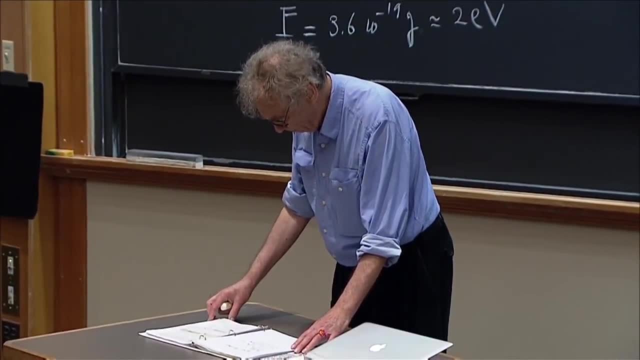 very, very, very low, And that's all I hope I have achieved now. As I mentioned, I hope you have enjoyed this lecture. If you have any questions, please let me know. If there are any questions, please feel free to email me And I'll be happy. 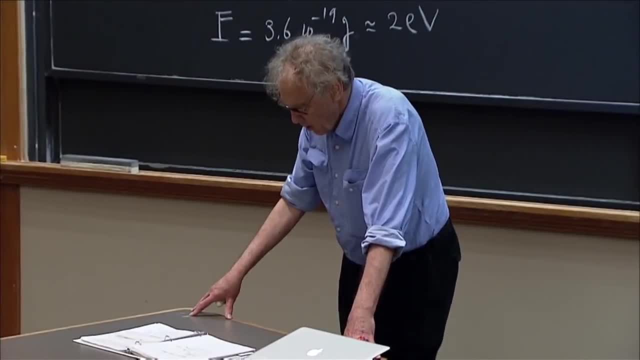 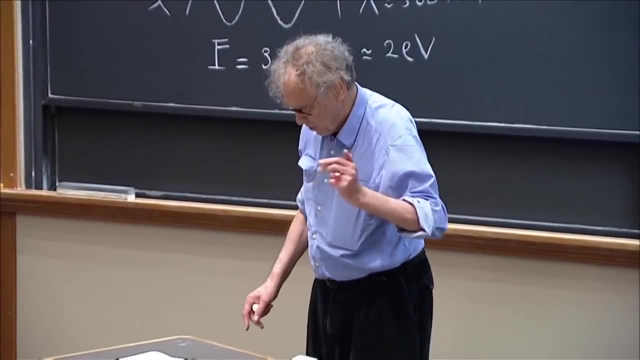 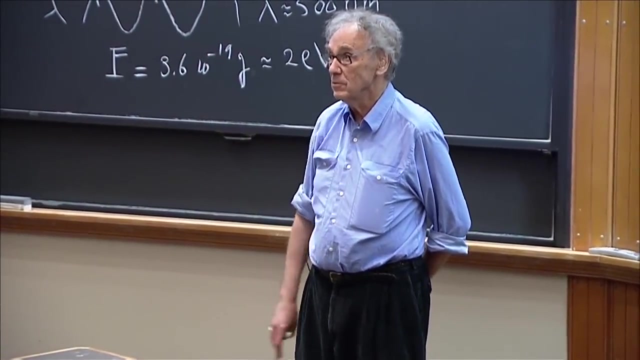 to answer any questions you might have about this lecture. Thank you. It's very important to remember that the amount of energy that is released when an electron changes from a higher energy state to a lower one is exactly the difference between these energy states, And so as the electron cascades down, as you will see how that works. 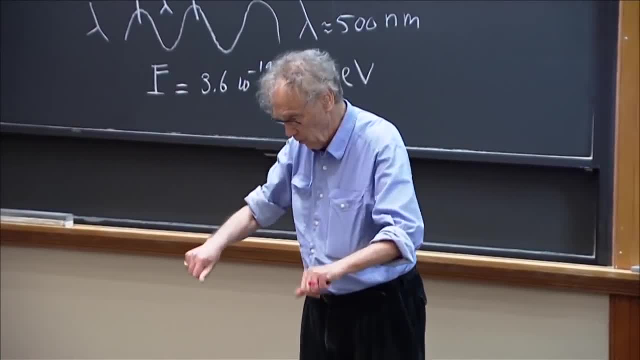 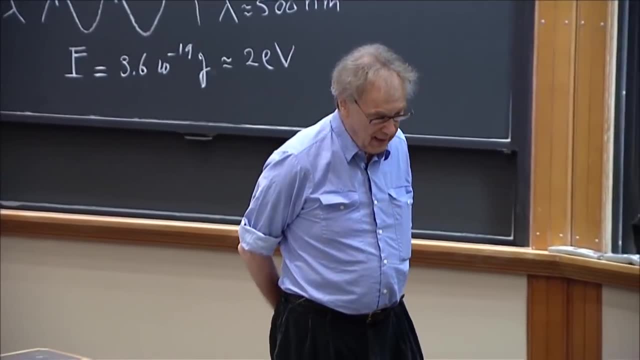 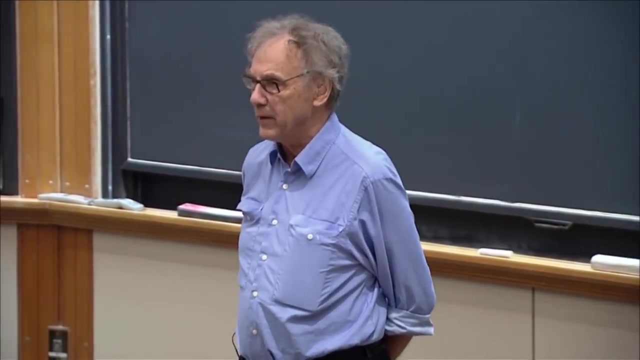 all the energy that was necessary to get it up will return. So if we now measure a single, the energy or the color or the wavelength of the photons that are emitted by an atom when an electron from a high energy state cascades down to the lower energy state, 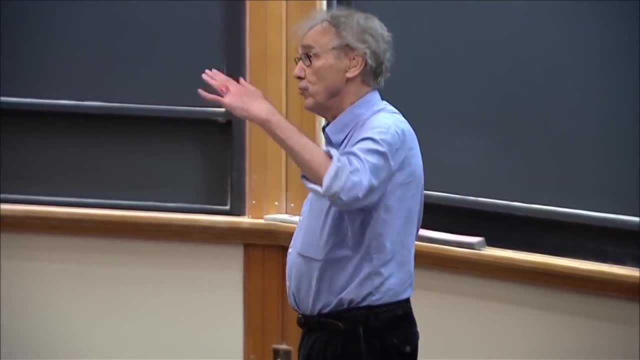 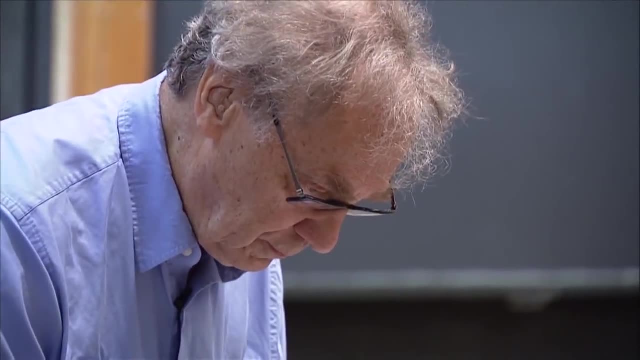 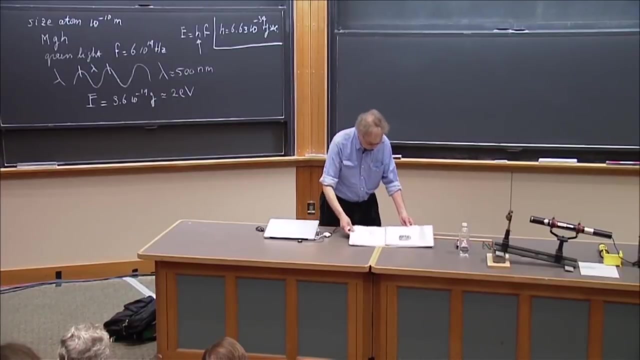 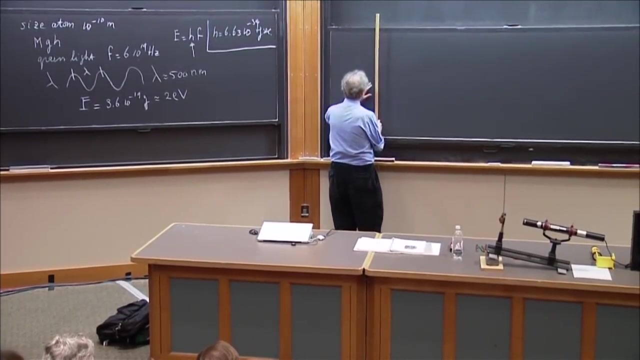 If we measure those, then we know where these energy levels are, And that's the way that it is done. Now I will make you an energy scale of electrons, arbitrarily chosen. I've not selected any particular values. I'm going to have a low energy level here, here, here and here. 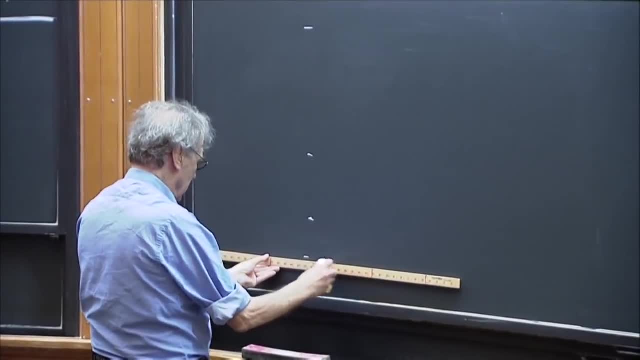 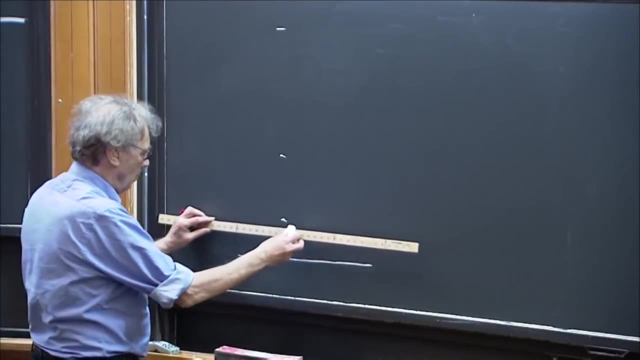 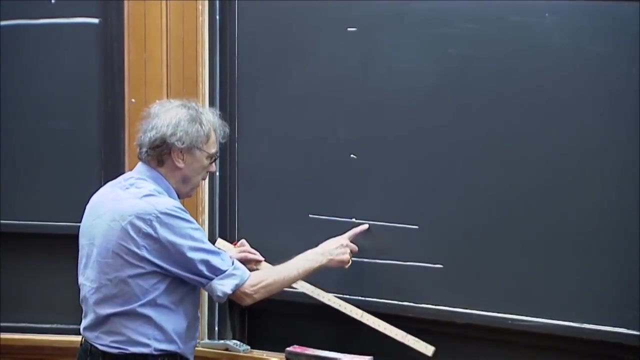 In other words, this energy level would be the lowest energy level that an electron could have in a particular atom, And this would be then the next level where it could be. It could not be here. It could be here or there. 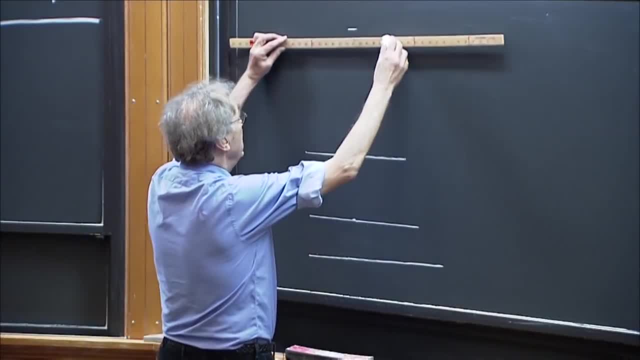 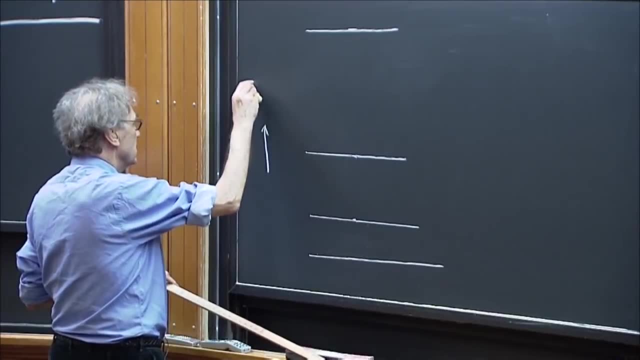 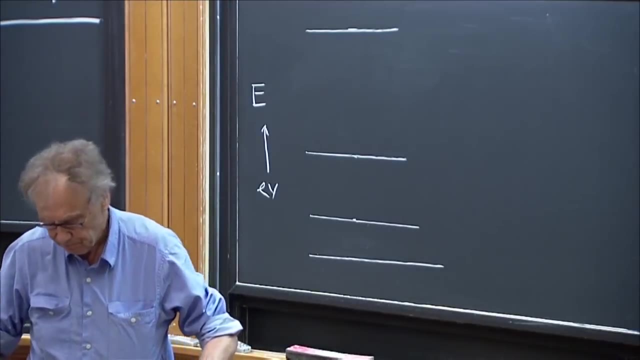 And the electron can be at this energy level. and the electron could be, for instance, at this energy level And this scale is energy, And the units may well be electron volts, some unit of energy. Now, let's assume that there is only an electron here. 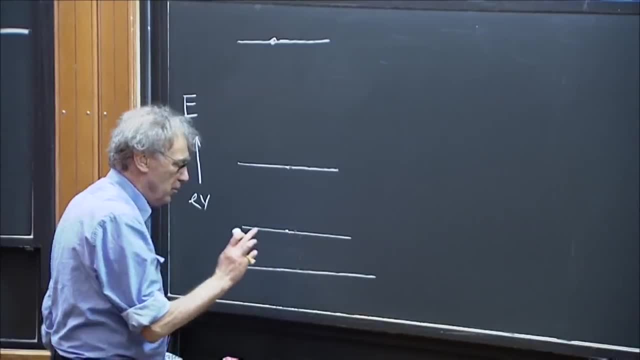 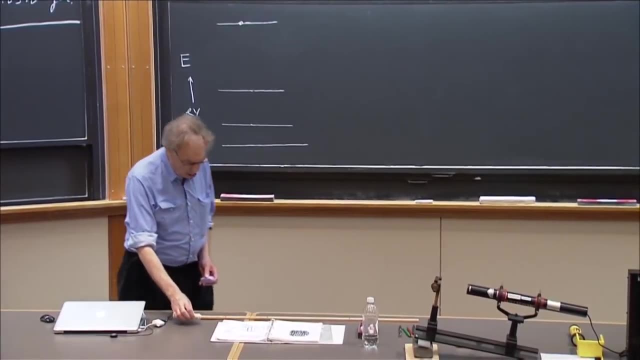 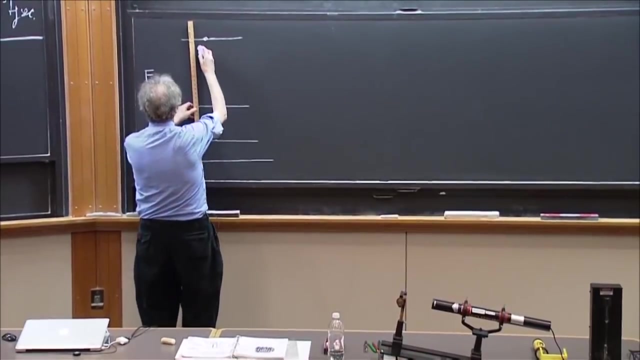 and that these energy levels are not occupied. So just one electron sitting there. This electron will now cascade down to its lowest state, and it has many different ways of doing that. One way that it could do that is the following: It goes in one jump. 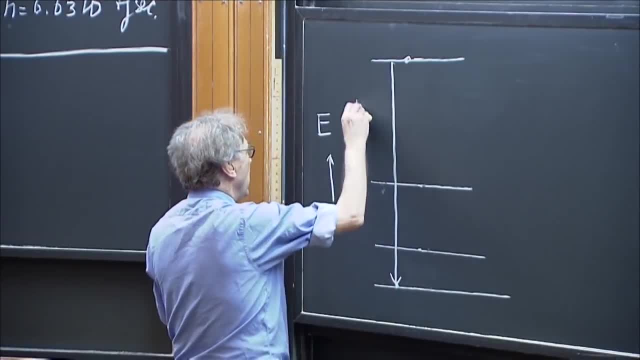 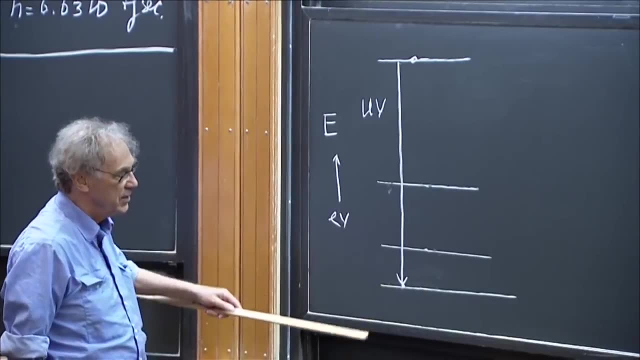 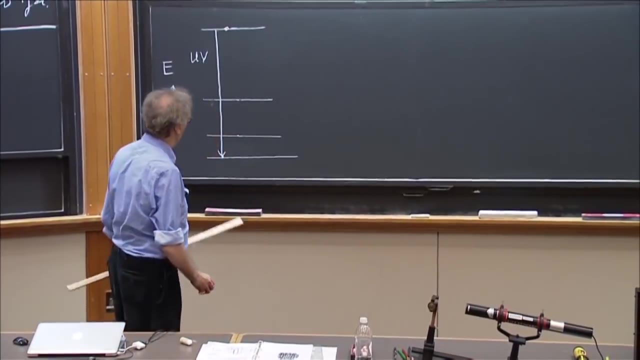 down and the radiation that it emits is so high in energy, because this is a huge distance in energy that we may not be able to see it. It may be ultraviolet, But of course it could also do it this way. 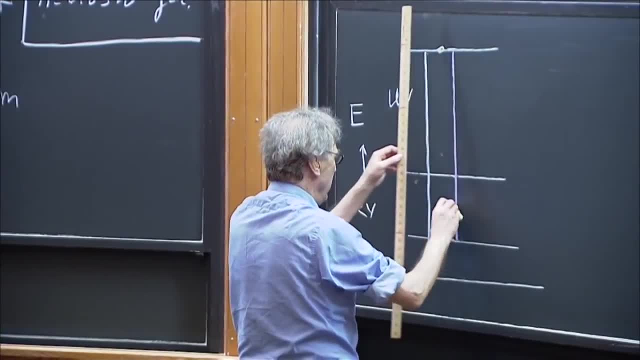 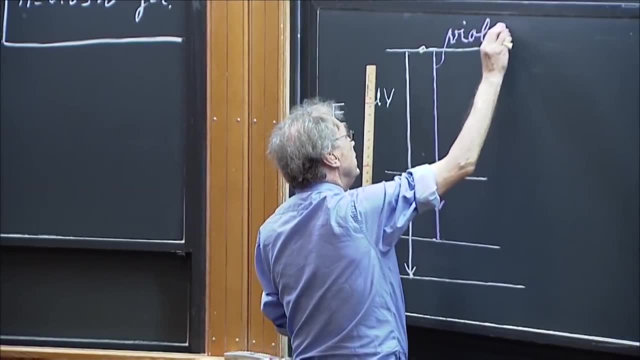 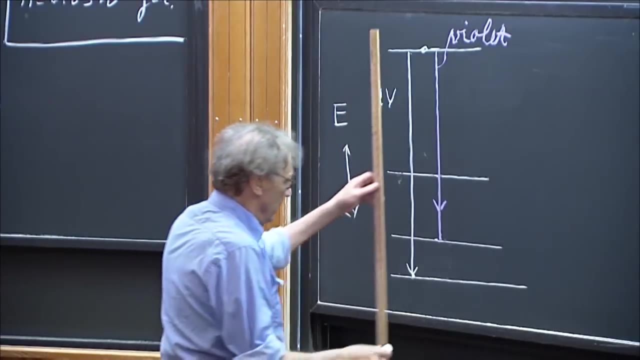 It could go from here to here and emit a violet photon. I will write that here so that people on TV can see that this color is violet. So it comes at this level and then it has to go ultimately down to the ground level. 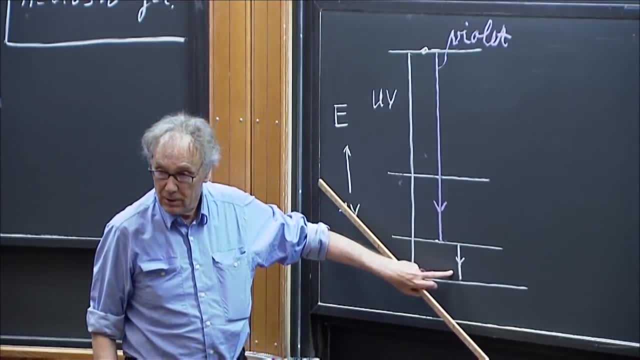 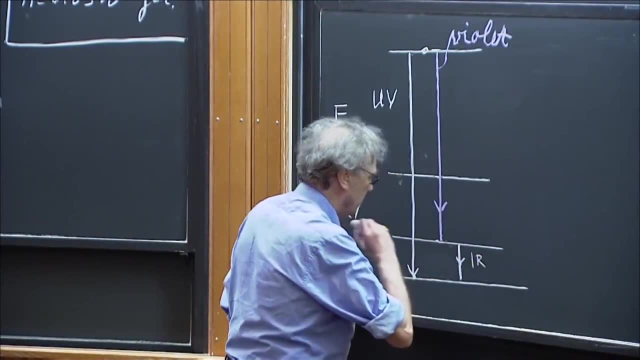 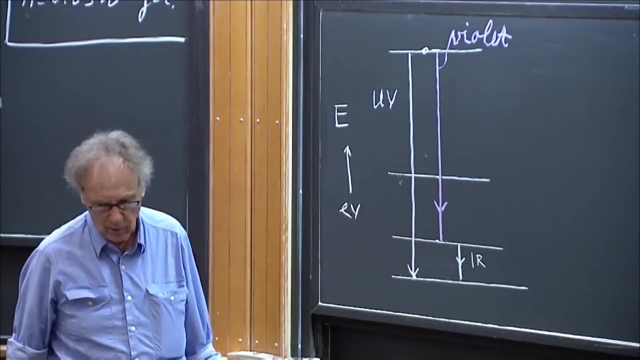 and this energy may be so little that we can't see it. It may be infrared, So let's assume that this is infrared. So it sends out two photons, a violet one and an infrared one. But of course it has more choices. 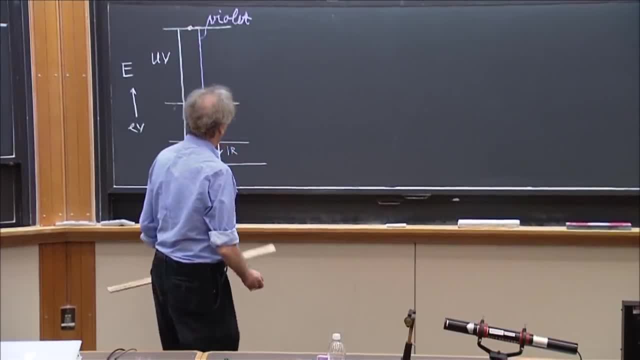 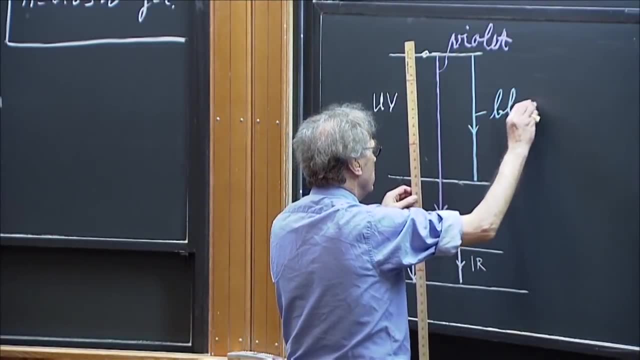 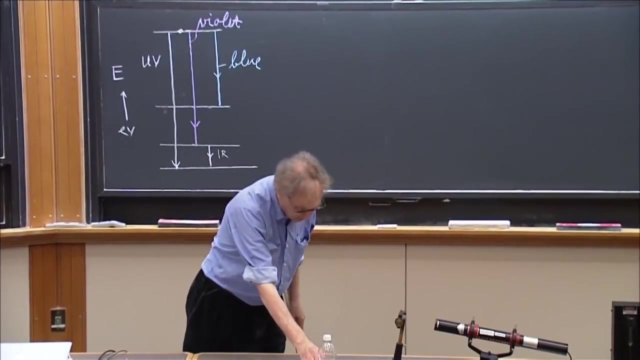 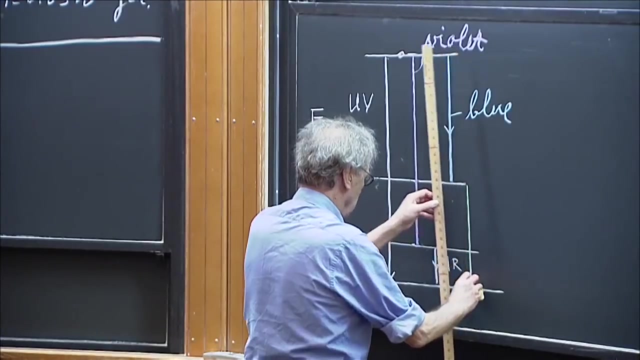 It could do the following: It could go from here to here and send out a blue photon, And then, when it is there, it could, for instance, go straight to the ground level. So it could do this, And this might be green. 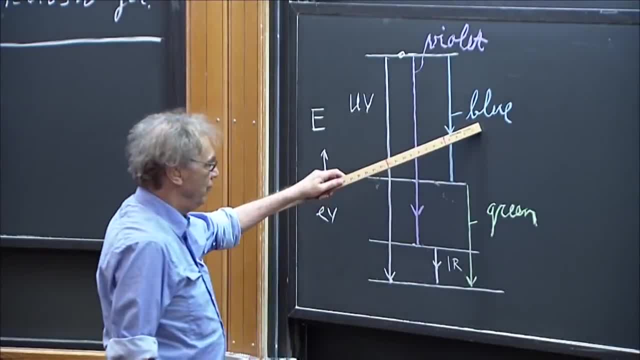 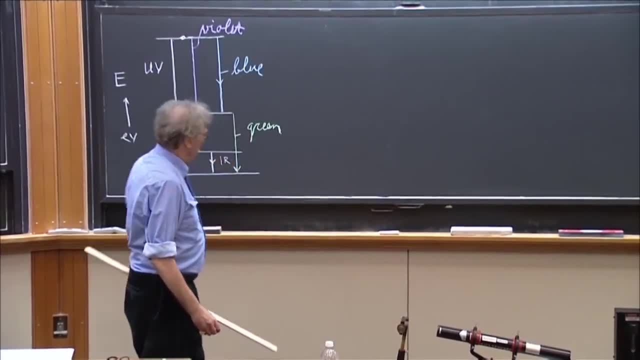 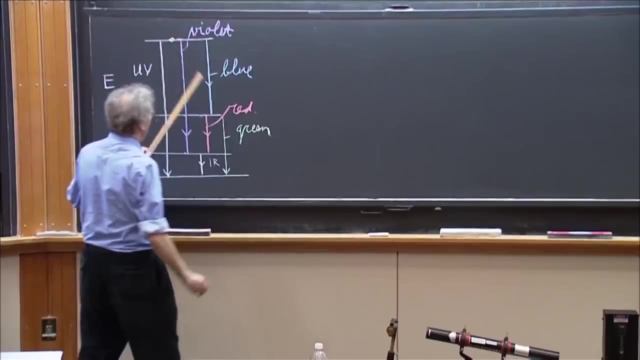 So now you get a blue photon and you get a green photon. But it could also have done something else. It could also have gone from here to here, And this is red. So now it would emit a blue photon, a red photon. 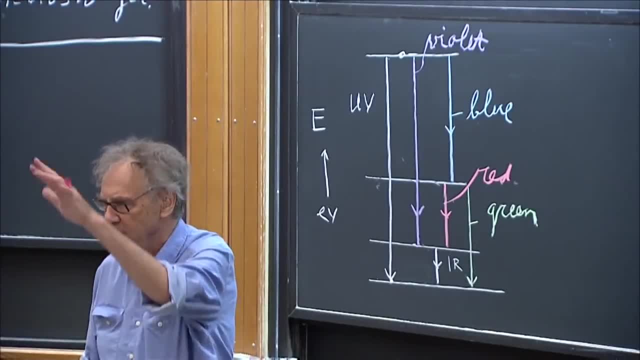 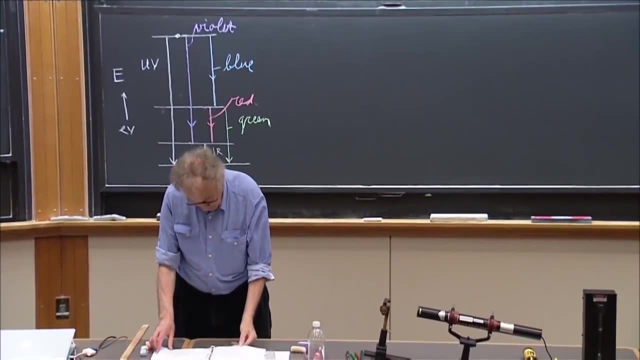 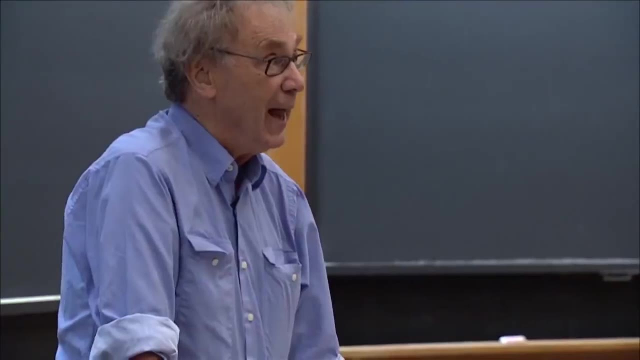 and then an invisible infrared photon. So you see, in cascading down from these high energy states of the electrons to these high energy states, they have a lot of options. So by looking at the light, for instance the light that is emitted by neon- 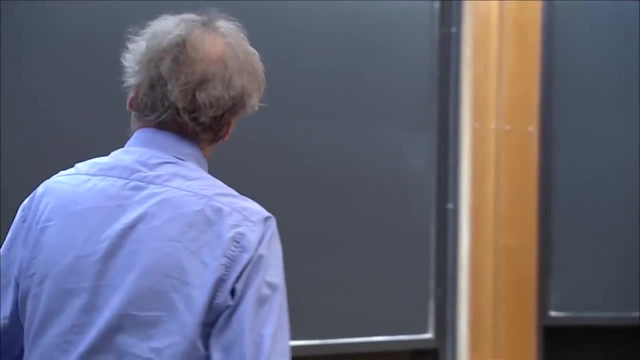 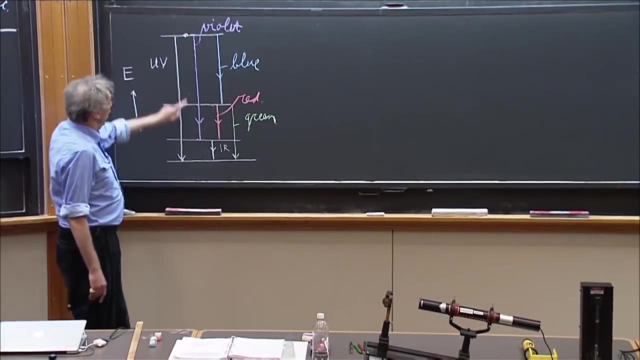 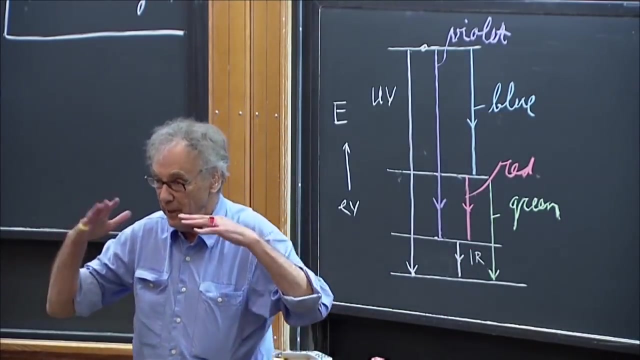 or by helium or by hydrogen. when you heat it, you will see the colors of these photons: Only the blue, only the violet, only the red, only the green, only the NIR, nothing else, nothing in between. It is a quantized situation. 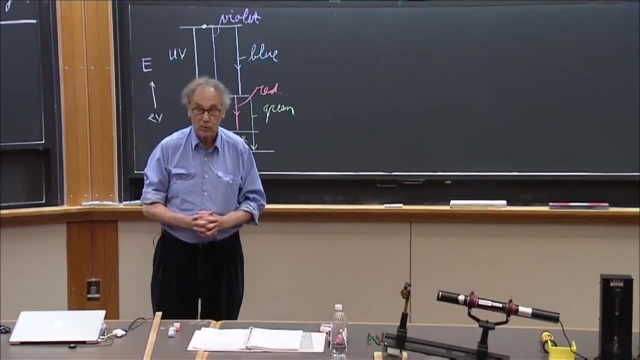 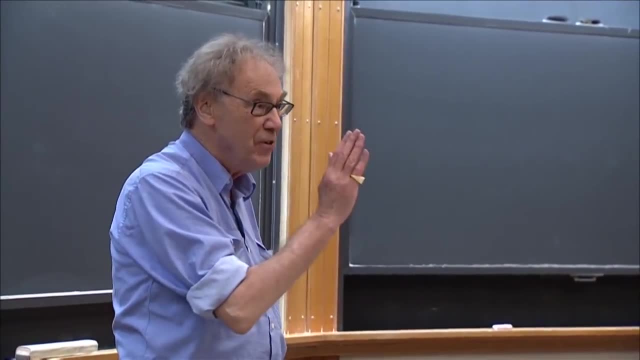 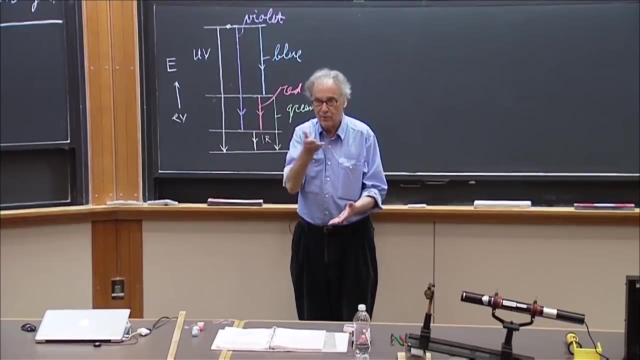 So if you look at the spectrum, if you have a spectroscope and you analyze the light, you don't see a continuum spectrum, but you see only these specific colors representative for these transitions. And so you can now figure out where the energy levels are of the electrons in the atom. 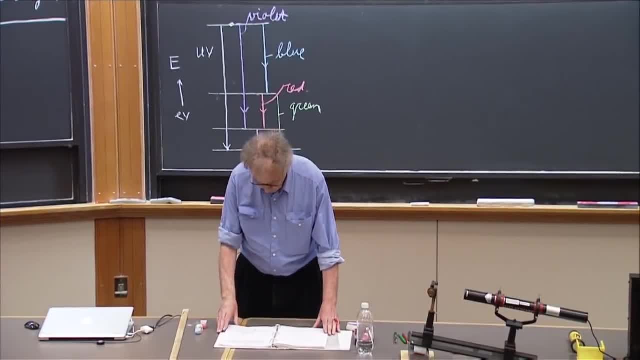 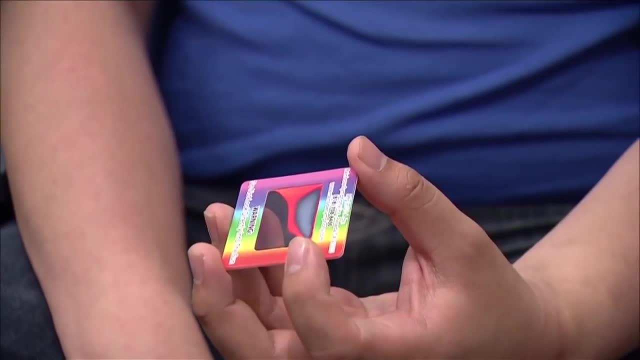 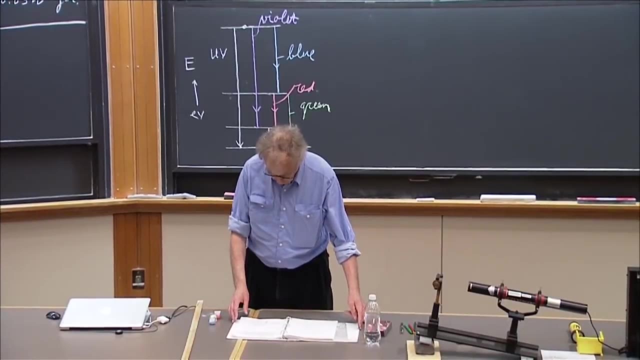 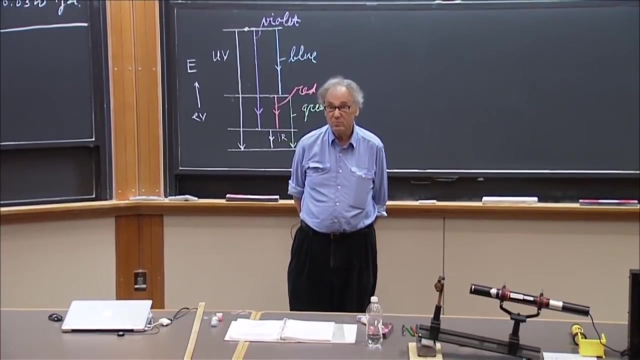 It's quite straightforward. All of you should now have a small piece of plastic, which we call a grating. Don't put your fingers on the plastic, because it loses some of its quality. It's called a grating, and a grating has the ability to decompose light into colors. 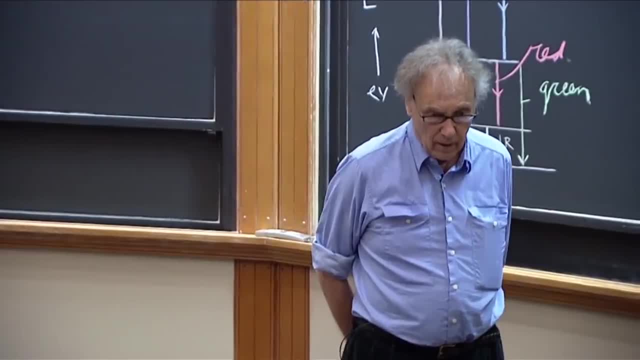 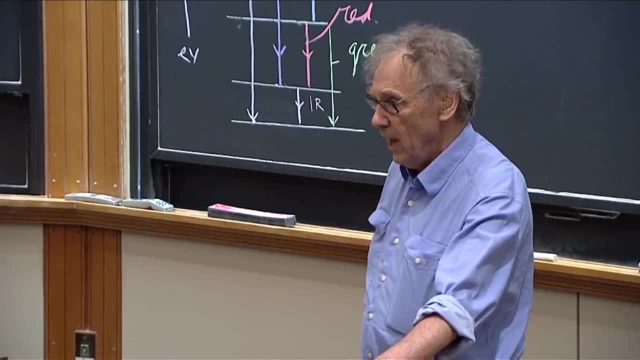 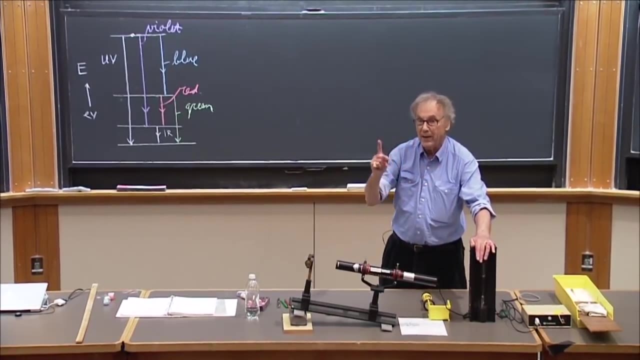 And I'm going to show you very shortly neon light from here and helium light from here, And then, with your grating, you will be able to see those unique lines, those unique energies which come out in only specific colors. But before I do that, 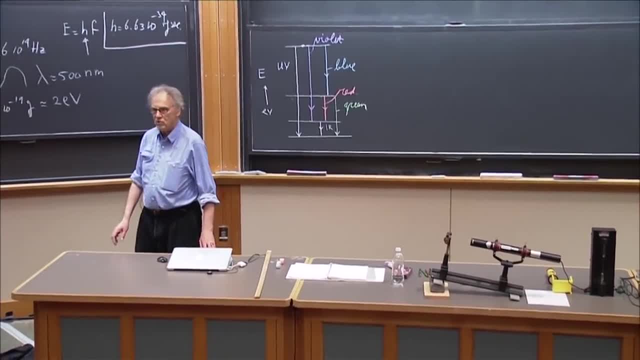 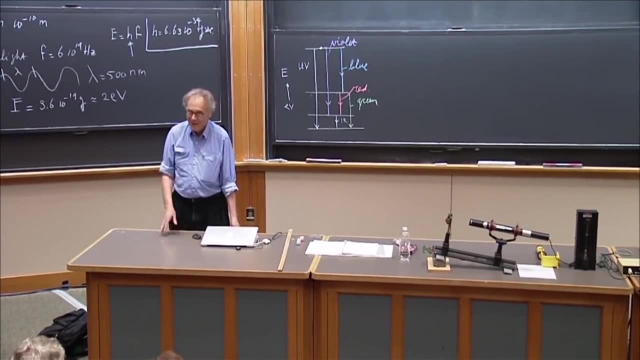 imagine that the people who are going to watch this lecture in the future on TV- you can give them a grating, but what they see on TV they won't see the lines, because that light, of course, is not really coming from helium. 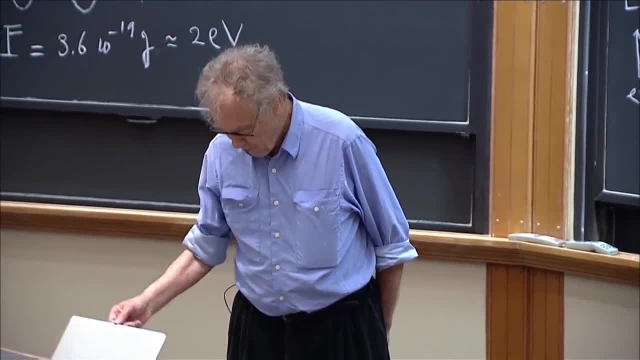 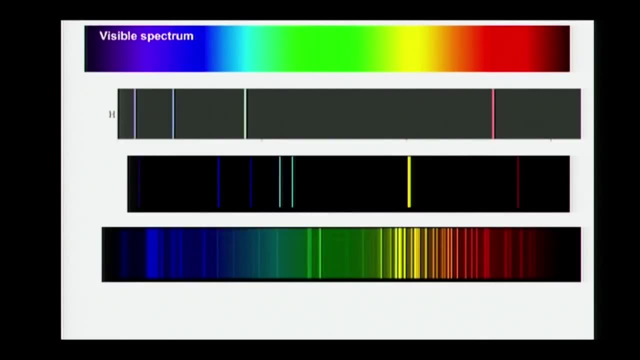 and not really coming from neon. So, therefore, I'm going to show you a slide- and that slide is an introduction for the people who watch me on TV and for the poor people who are now in 34101- to show them what you are going to see. 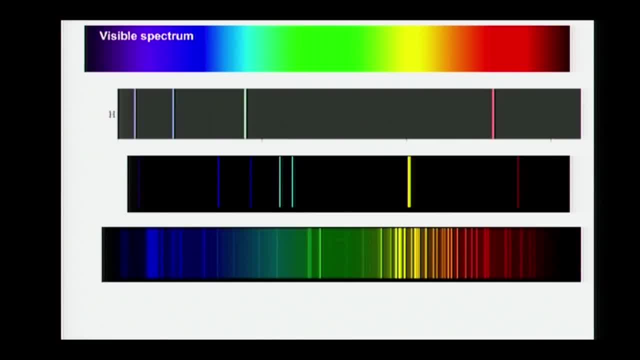 The upper spectrum is the spectrum of a solid object. that is very hot, maybe four or five thousand degrees centigrade. It gives a continuous spectrum And you see the shortest wavelengths on the left. that is violet and then you get blue and all the way to the right. 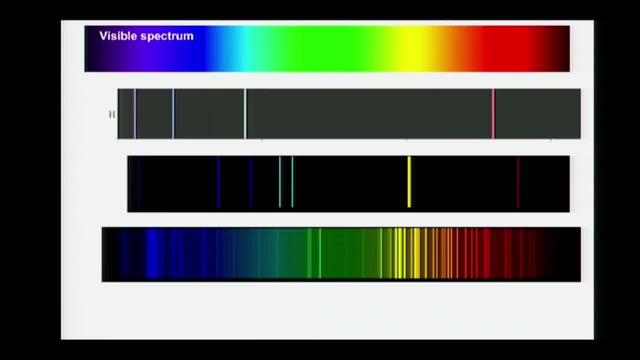 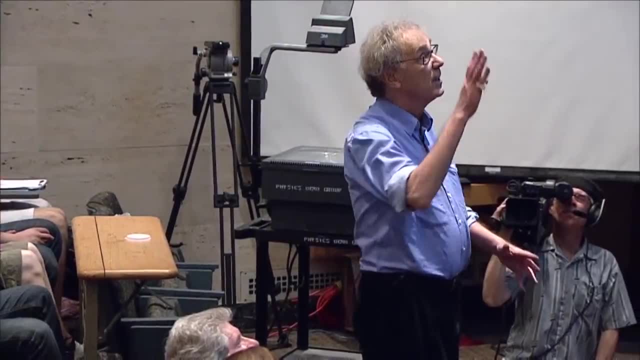 you get the red. The second spectrum from above is hydrogen. Hydrogen has only four lines in the visible part of the spectrum. There are more outside the visible, but in the visible part there are only four, And when I prepared this 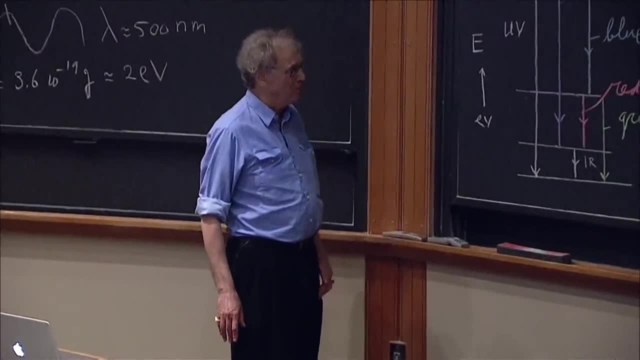 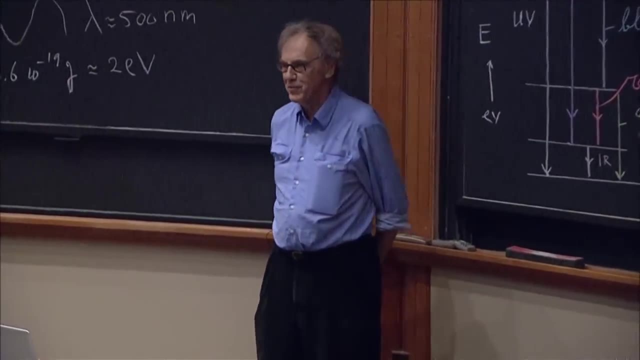 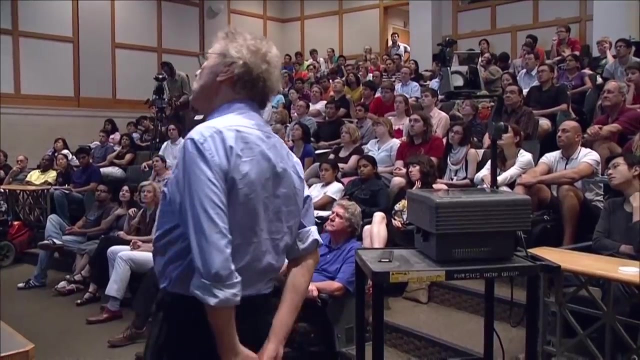 I didn't choose these levels in a specific way, but it turns out that I also have only one, two, three, four in the visible, purely log, But hydrogen has only four in the visible and there are several that are in the UV. 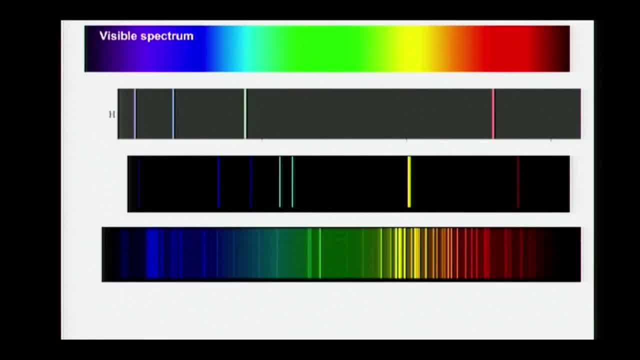 and that you would not be able to see. And then, when you go one step down, you see helium, And helium, I'm going to show you- Hydrogen has only one electron, So you really don't expect too many of these levels. 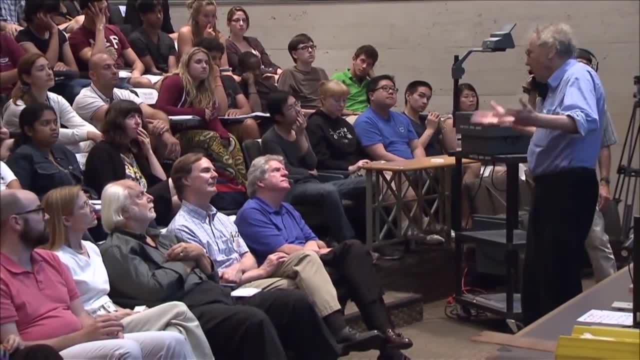 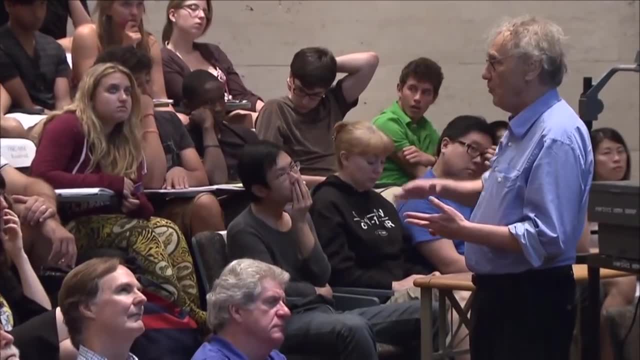 Your intuition tells you: if you only have one electron, how many levels can you have? Helium has two electrons, so you already expect more of these quantized levels. So you expect more lines, and you indeed see more lines If you go to neon. 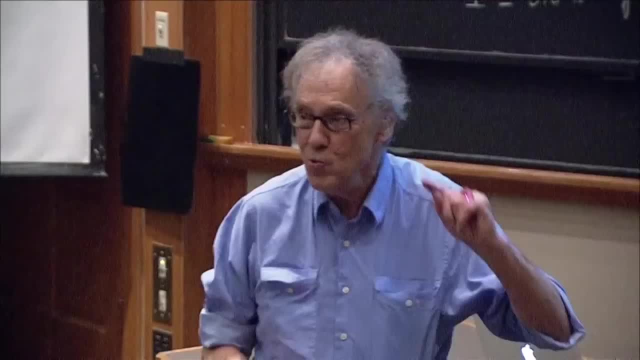 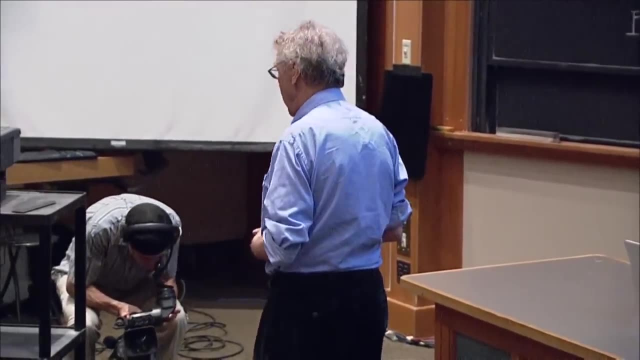 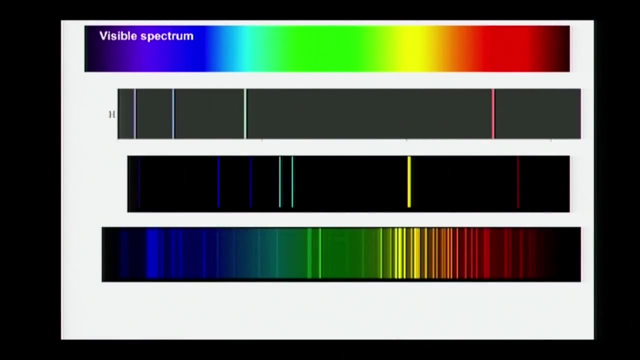 which has ten electrons. you expect a whole zoo of energy levels, And so you expect an enormous number of these emission lines, of these photons, and indeed that's what you see. Neon has an enormous number of these spectral lines. We're going to leave this on. 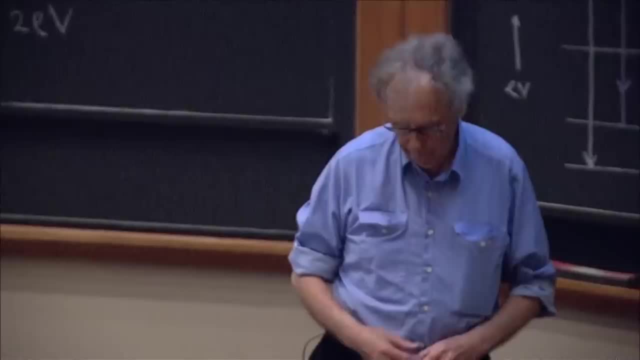 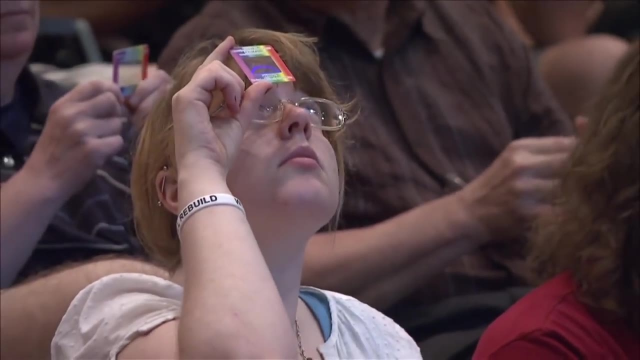 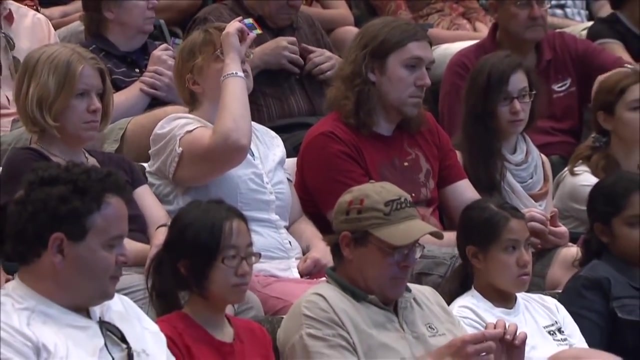 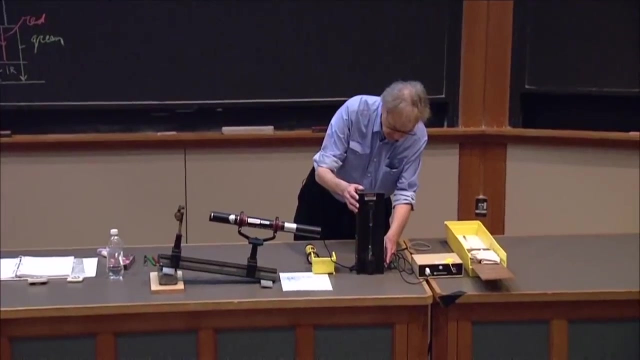 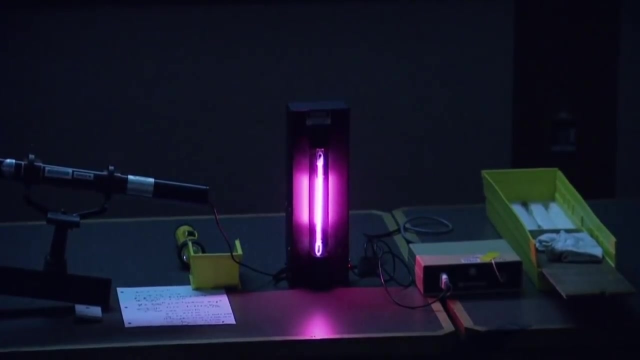 while you now take your grading out, And the first one that I'm going to show you is helium. Yeah, helium is this one, and we're going to make it dark. Just turn it on. When you use your grading, you can turn it in many ways. 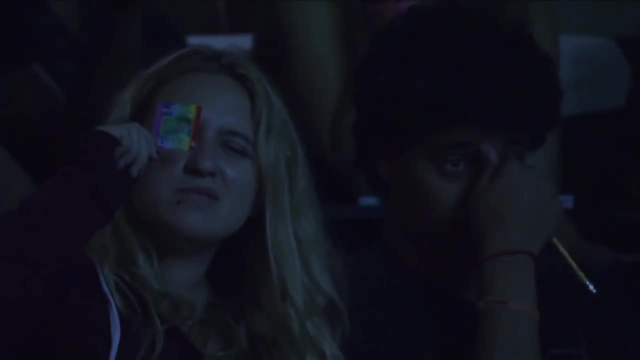 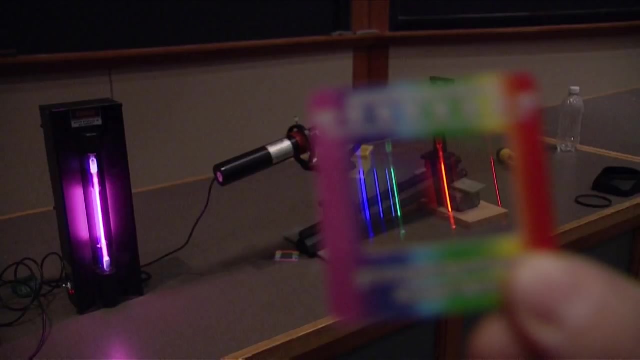 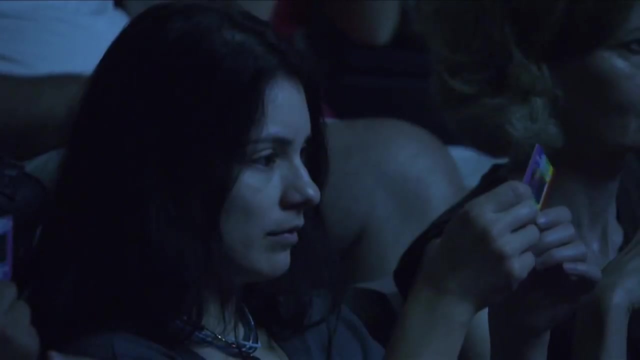 I want you to turn it in such a way that if you look all the way in the right side, so you look towards the right through your grading, that you then see vertical lines, And the vertical lines that you see are really vertical, because my lamp is vertical. 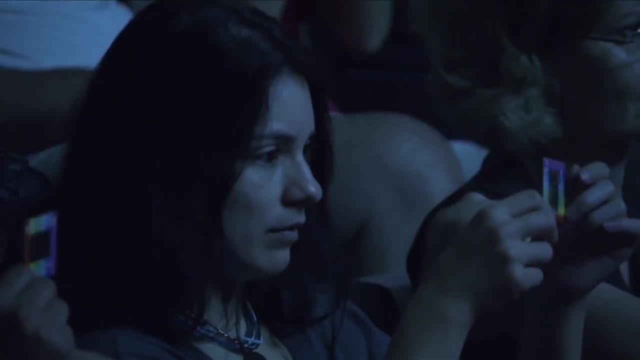 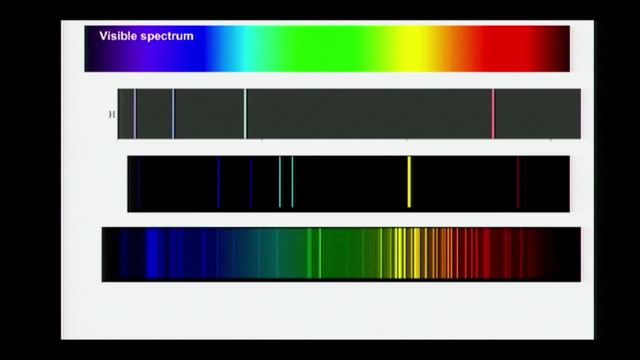 That's the reason, And when you look at it, you will see very much the same helium lines that you see there very closely. If you look all the way at the left, you will see the same spectrum, but it's a mirror image. 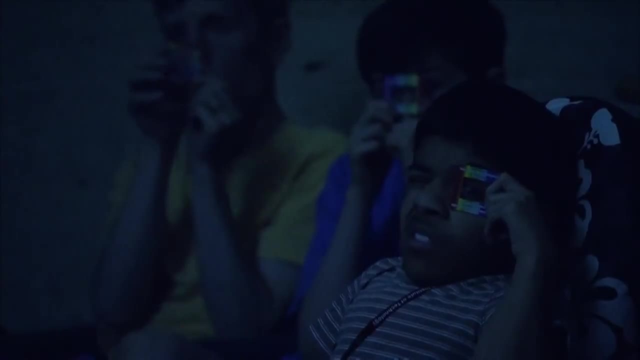 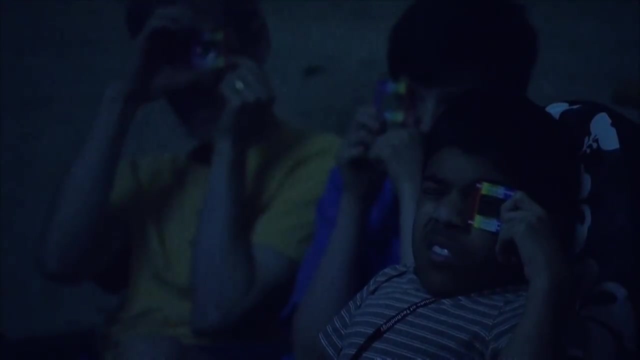 And so, since it's the same, it's not useful to look both at the left and the right. Just so keep looking at the right, then you will first see, on the left side, the blue, and then, when you go to the right, 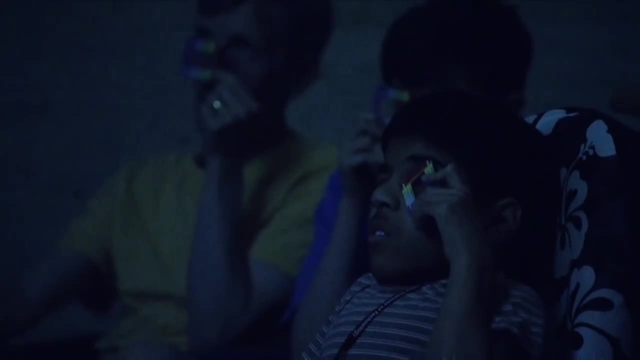 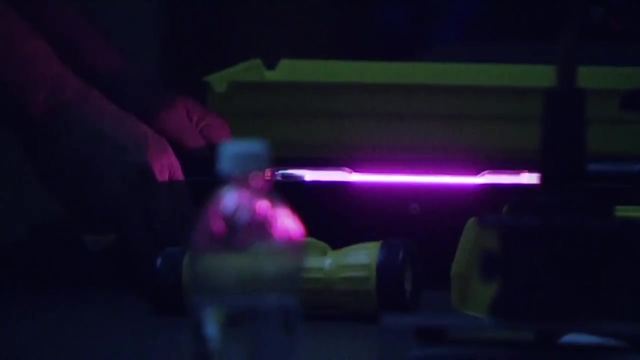 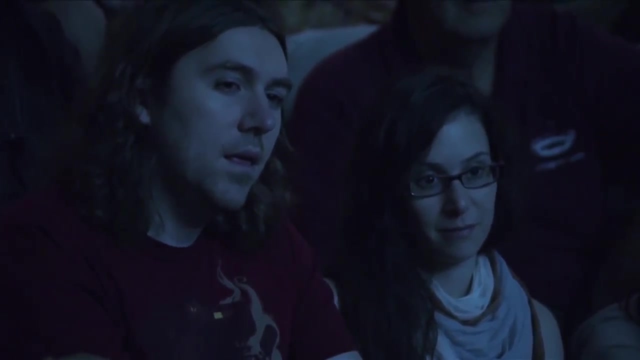 you will see the red. Now we're going to put in a neon, And this is very hot so I have to be careful that I don't burn myself. So now we're going to put in the neon. And now compare this: 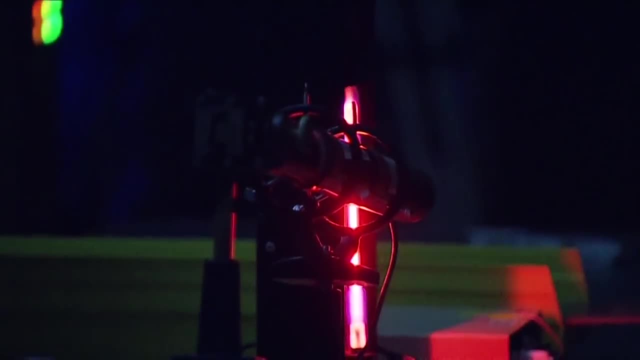 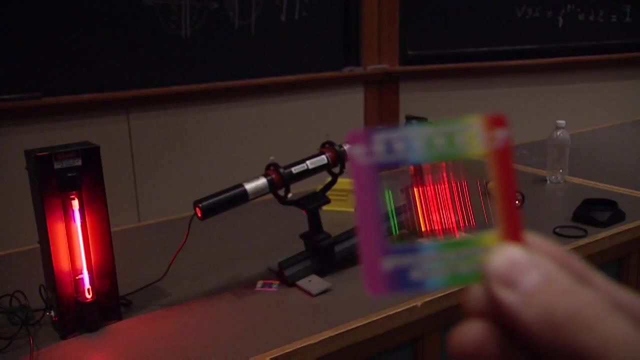 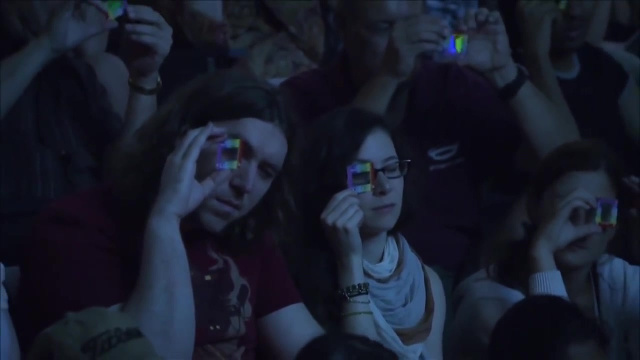 with what you see on the slide. You see the huge number of lines on the right side which is red. That's the reason why neon, when you see it with color, is red And in the commercials it's so reddish the light. 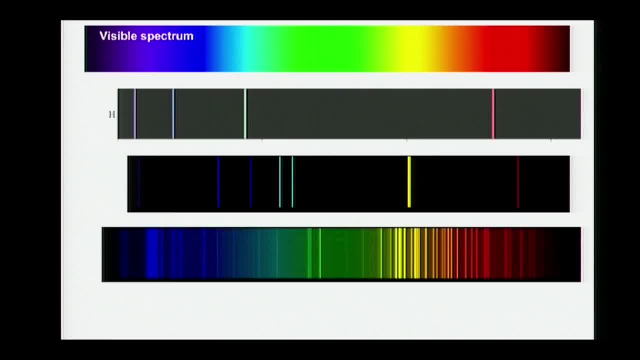 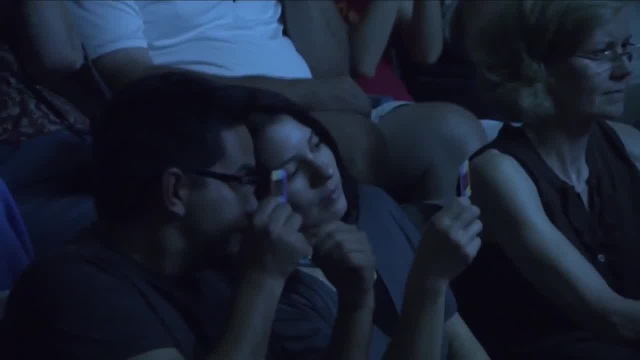 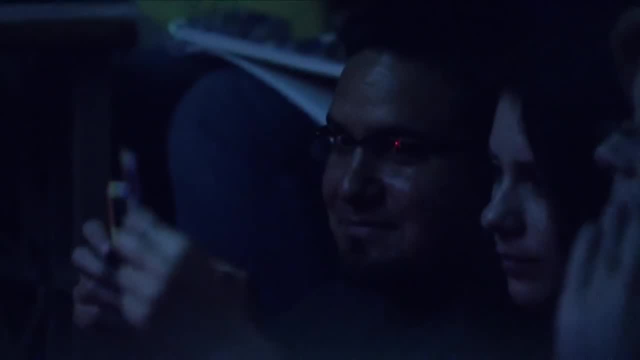 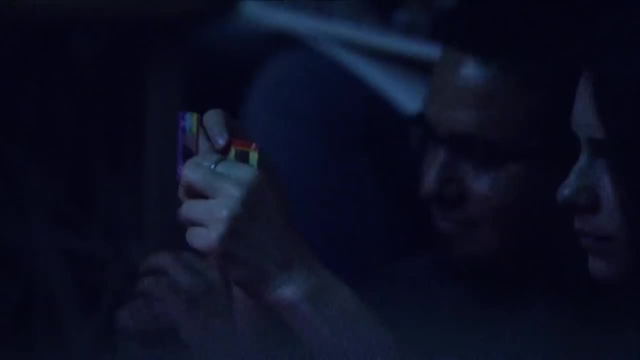 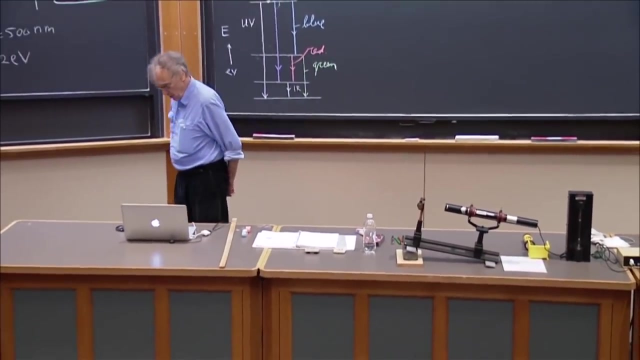 So look all the way to the right, then you see the line spectrum of neon. It's ten electrons. These gradings you can keep as a souvenir And I would like you at home to use it, And also on the streets, On the streets. 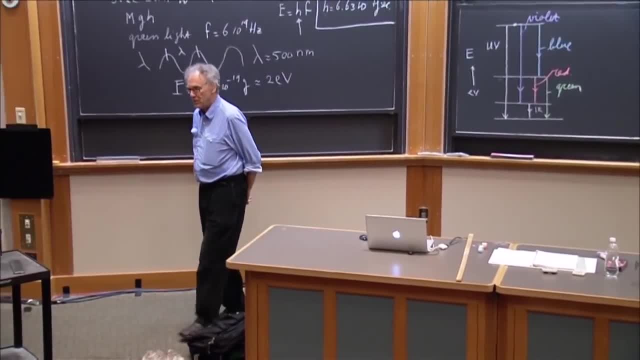 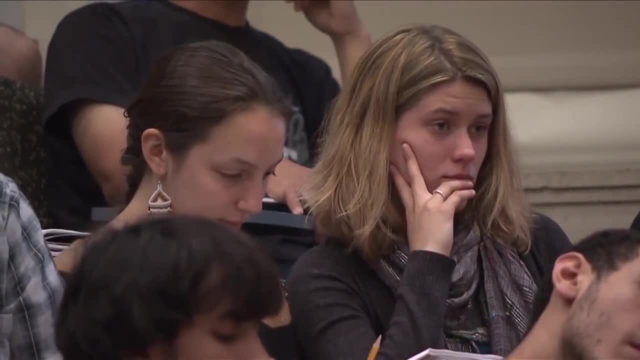 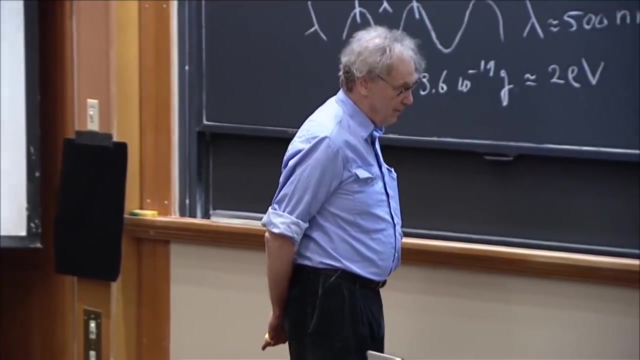 there are lamps which have mercury, Beautiful lines in mercury. Some lamps are sodium. Not too exciting, but two nice yellow lines in sodium lamps. And then there are neon, So you can also use it on neon. But what may be even more interesting? 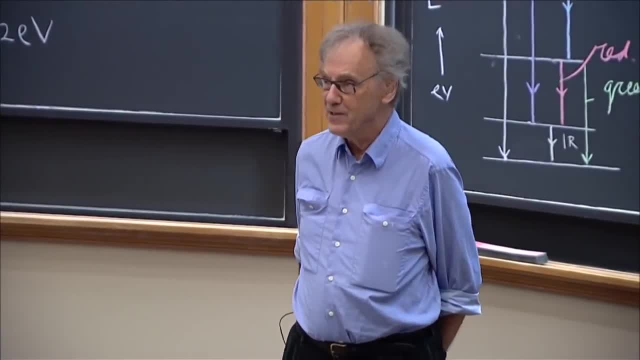 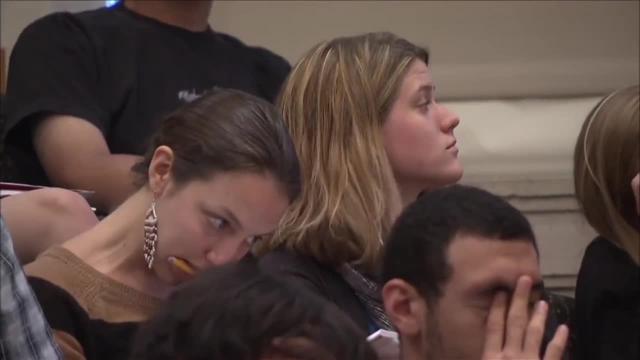 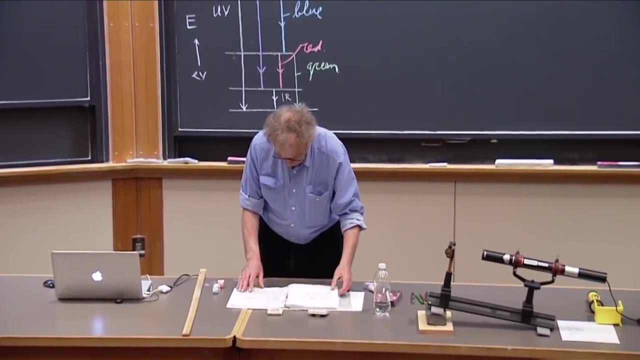 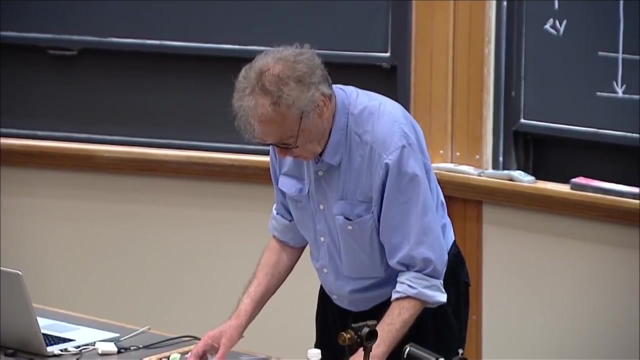 just look at an incandescent lamp. then you don't see any lines at all. Then you see a continuum spectrum, as I showed you, which was the spectrum at the top. So use it. Quantum mechanics took a big leap in the twenties and it would not be possible. 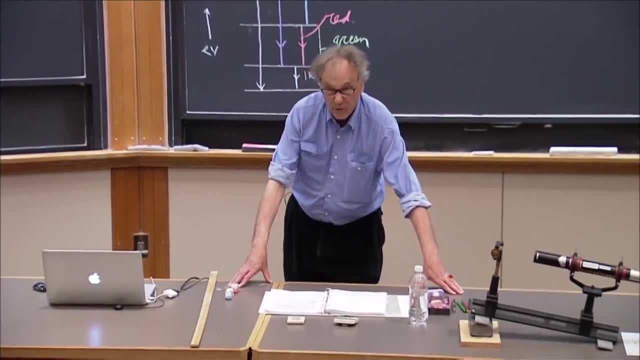 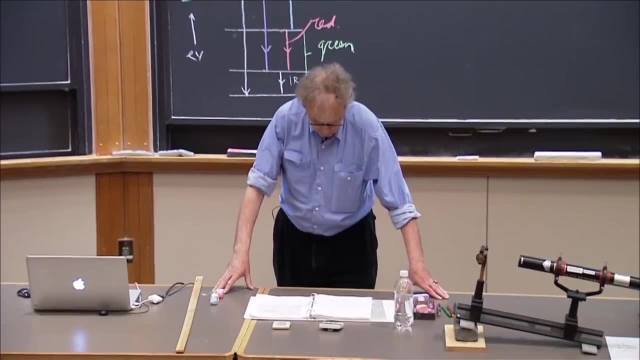 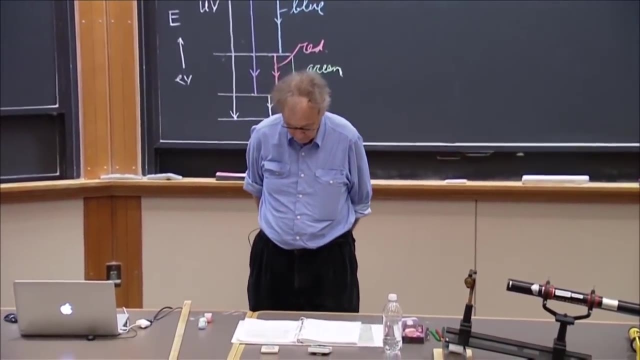 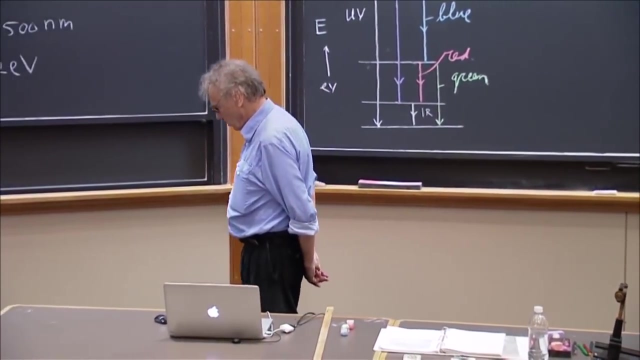 in a considerable time to do justice to all the basic concepts. However, we already have discussed the discrete levels, and I want to discuss at least one more very non-intuitive consequence of quantum mechanics. For one thing, prior to quantum mechanics, there was a battle. 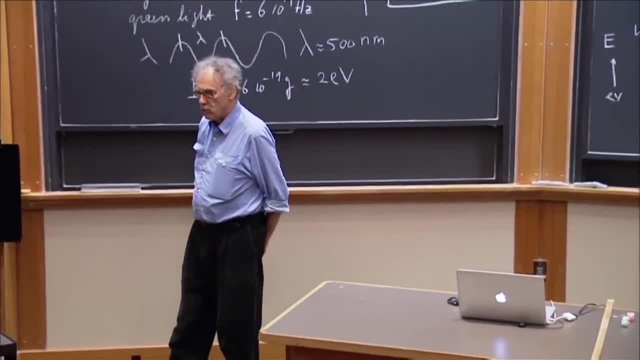 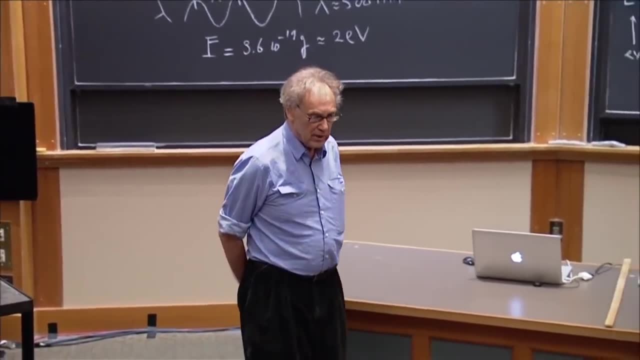 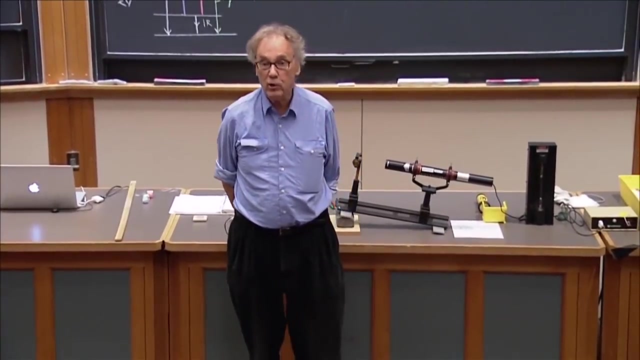 between Newton in the seventeenth century, whose name is Huygens. Newton said light is particles and Huygens says no, light are waves. I have learned to pronounce Huygens incorrectly, because the correct way to pronounce it is Huygens. 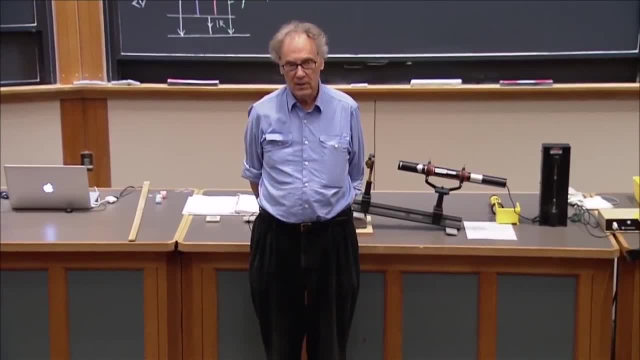 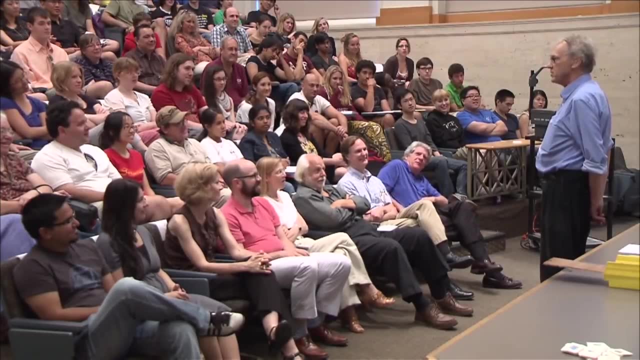 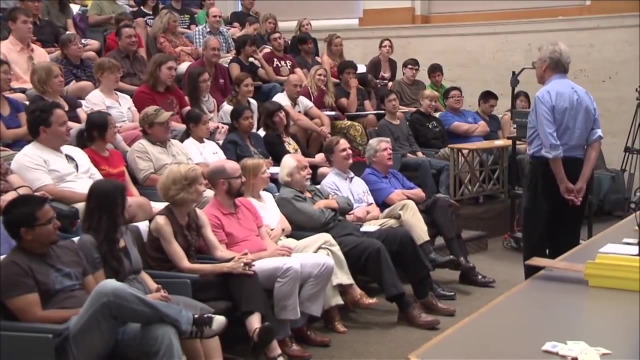 But since you don't have an in your language and you don't have a in your language, you cannot say Huygens. so I have adopted Huygens for the years and I call it Huygens. However, if anyone in my audience can really say Huygens, 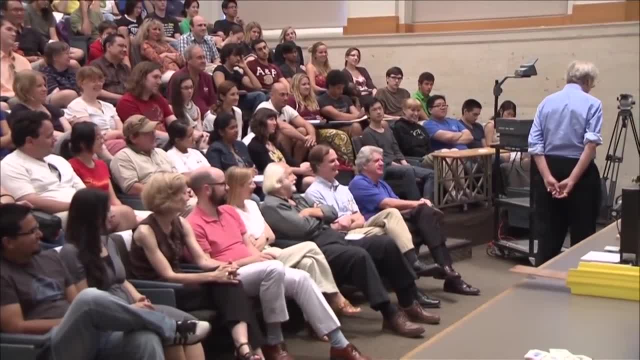 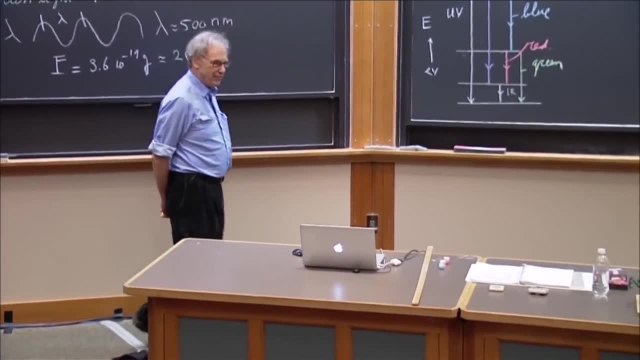 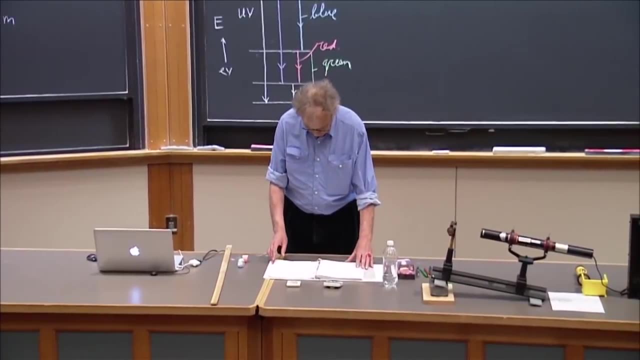 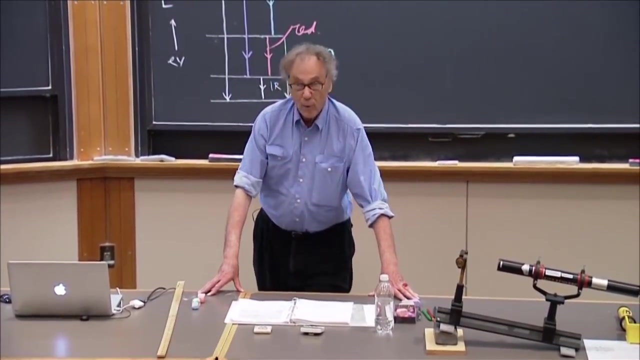 they are Dutch for sure. In 1801 the battle between the two was more or less settled by Jung, and it came out in favor, overwhelmingly in favor, of waves Around 1801. the general idea was that as time went on, discomfort was growing and there were also experiments. 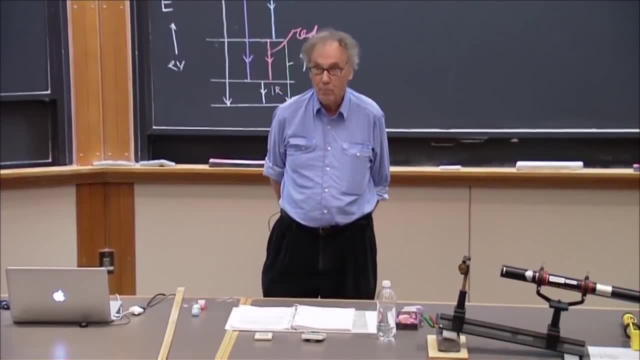 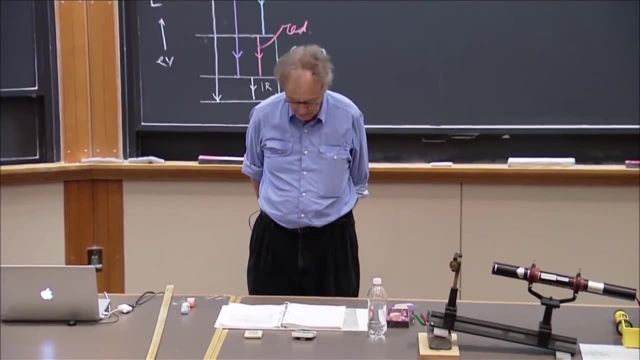 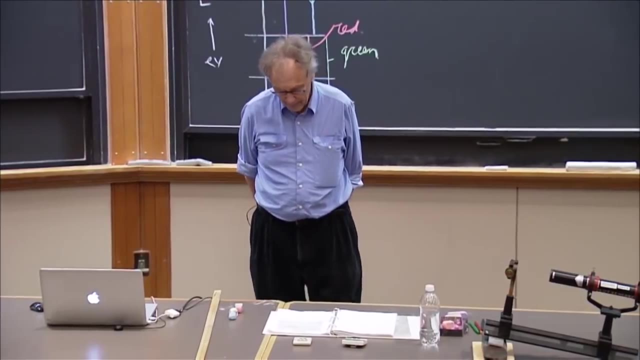 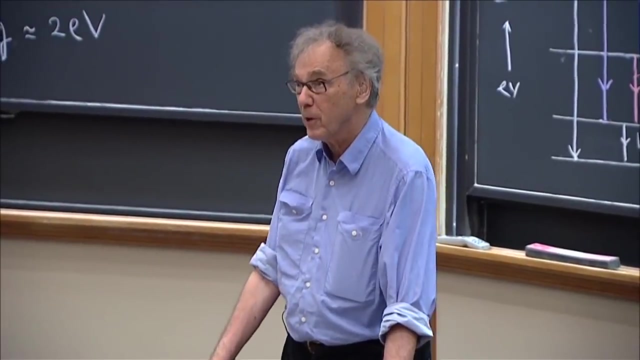 that showed rather conclusively that light really behaves also like particles, And it was one of the great victories of quantum mechanics that it showed that light is both. At times light behaves like waves and at other times, depending upon how you do your experiments, light behaves. 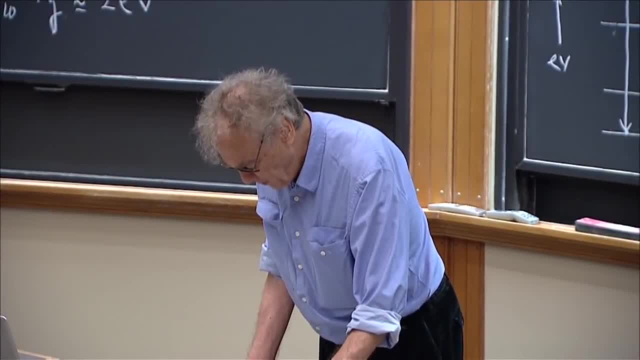 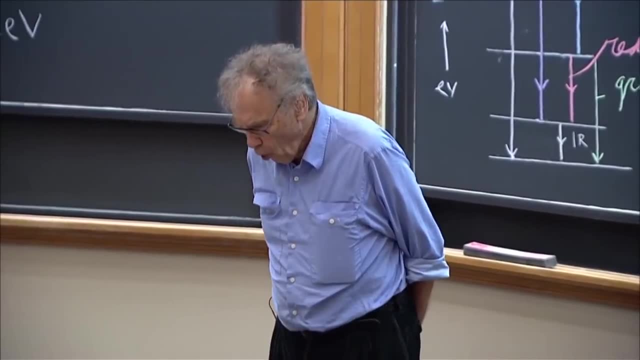 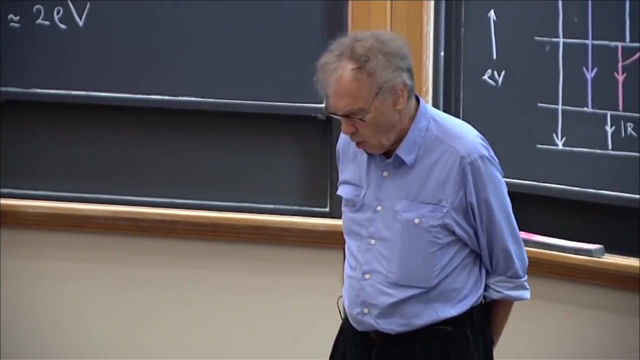 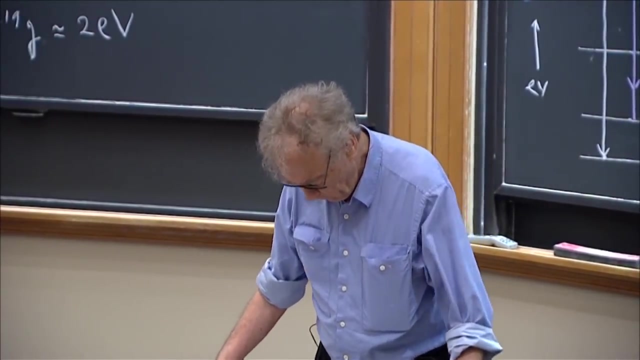 like particles. In 1923 Louis de Broglie made the daring suggestion that all particles can behave like waves, And the smaller the mass and the lower the speed of the particle, the larger, he said would be the wavelength. So he used first the concept. 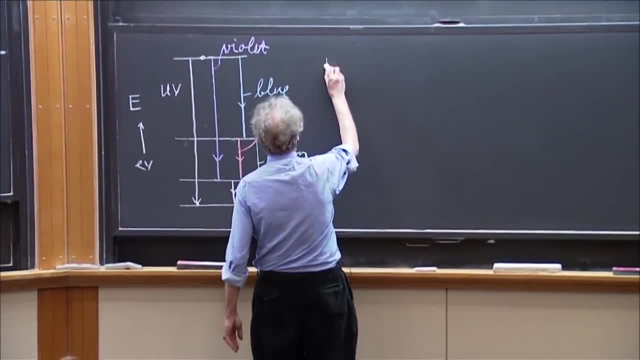 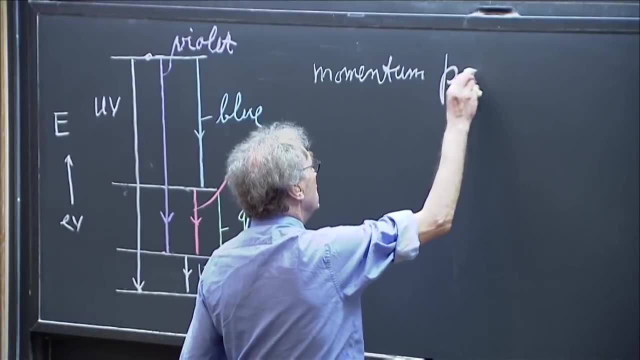 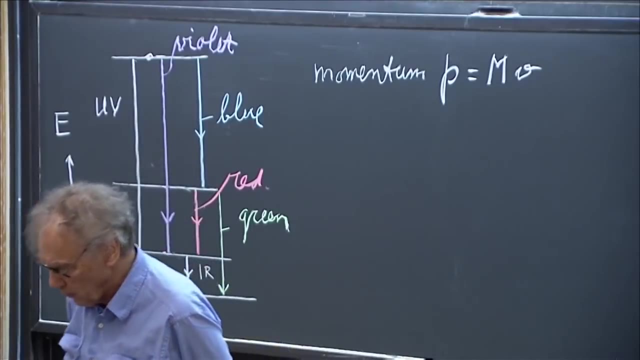 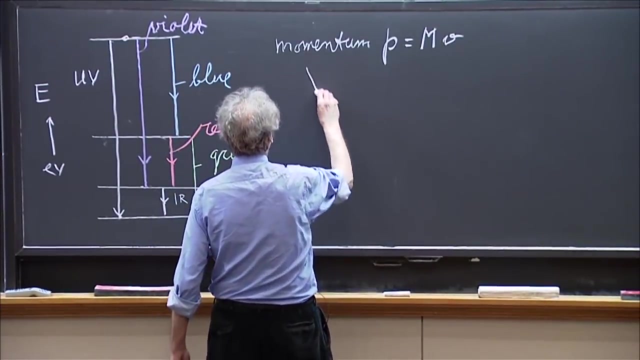 of momentum. I assume that most of you already know what momentum is. The momentum of a particle is: P is the product of the mass of the particle times its velocity, And so Louis de Broglie came with the suggestion that the wavelength of a particle 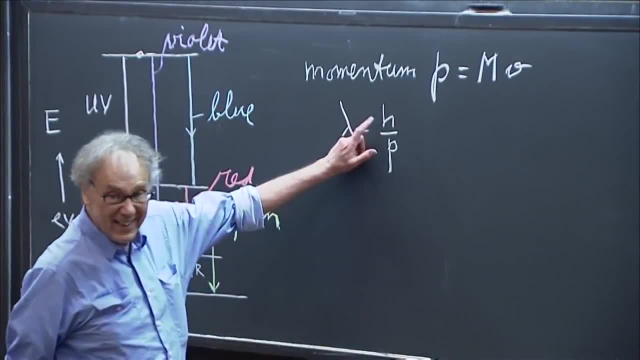 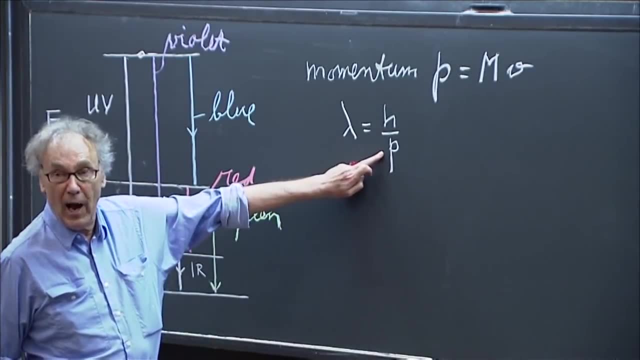 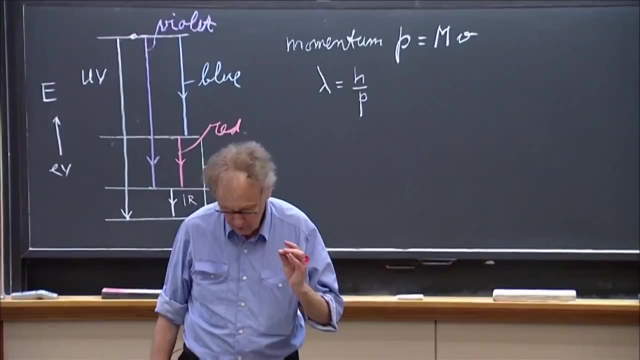 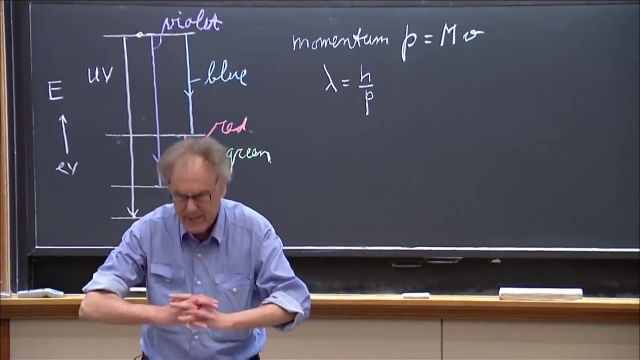 equals H divided by P, H. again, That is Planck's constant. And so you see, a particle with an enormously high momentum would have a very low wavelength. So he says all particles can behave like waves. Now, if he is right, that means 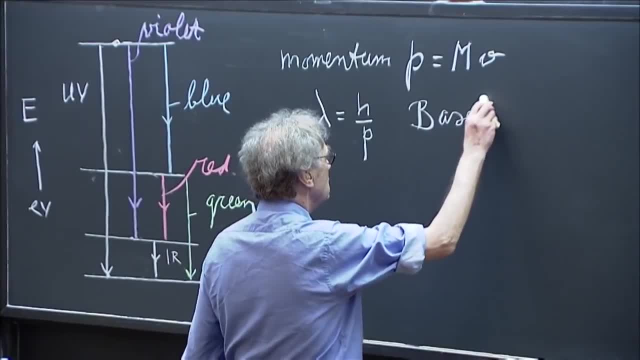 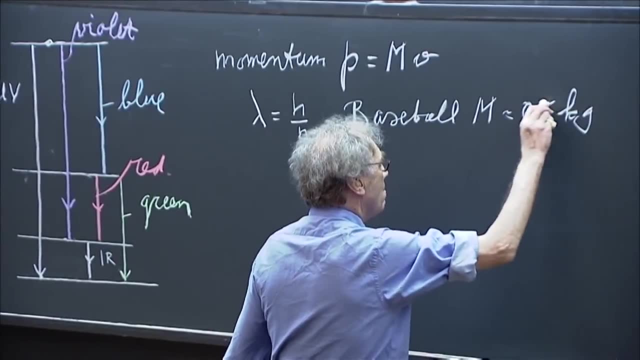 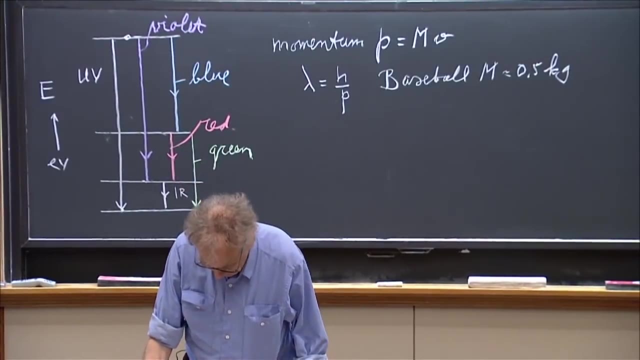 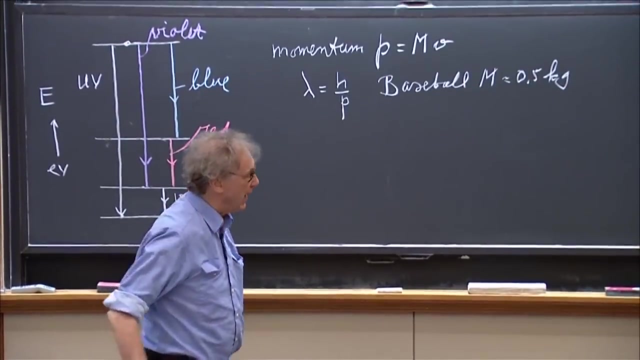 we are now talking about a baseball whereby the mass is about half a kilogram and we give the baseball, say, a speed that is doable. I've heard of it, a speed something like close to 100 miles per hour, 44 meters per second, so V. 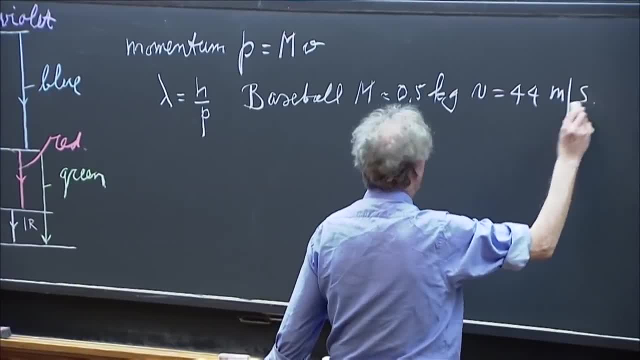 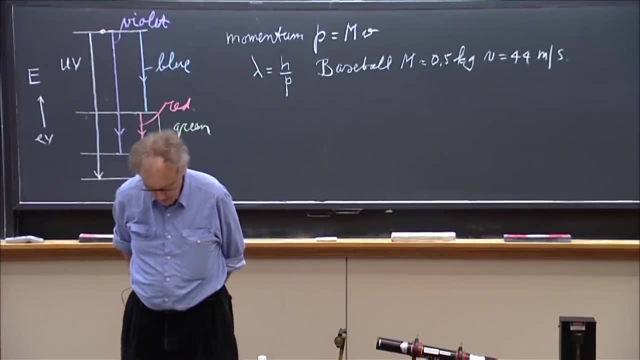 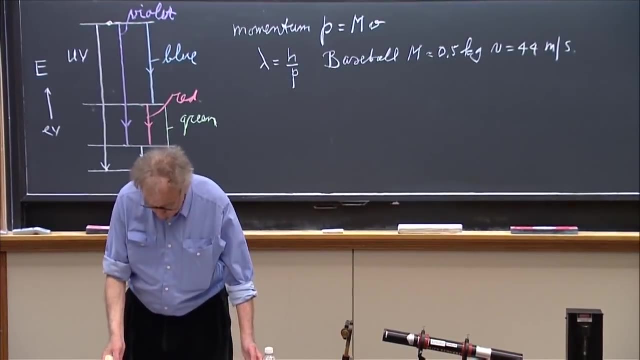 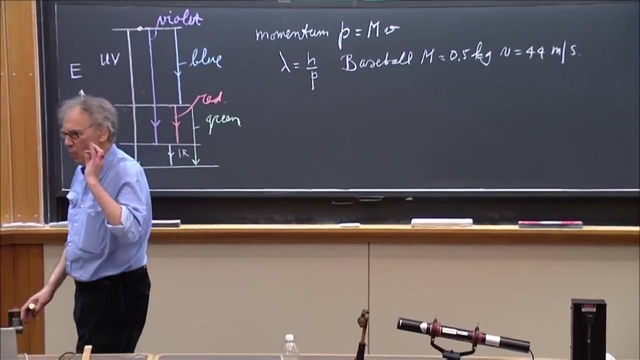 is 44 meters per second. then we can ask Mr de Broglie what is the wavelength? And the answer is that the wavelength is 20 orders of magnitude smaller than the size of a proton- 20 orders of magnitude, that is a one with 20 zeros. 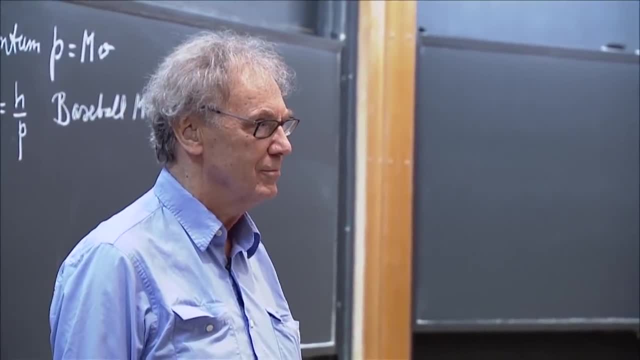 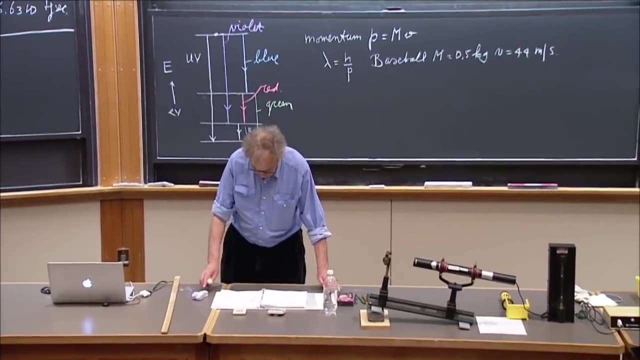 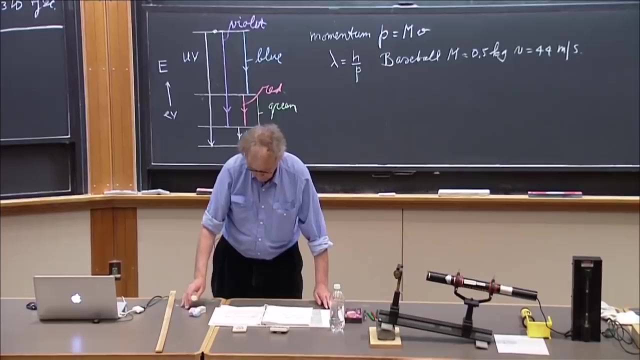 times smaller than a proton, So it's meaningless. Again, as I said earlier, quantum mechanics doesn't play a role in our daily lives of tennis balls and baseballs, But let's now turn to an electron. So now we're going to change from a baseball. 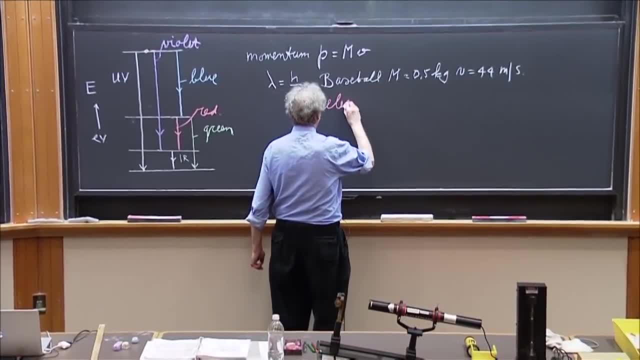 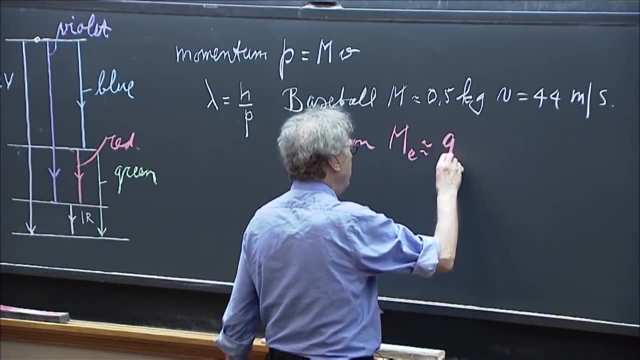 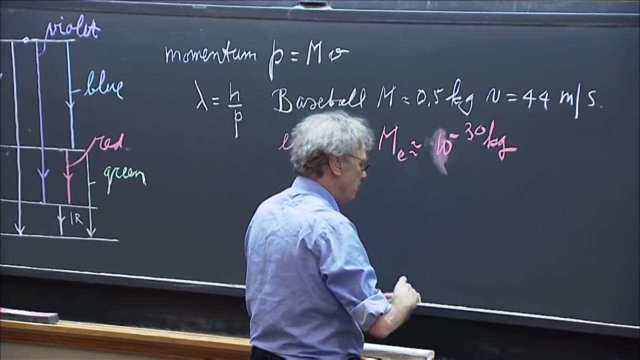 I use a different color so that you can really see the difference. I now go to an electron. It's about nine, or I forget the nine, 10 to the minus 30 kilograms. I'll clean this up because it looks so bad on television. 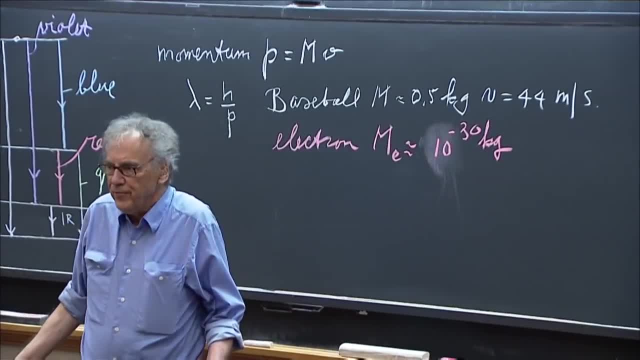 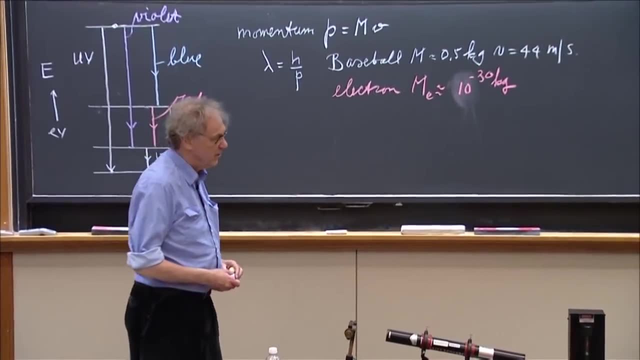 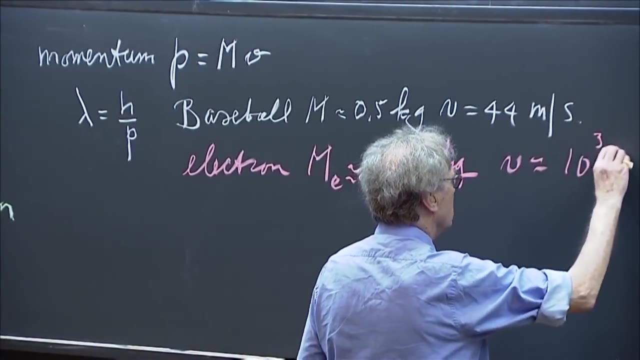 10 to the minus 30 kilograms. And if I give an electron a modest speed of thousand meters per second, which is about 3600 kilometers per hour, is about 1000 meters per second. If now I ask Mr de Broglie, 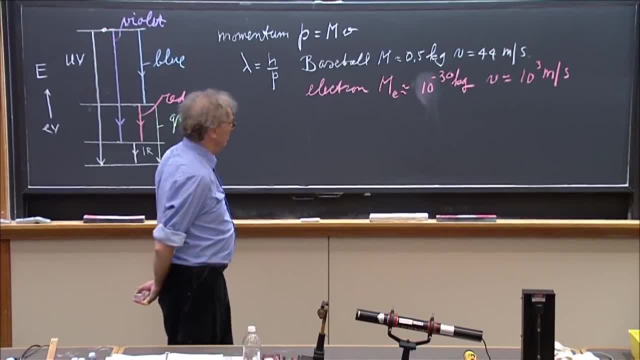 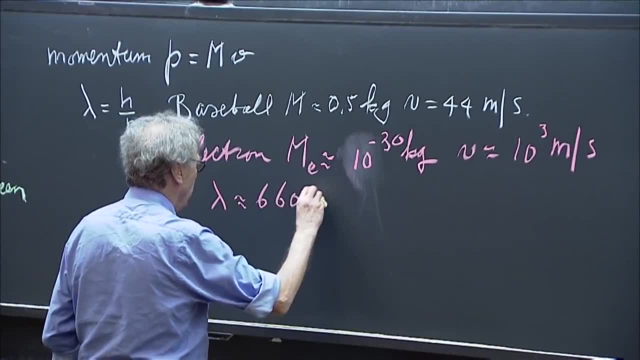 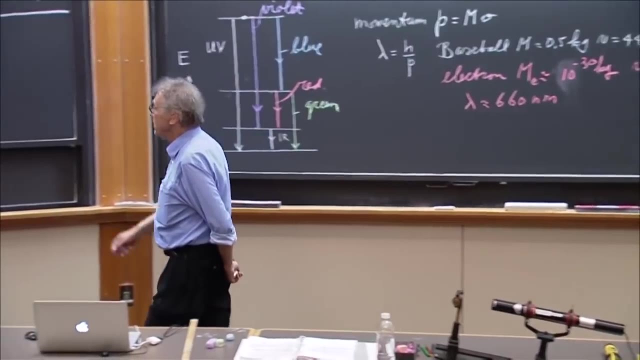 what now is your wavelength? you can calculate using Max Planck's constant that lambda is approximately 660 nanometers. Well, that is a meaningful answer. It means if green light has a wavelength of 500 nanometers, then 660 nanometers is a reasonable number. 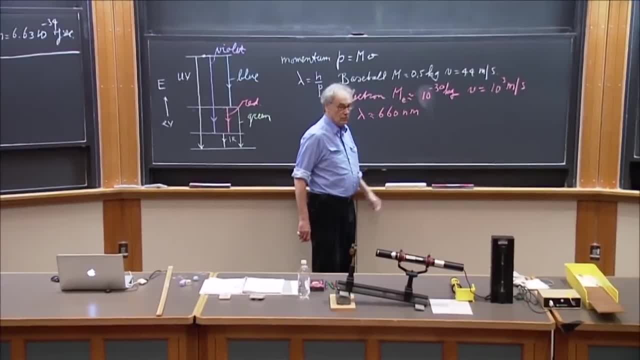 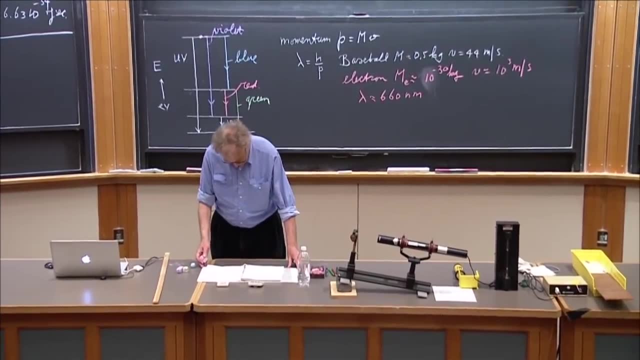 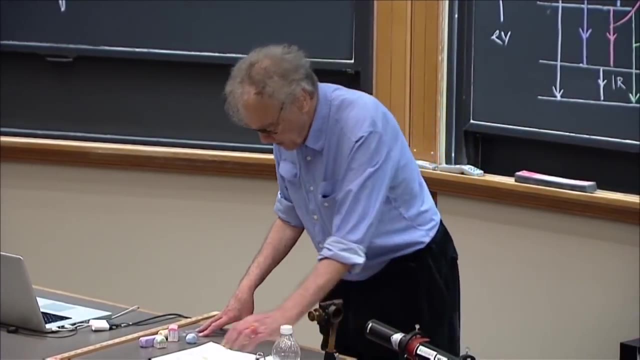 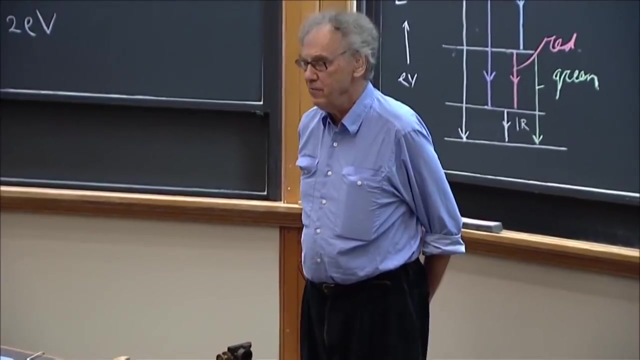 It is equivalent in terms of color red light. So you see, de Broglie makes sense for electrons, but not really for baseballs. In 1926, the Austrian physicist Schrödinger drove the nail in the coffin when he formulated a very famous equation. 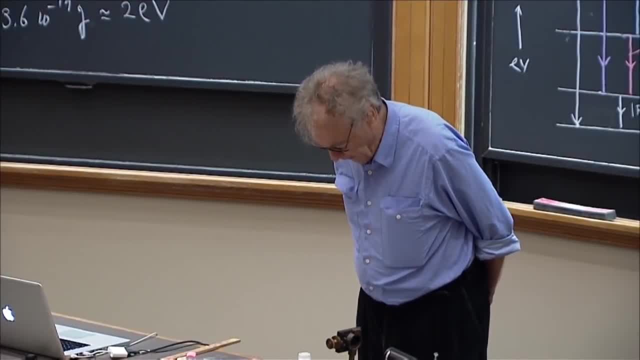 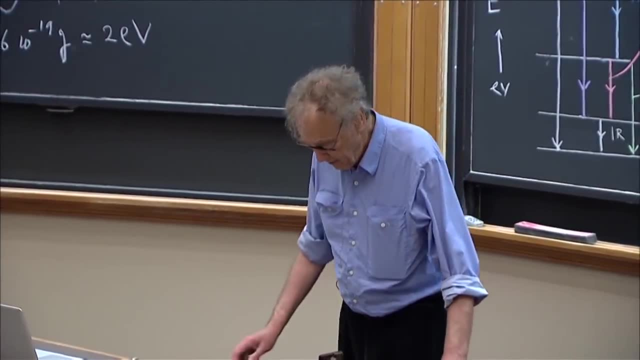 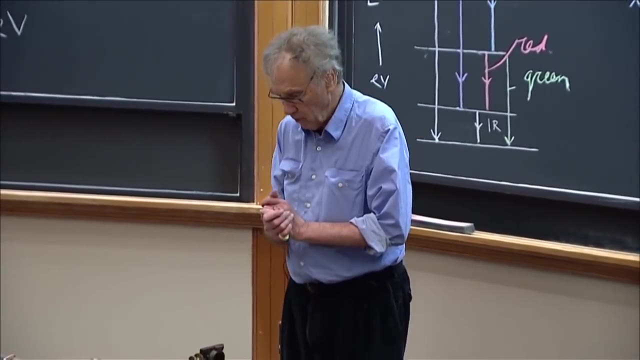 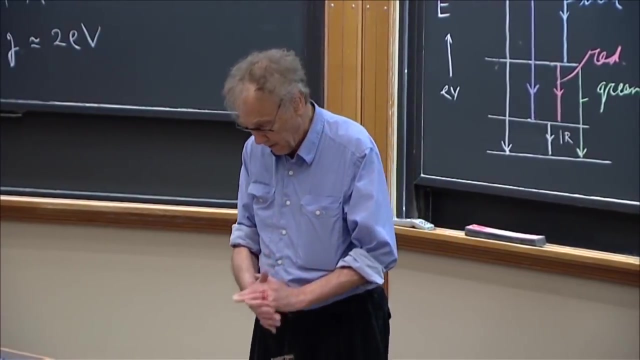 and that is really the ground pillar of quantum mechanics, in which he unified the wave and the particle character, And indeed all electromagnetic waves, that means radio, x-rays, UV, infrared optical light- can behave like particles and all particles- protons, neutrons, electrons. 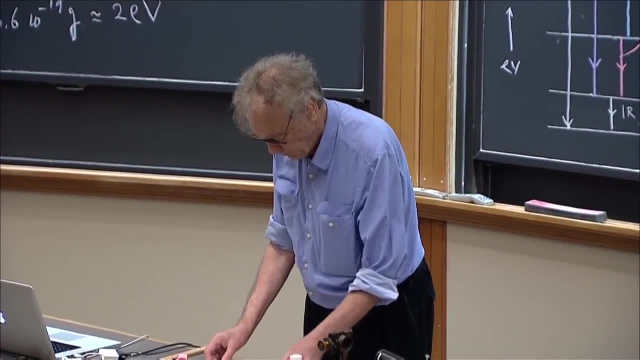 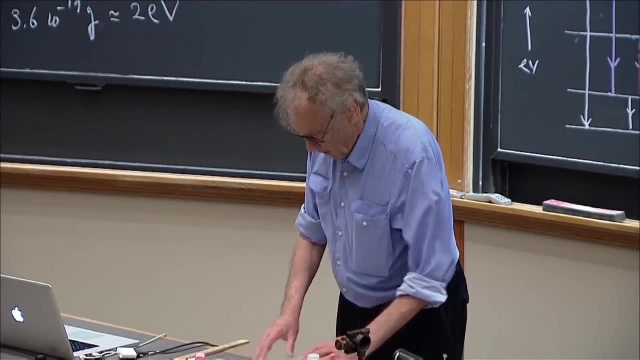 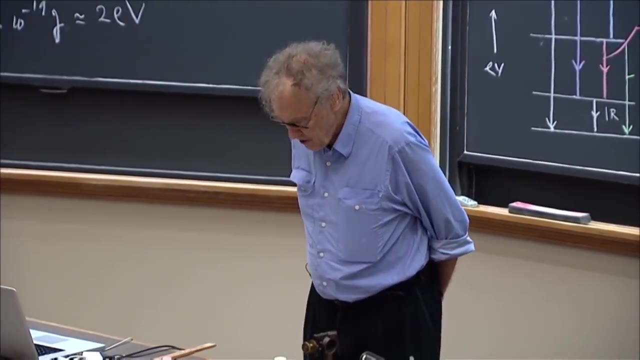 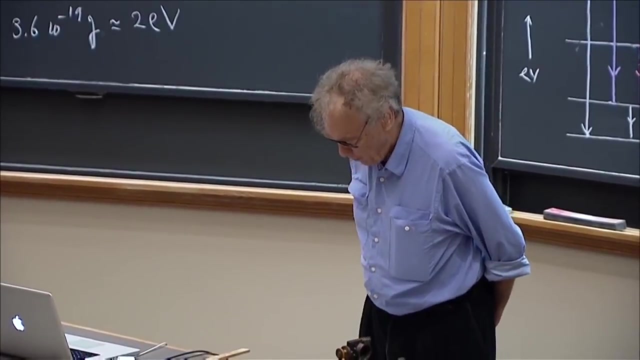 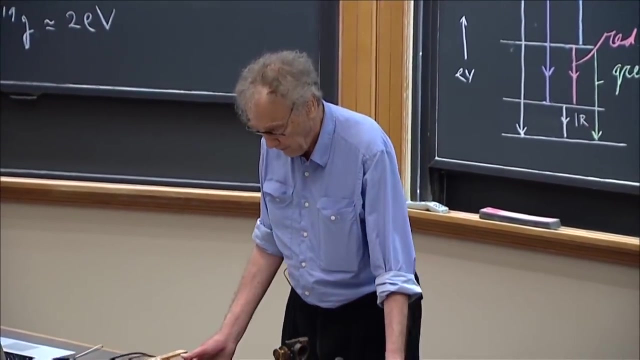 can behave like waves. In classical Newtonian mechanics, you should be able to determine the position of a particle very accurately, where it is located, and at the same time you should be able to determine its momentum very accurately. There is nothing in Newtonian mechanics but the German physicist. 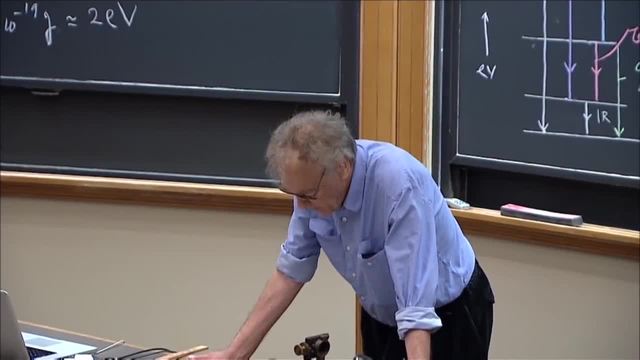 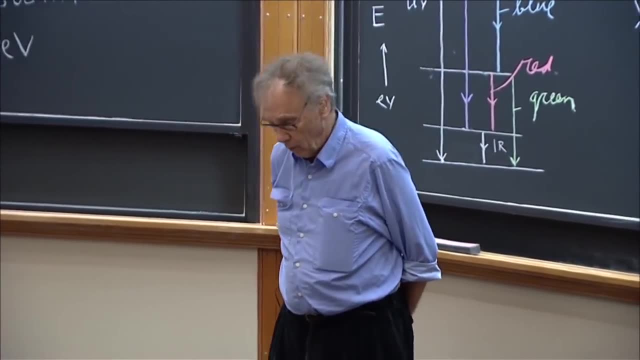 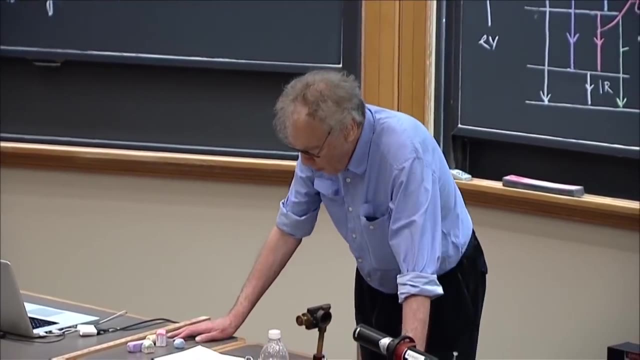 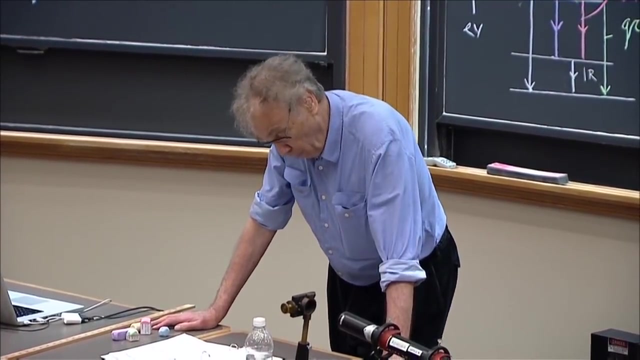 Wernher Heisenberg realized in 1927 that a consequence of quantum mechanics is that it is not possible. Strange as it may sound, Heisenberg proved that the position and the momentum of an object cannot be measured very accurately at the same time. 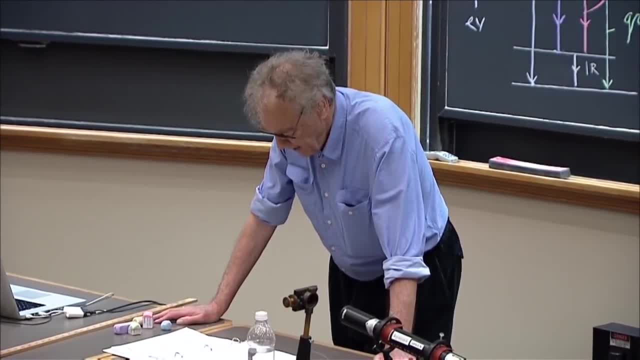 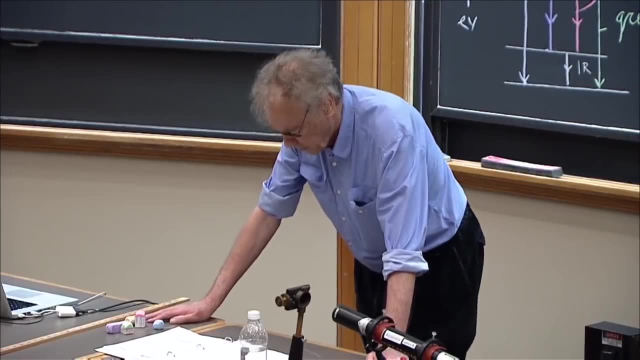 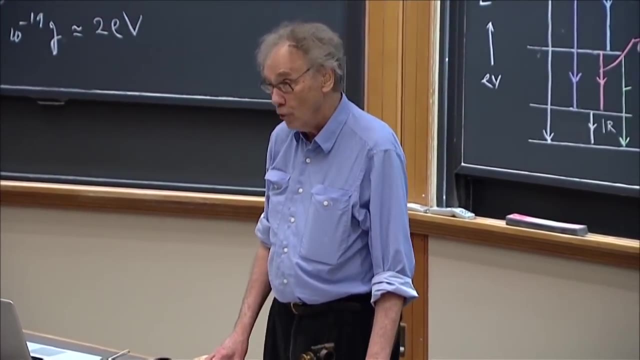 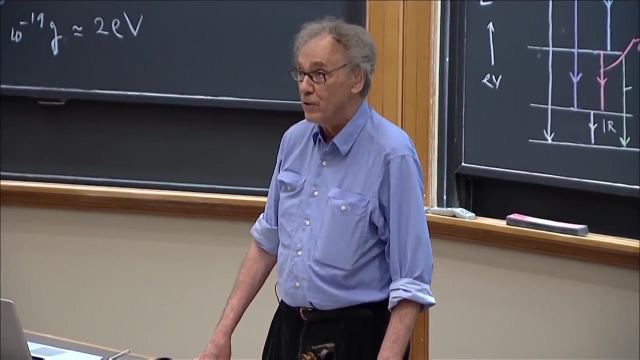 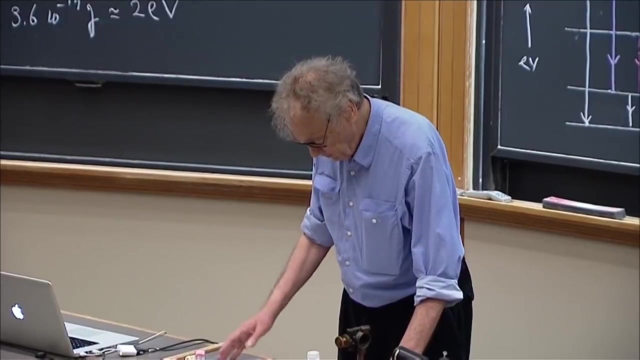 The two concepts of exact position of an object and its exact momentum together have no meaning in nature, And this is called Heisenberg's uncertainty principle, for which he was awarded the Nobel Prize. De Broglie also received the Nobel Prize. This whole idea. 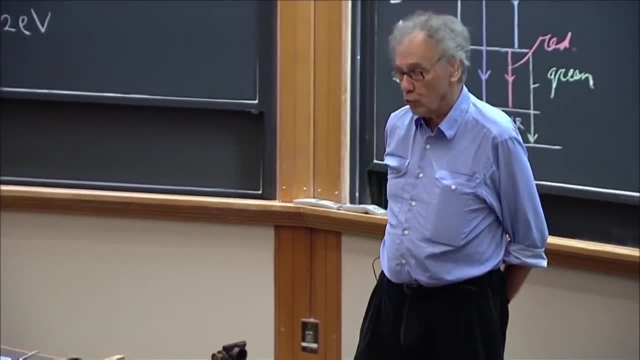 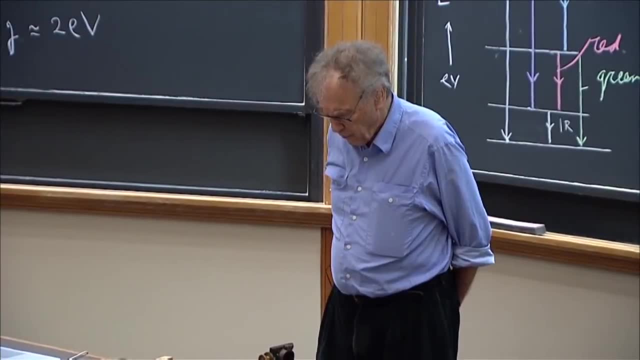 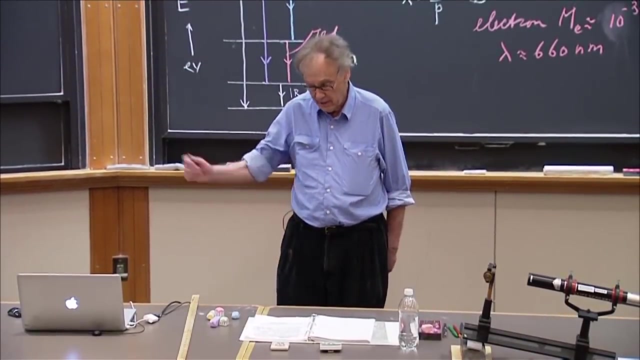 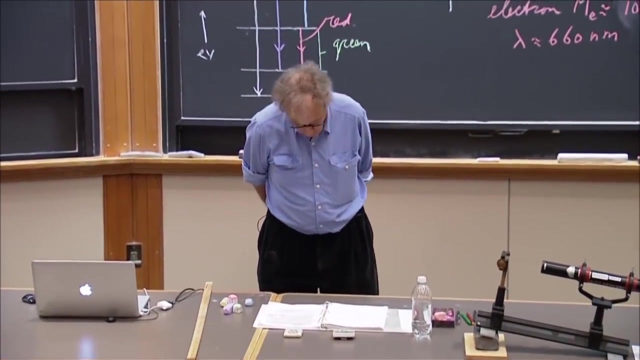 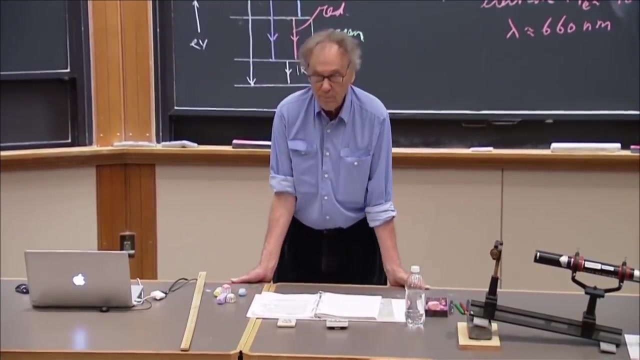 of the Heisenberg's uncertainty principle is a profound, non-classic idea and it's very hard for any one of us, including myself, to comprehend. Why shouldn't you be able to determine some position in Heisenberg's uncertainty principle? I want to repeat. 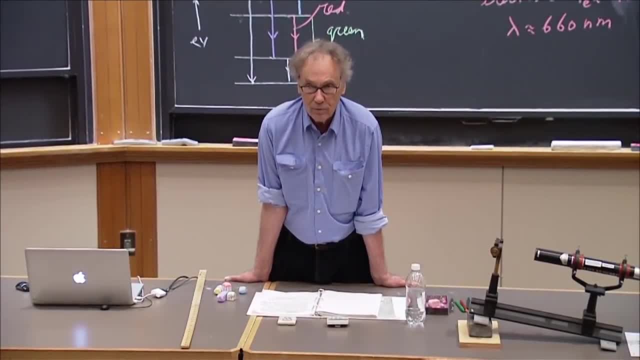 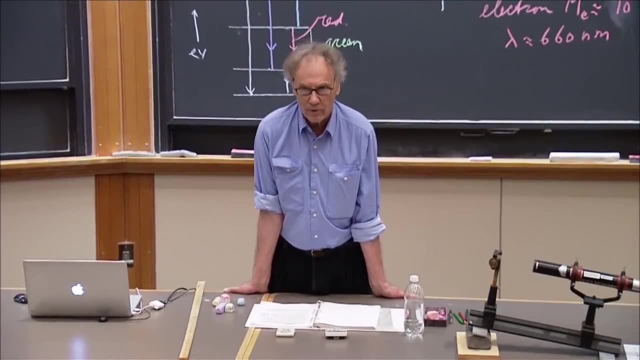 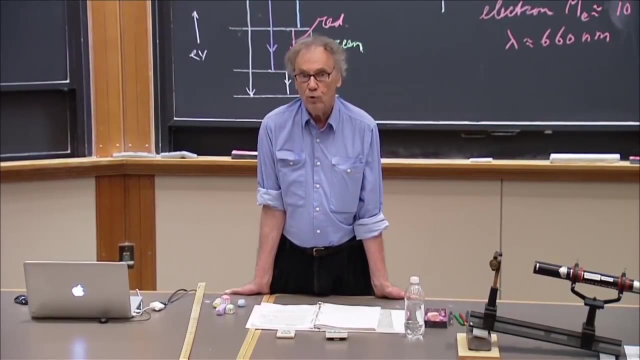 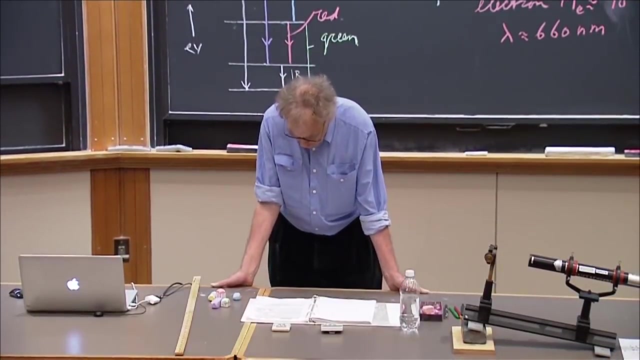 it to you, because the part that is coming now is the most difficult for you, because I'm actually going to write the equation Heisenberg's uncertainty principle- on the blackboard and I know it's going to take some time at the very end to understand it. 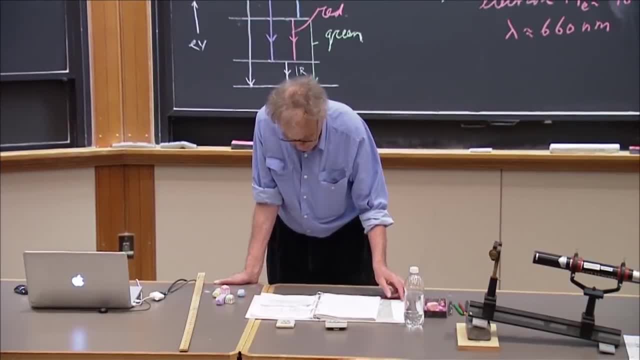 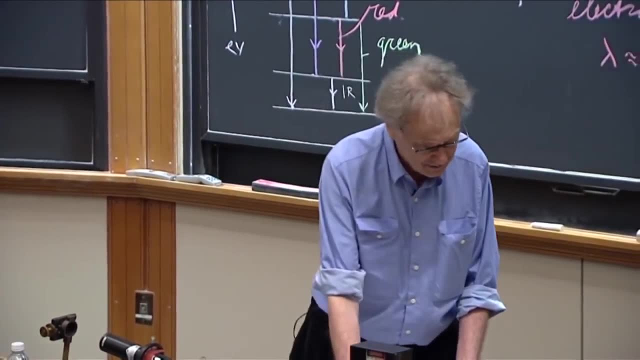 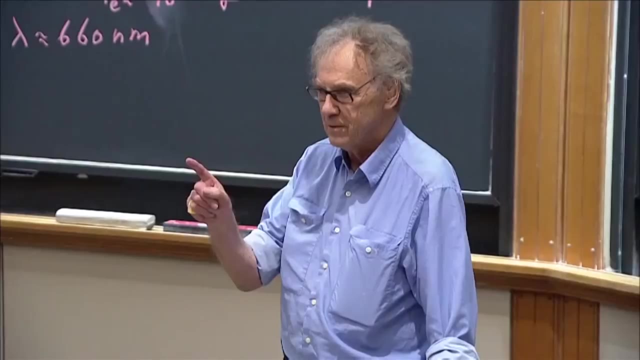 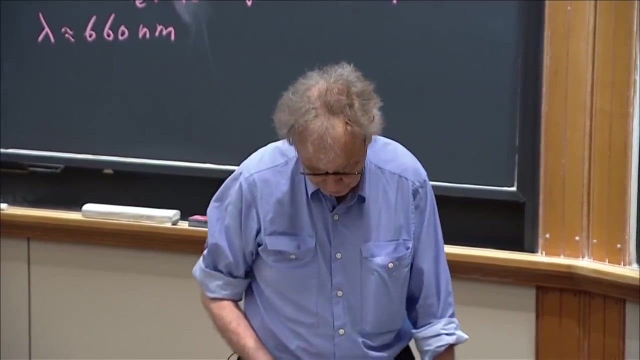 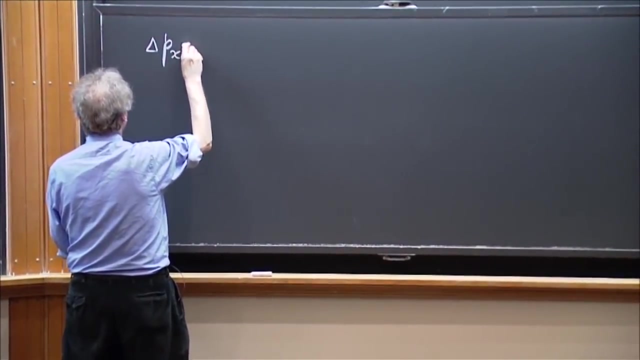 So I want to repeat it: the very concept of exact position of an object and its exact momentum together have no meaning in nature. And let me now write down Heisenberg's uncertainty principle, so that it may come to life: Delta p, x multiplied, this dot means: 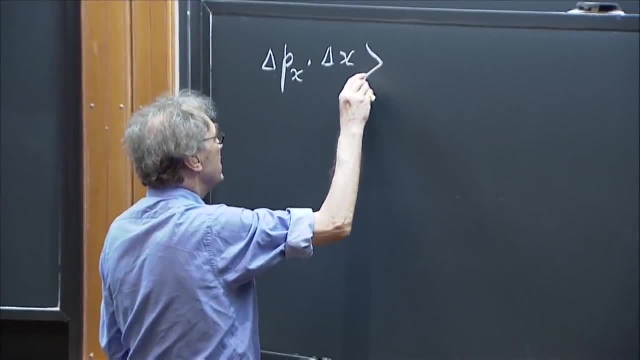 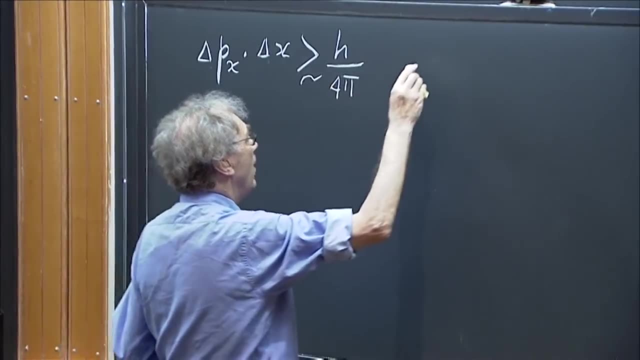 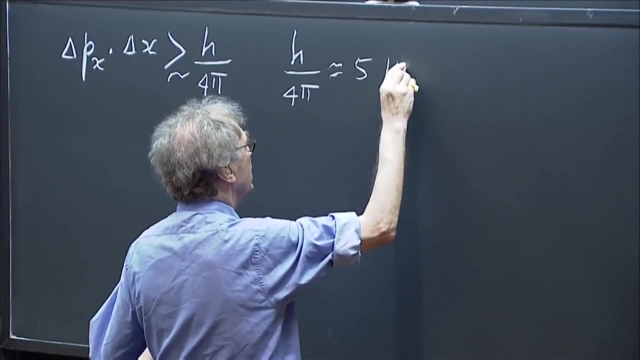 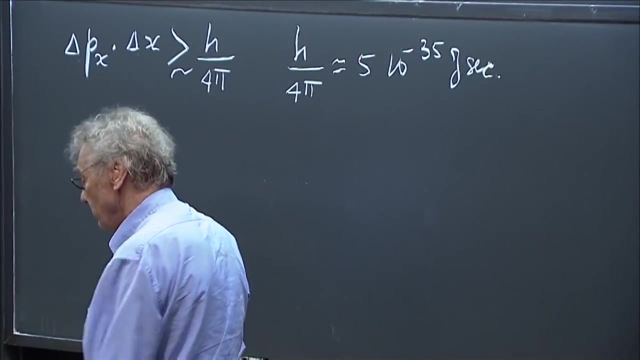 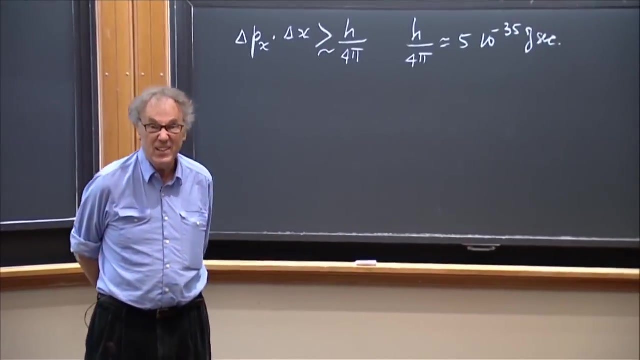 multiplied by delta, x is larger than or approximately equal to h divided by four pi. and just to remember to remind you, h divided by four pi is minus thirty five joule seconds. What does that mean? Well, let's first talk about the delta, The capital D. 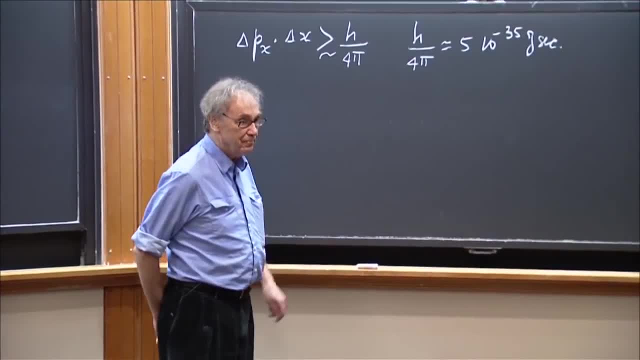 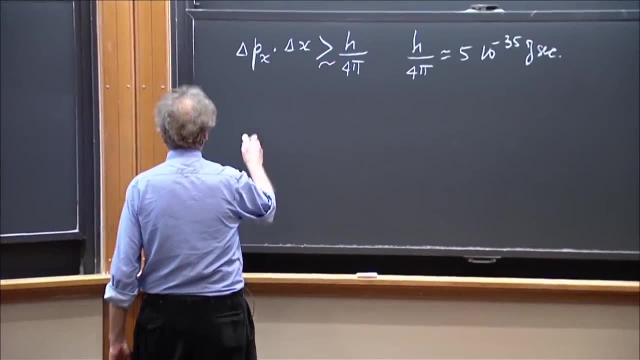 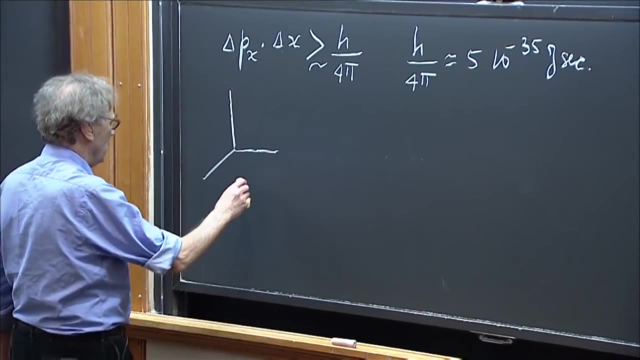 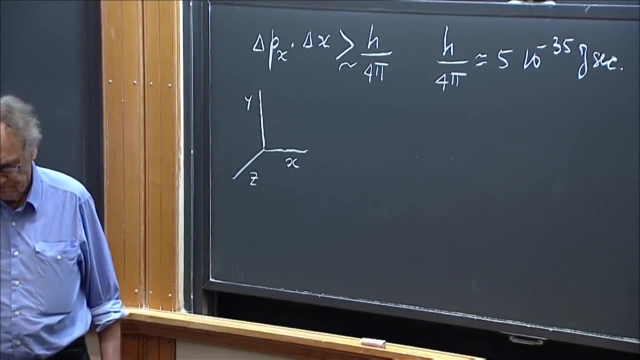 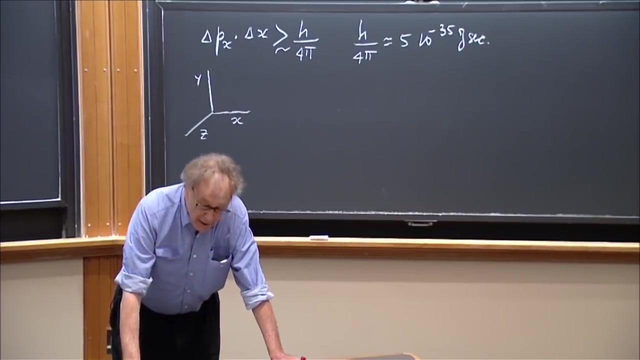 in Greek is this symbol delta. We use that very often in mathematics and in physics. We live in a three dimensional world. This could be x, this could be y, this could be z. Assume now that the particle is somewhere on the x axis. 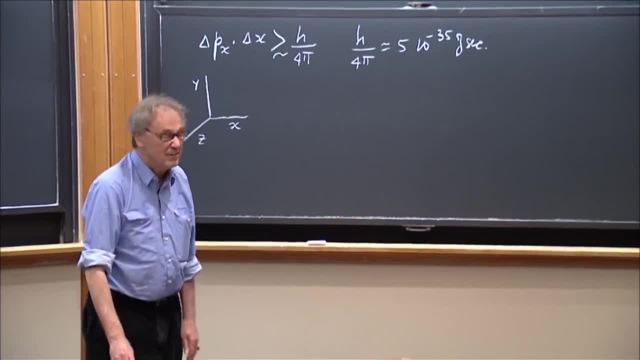 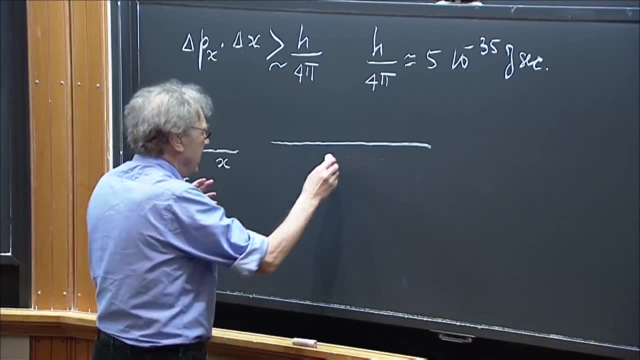 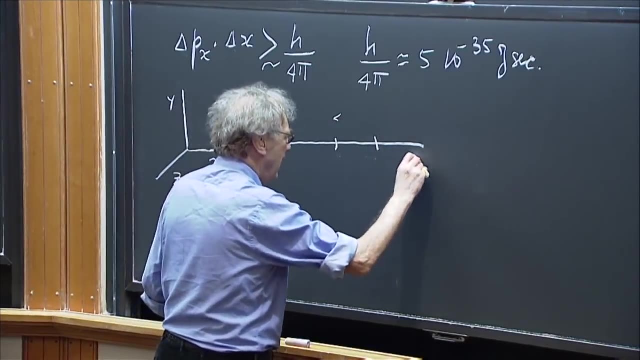 But I do not know precisely where it is. So here is this x axis. I don't know precisely where it is. It is somewhere larger than x one and somewhere lower than x two. So this is the x axis. Then we call this often. 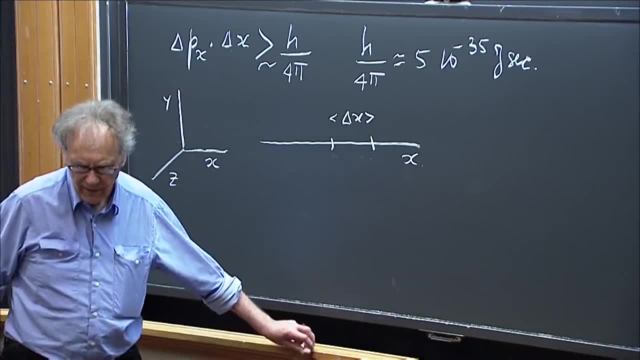 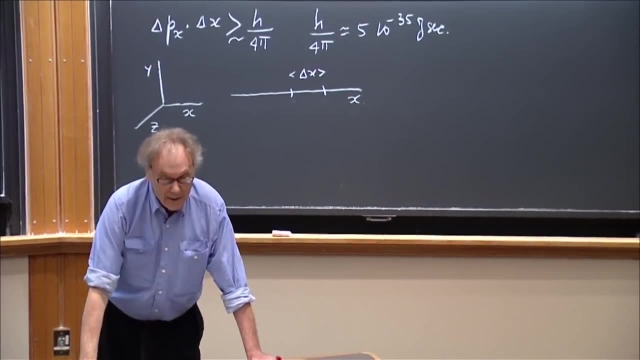 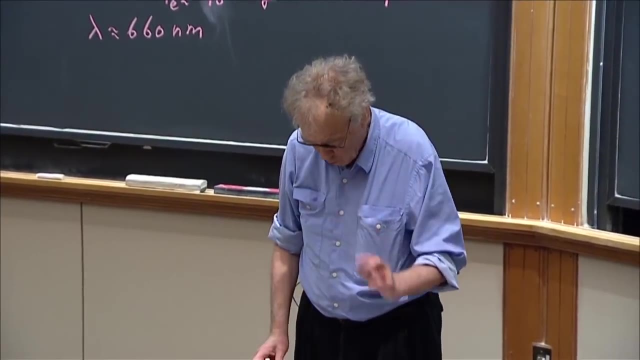 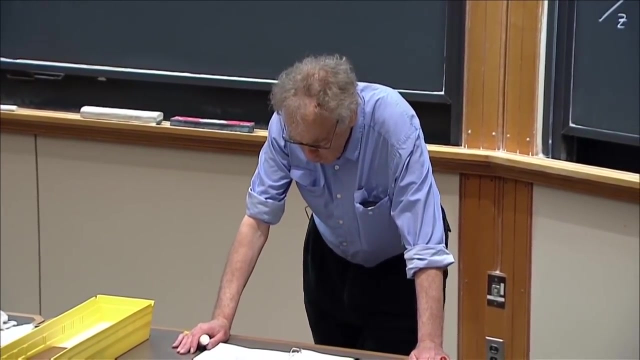 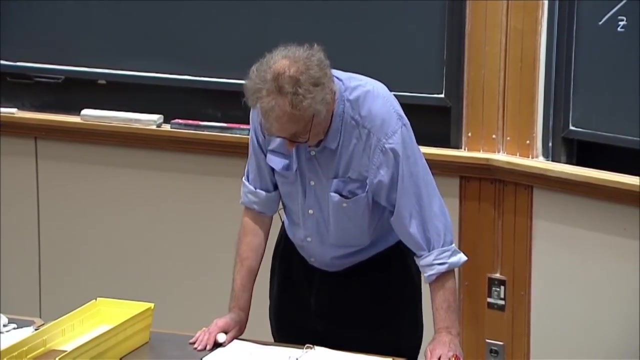 delta x. So the delta x indicates our lack of knowledge where exactly the particle is. It is an uncertainty in the position x. The same is true for the momentum p. Delta p indicates the uncertainty in our knowledge of the momentum- Heisenberg's uncertainty. 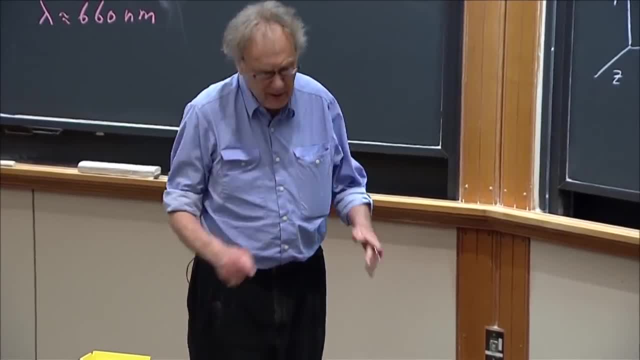 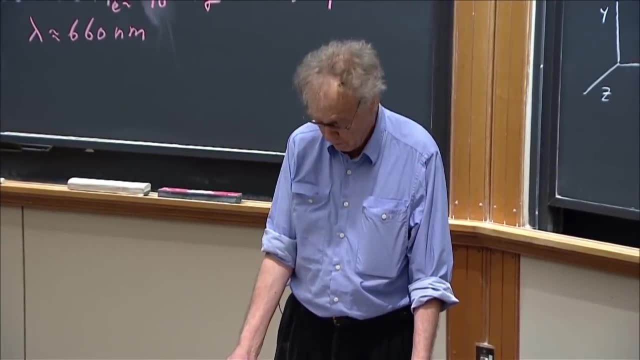 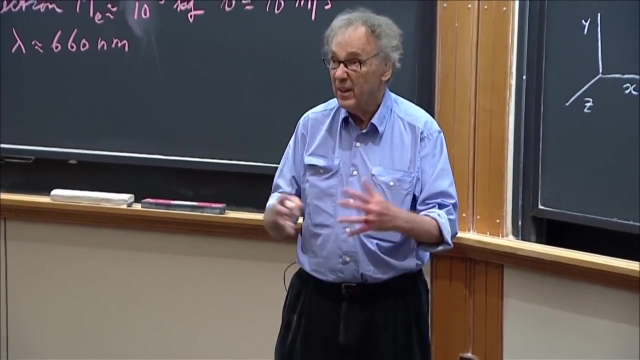 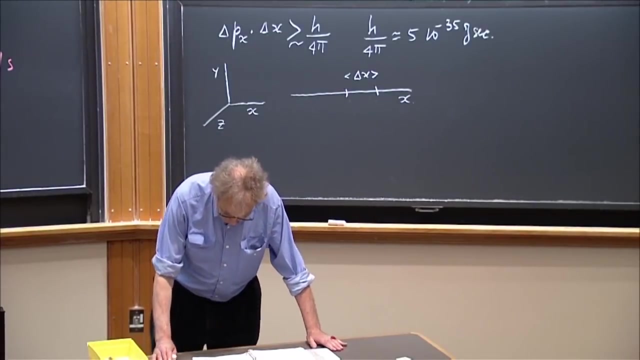 principle tells us that if delta x is very small, in other words the particle is contained in a very small range and is very large, then the uncertainty in the momentum is very small. So then we can know p very accurately. But it is not possible, according to Heisenberg. 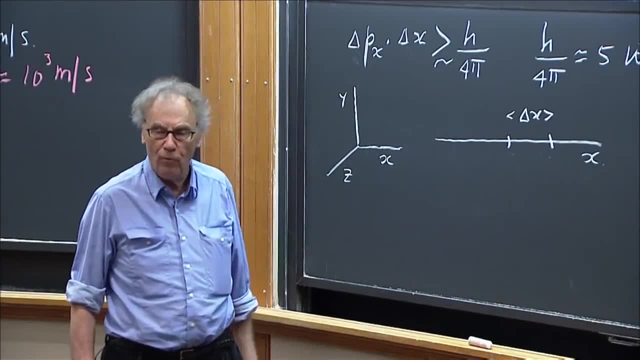 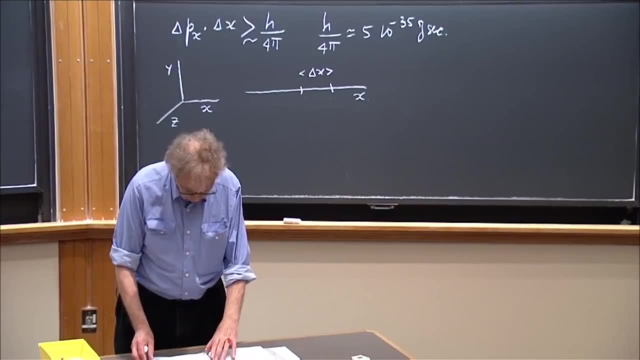 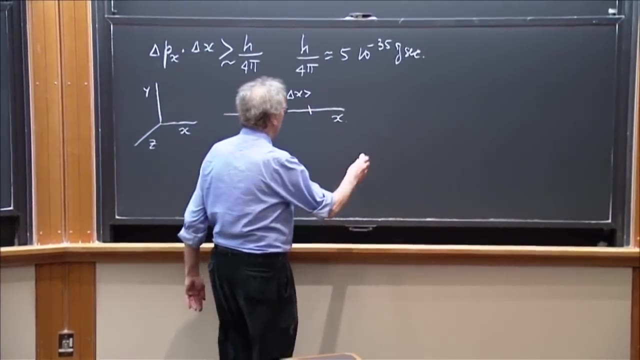 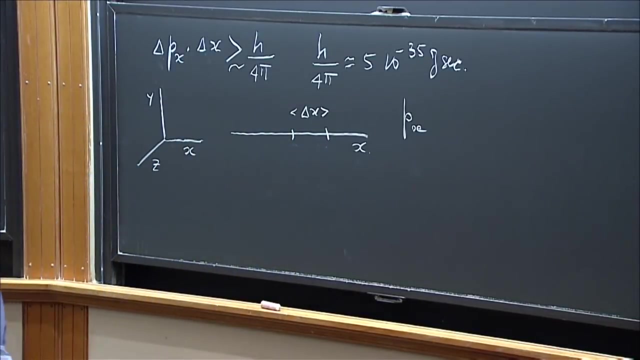 to get a very small value for delta p and at the same time, get a very small value for delta x. That is not possible. Before we can get into action, I have to explain to you why there is an x here and why there is a delta x there. 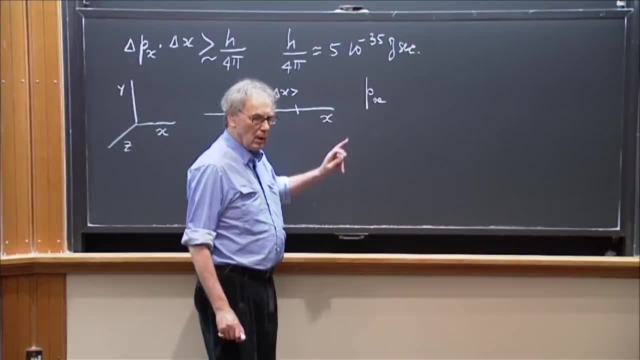 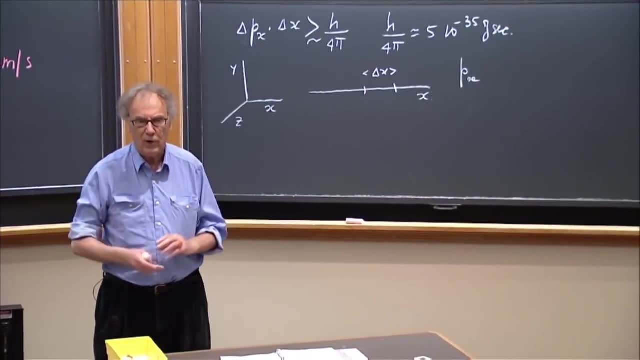 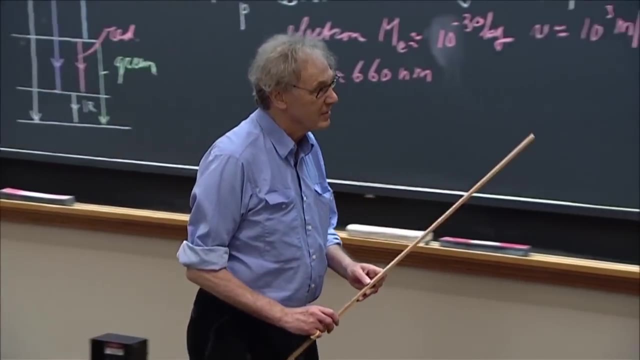 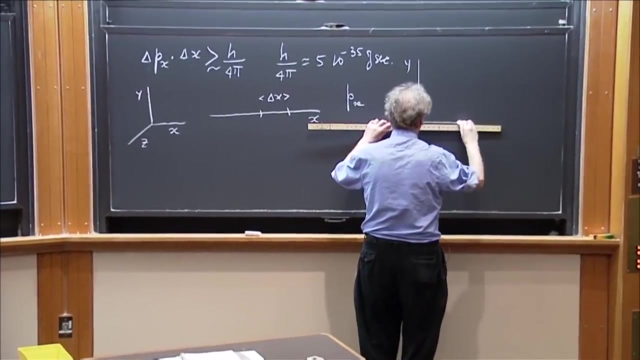 Momentum is what we call a vector. It means it has a magnitude and it has a direction, the same as velocity. I will show you. you are going by your car and you are driving. I call this the y direction, I call this the x direction and 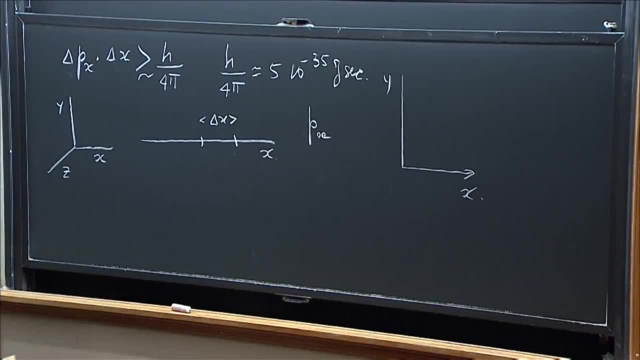 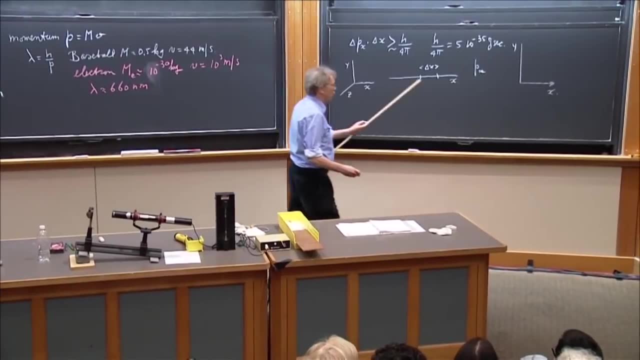 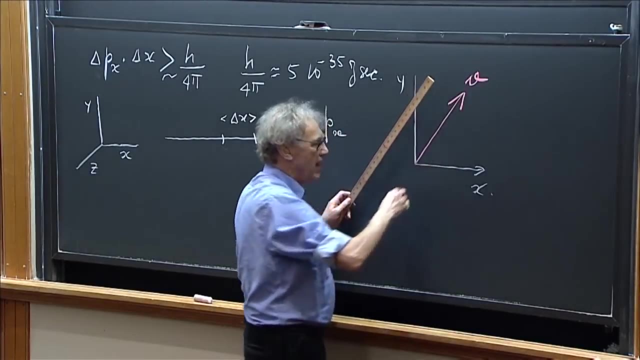 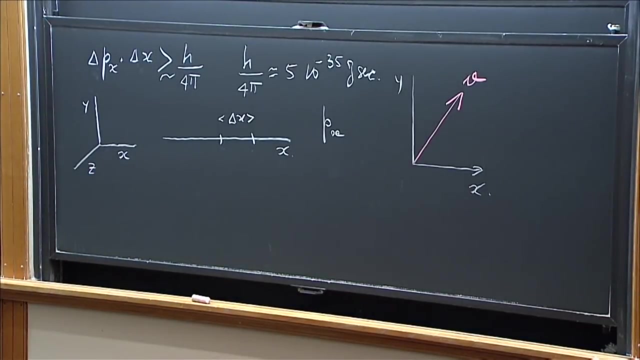 this may be north, that may be east, that is irrelevant, and your car has a certain velocity, and the velocity is neither in the x direction. the length of this arrow indicates, then the speed, and the direction of the arrow indicates the direction that you are going, and that is why this is. 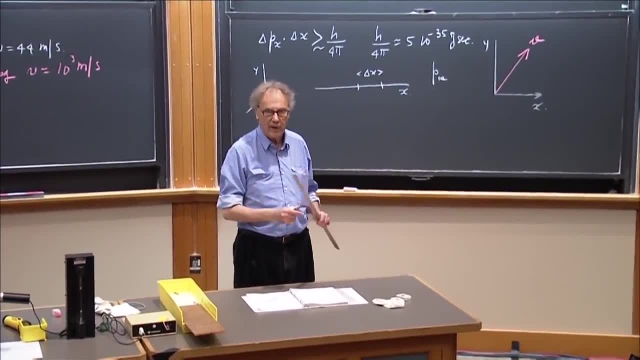 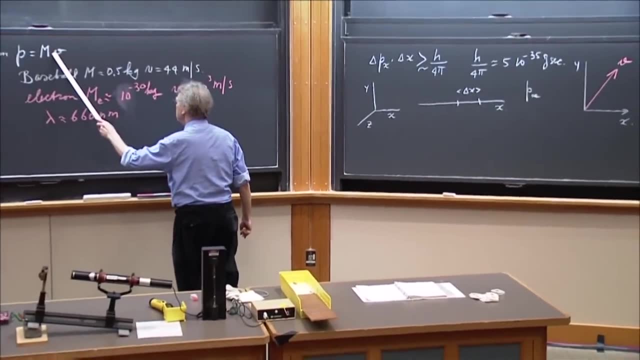 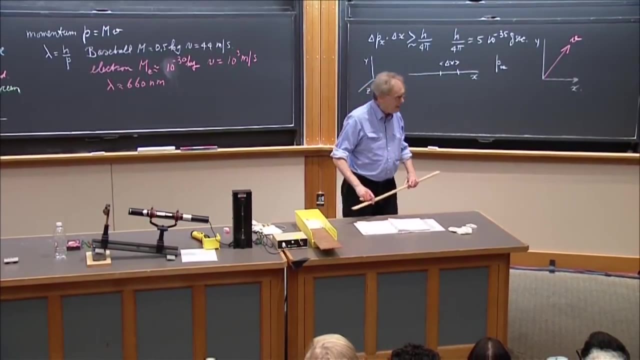 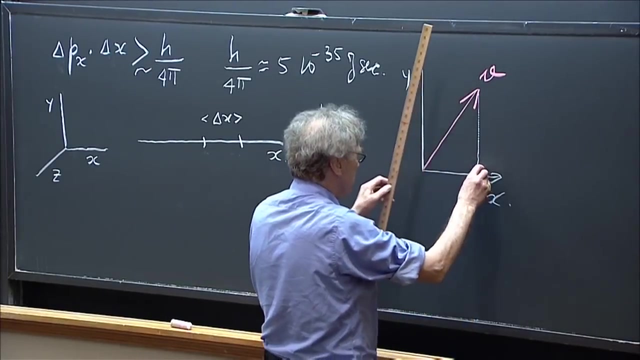 called a vector. you have to know two things: you have to know the magnitude and you have to know the direction and momentum. p is the product of m and v. if we take v and we project it onto x, so this angle is 90 degrees, then this vector 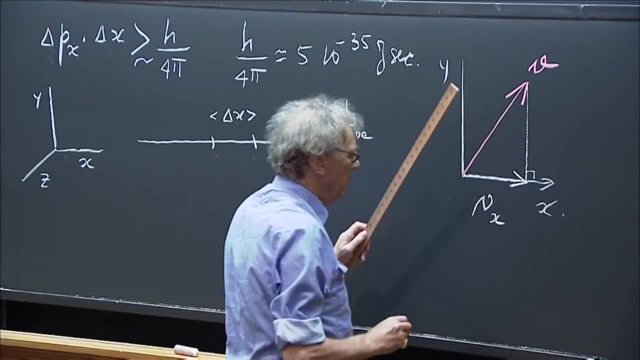 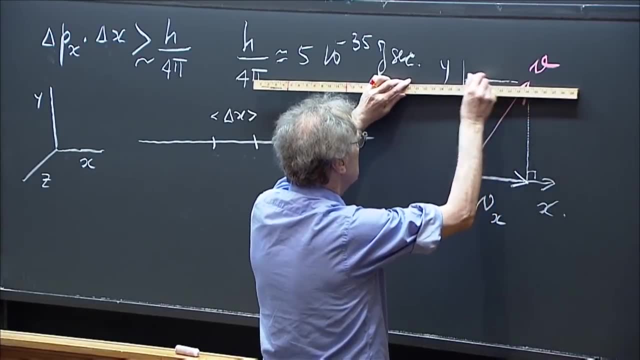 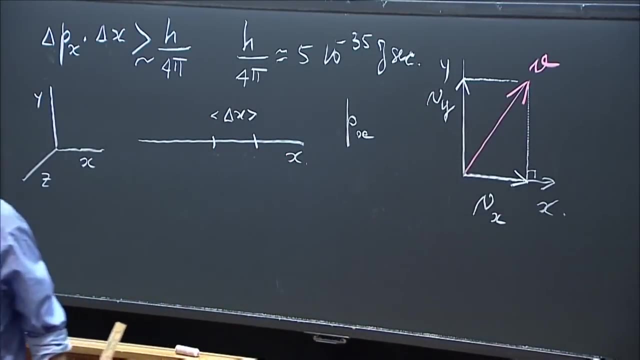 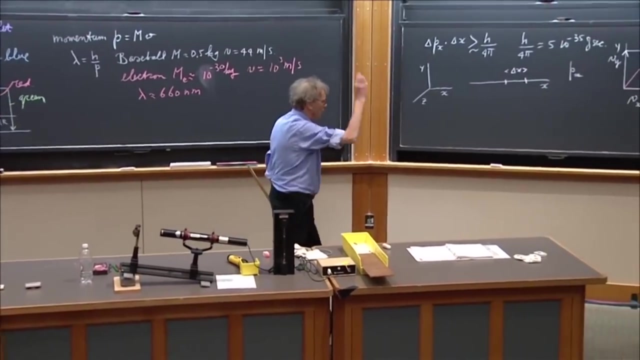 is called v of x. it is the x component of the velocity vector v, and if I project it here, then this vector is v of y, the y component of this vector, and so in this picture I could draw the momentum vector in the x direction. I don't have to put in the general 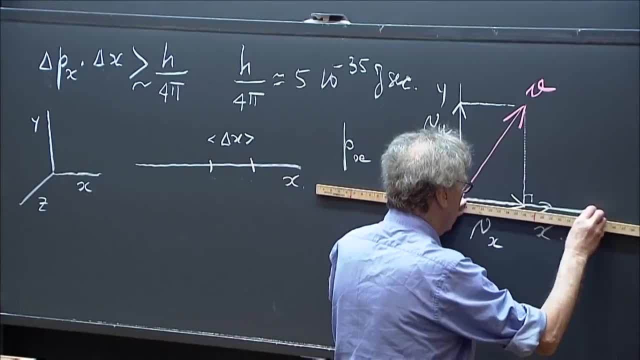 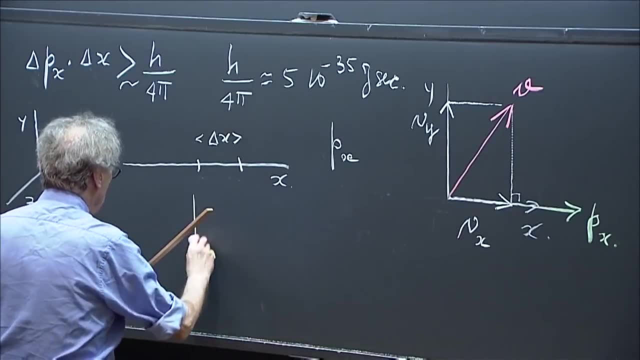 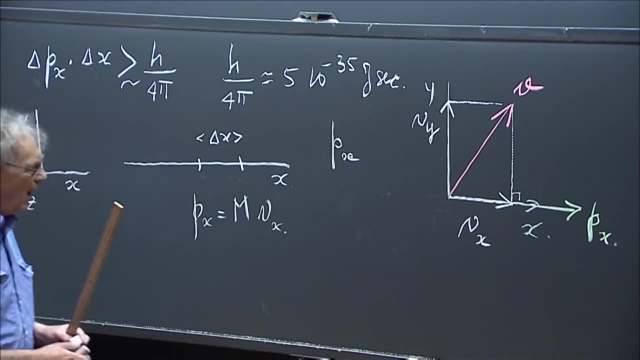 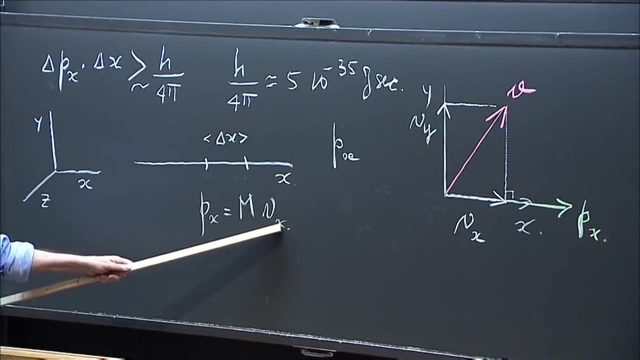 momentum, but this then, for instance, could be p of x, and so I could write down then that p of x equals m times v of x. that is the only meaning that I have here, and I can change the x here to a y, and I can change this to a y. 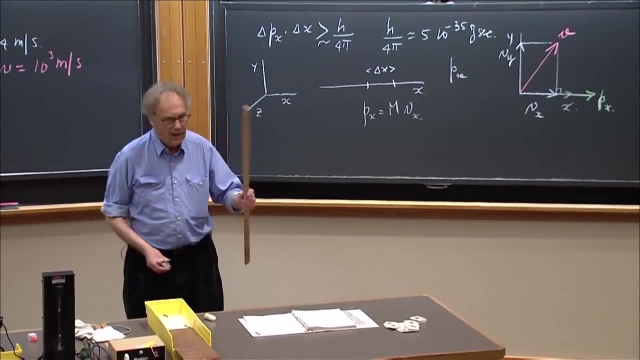 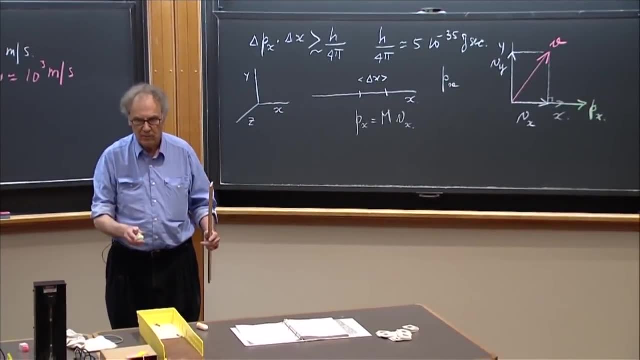 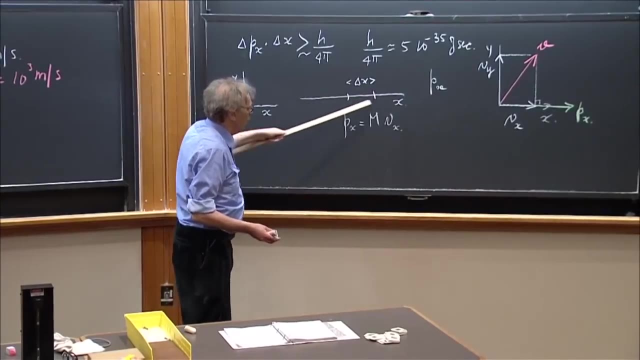 and this to a y, and uncertainty principle again holds in the y direction. I can change this to a z and I can change this to a z. then the uncertainty principle also holds in the z direction. but it is possible that if the particle is only moving in the x direction, 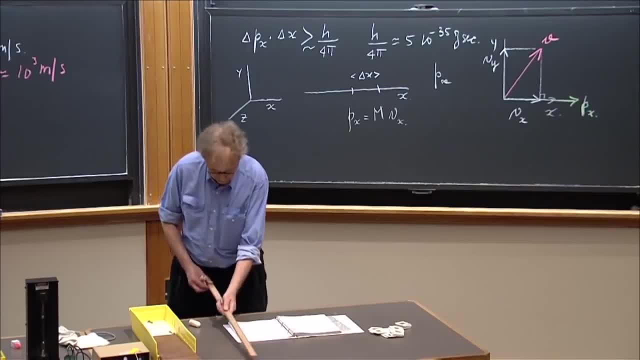 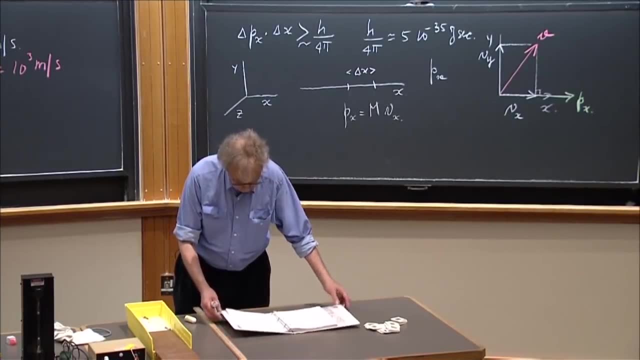 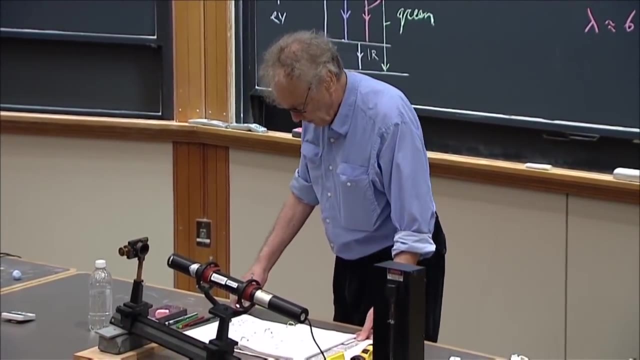 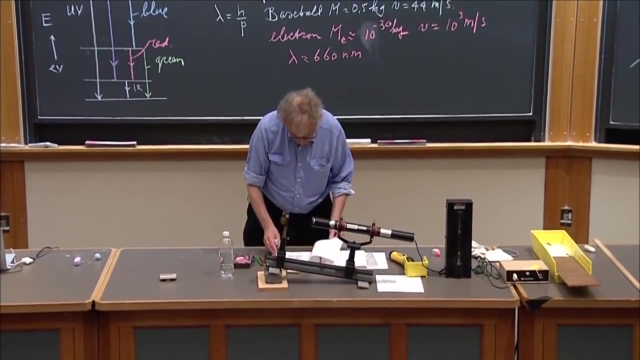 that the particles in the z direction are of no interest. but in principle you can write down the uncertainty principle in three independent equations. there is a wonderful book which is called Mr Tompkins in Wonderland and it is a professor who appears in the dreams of Mr Tompkins. 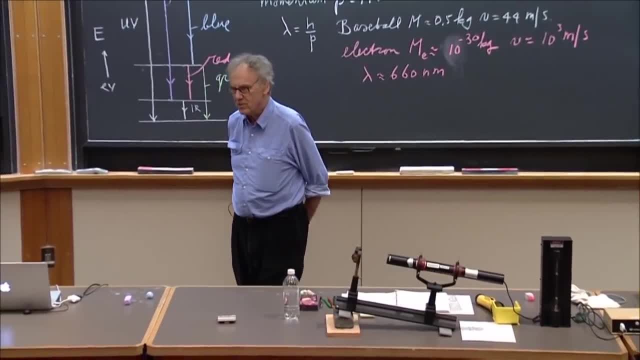 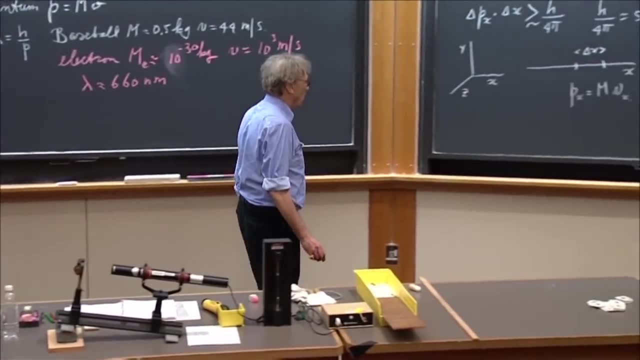 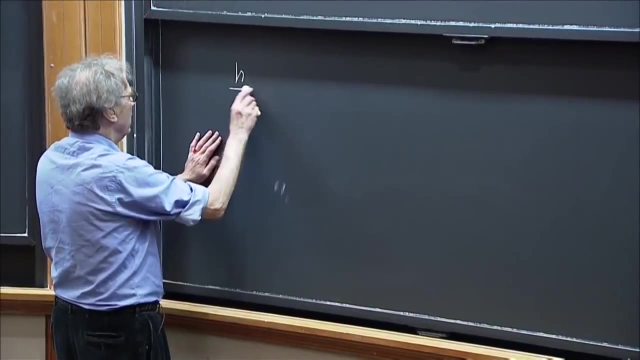 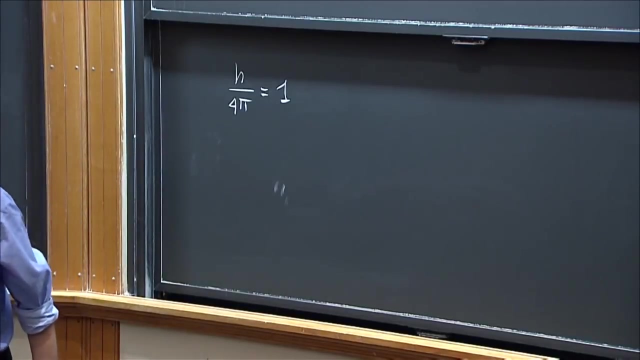 and this professor is teaching quantum mechanics and in one of the dreams he says to Mr Tompkins: just assume that h divided by four, pi is one. and he takes a billiard ball, one billiard ball, and the billiard ball has a mass of one. 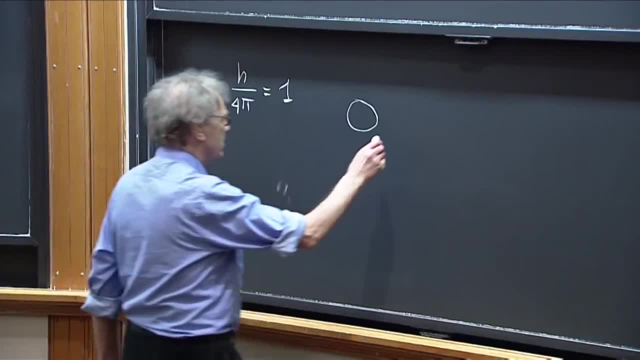 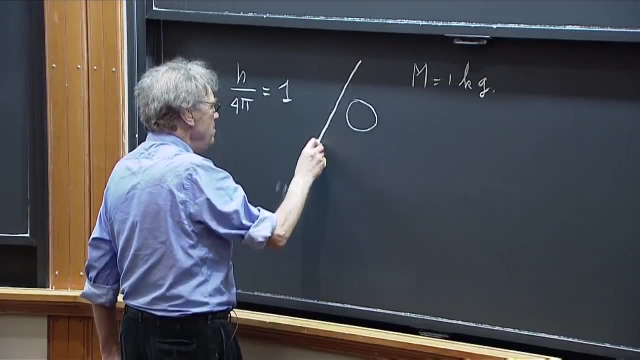 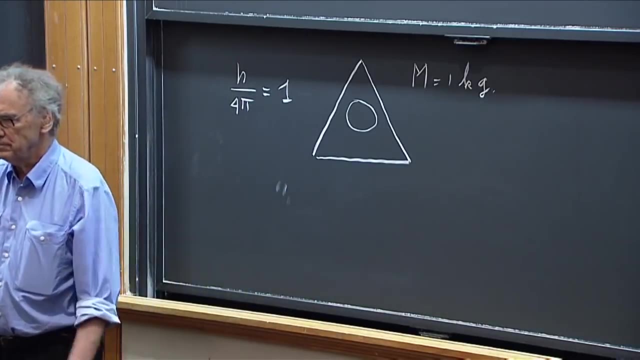 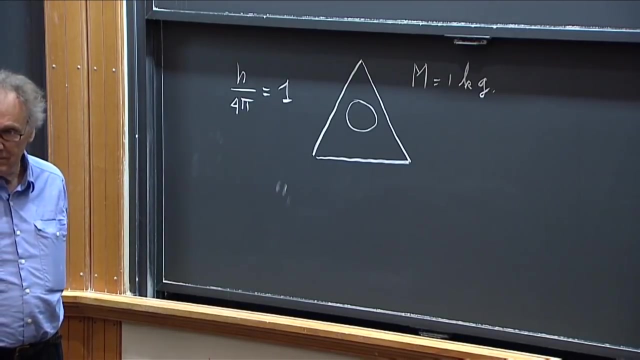 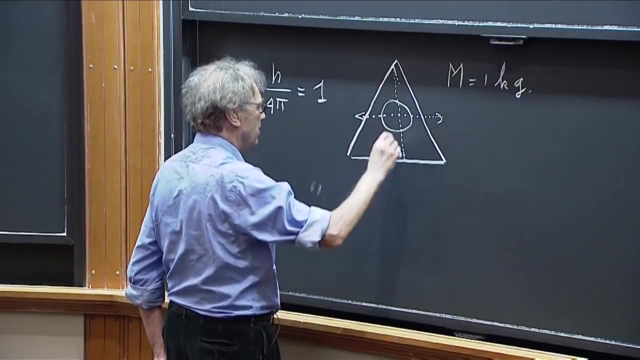 kilogram. so here is a mass which is one kilogram. and then in the dream he puts around the billiard ball a wooden triangle. now the billiard ball is now constrained. it is constrained in the x direction, it is also called. it is also constrained in the y direction. 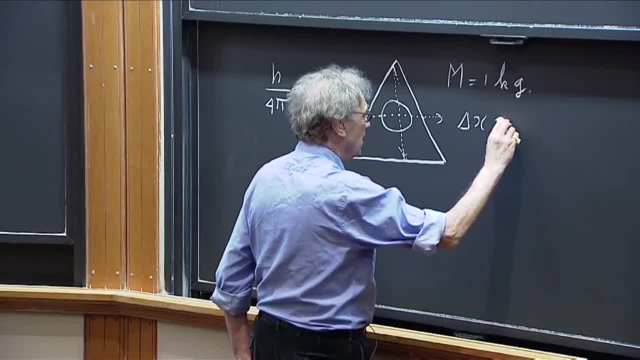 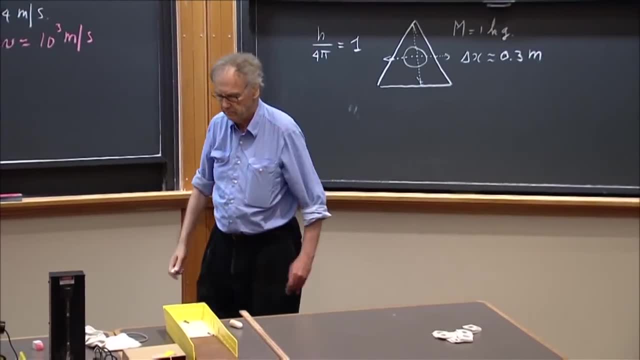 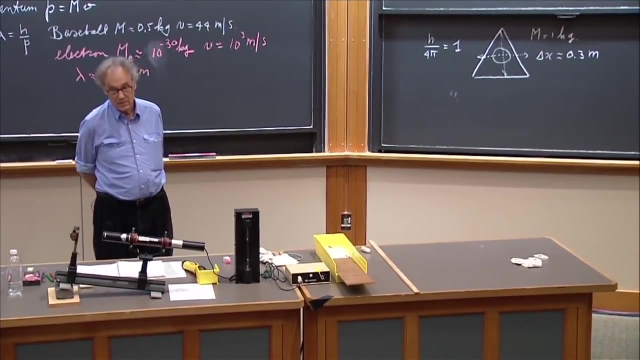 and the dimension here is roughly, so we would call that delta x is roughly 0.3 meters, in other words 30 centimeters. that's about how big these are. so the professor says we can now calculate what delta p is with the uncertainty principle. that's very easy. 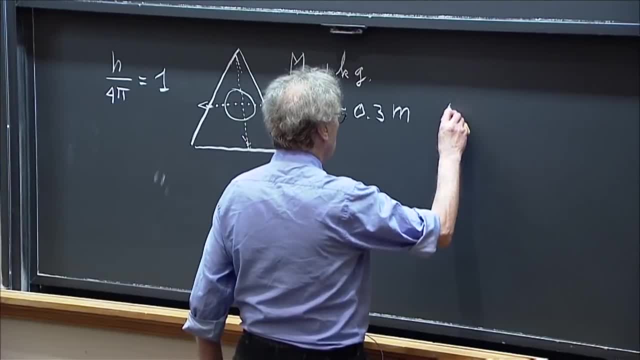 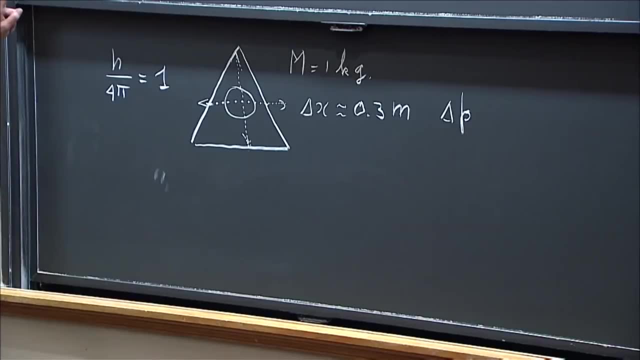 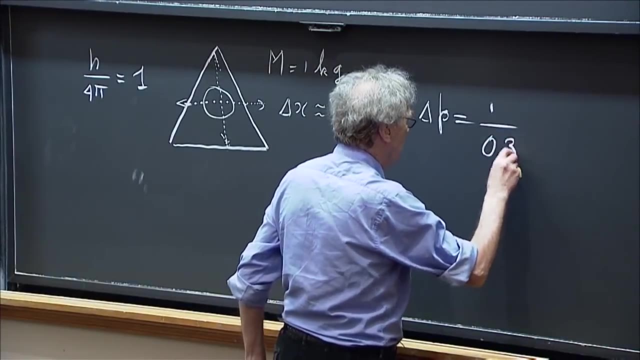 delta p in the x direction is about the same as in the y direction, so I will just use delta p and ignore the x and the y. so delta p is one. remember he calls this one divided by 0.3, which is the 0.3 meters. 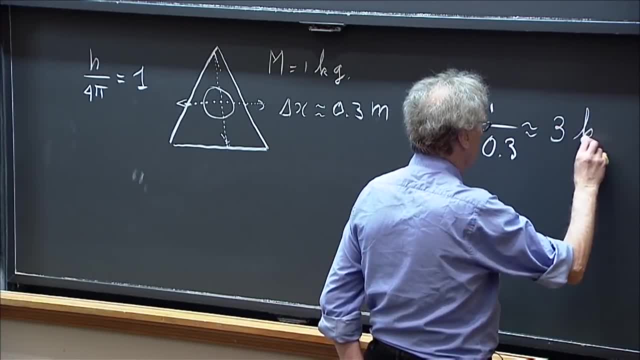 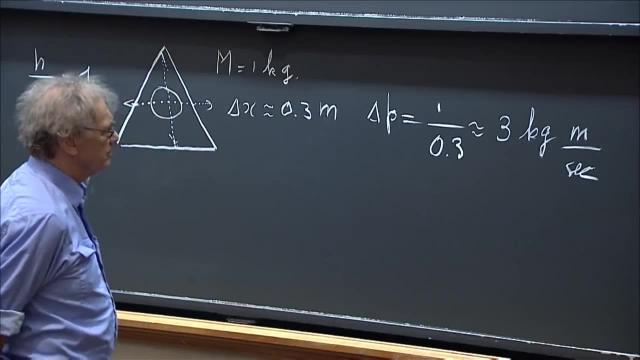 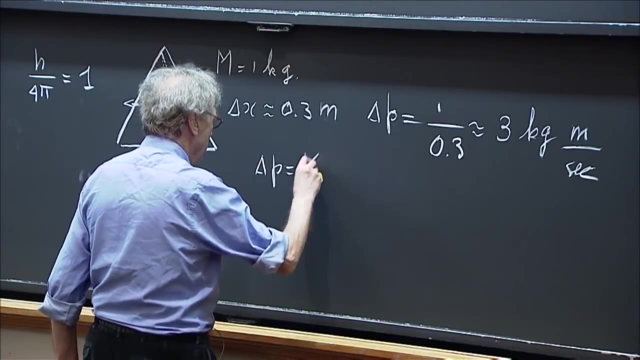 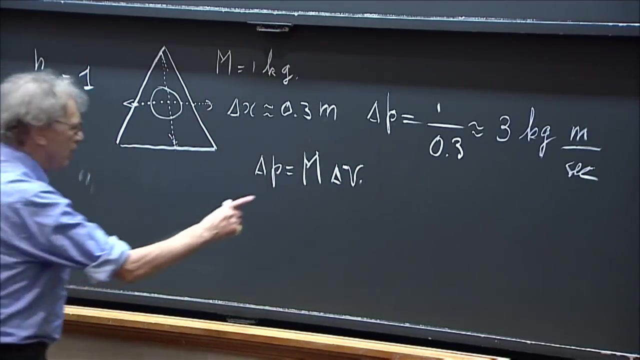 and so delta p is very roughly three, and this is a nasty unit which is one kilogram meters per second. since the mass is one kilogram, delta p is m times delta v. that follows from the definition of momentum, and since m is one kilogram, it means that delta v. 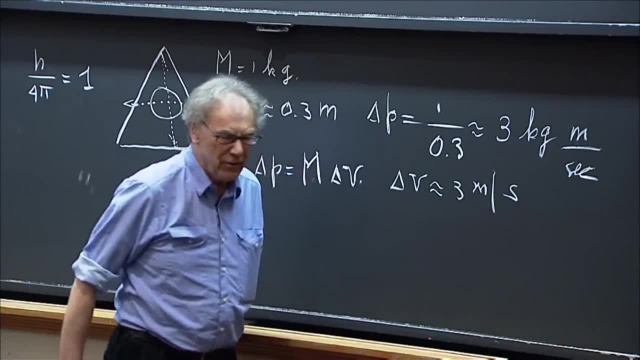 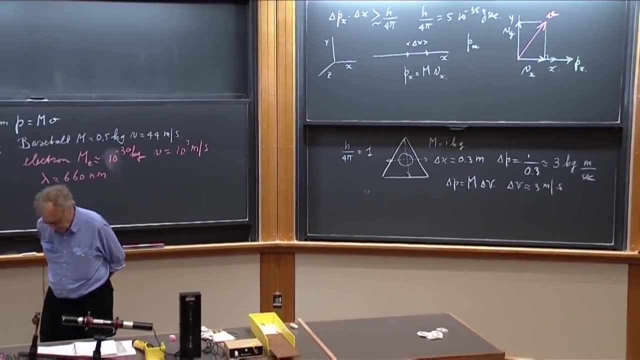 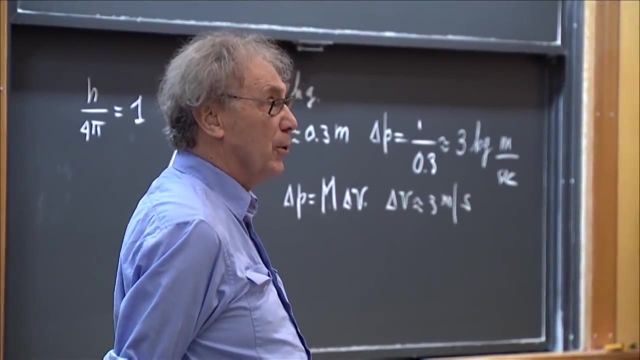 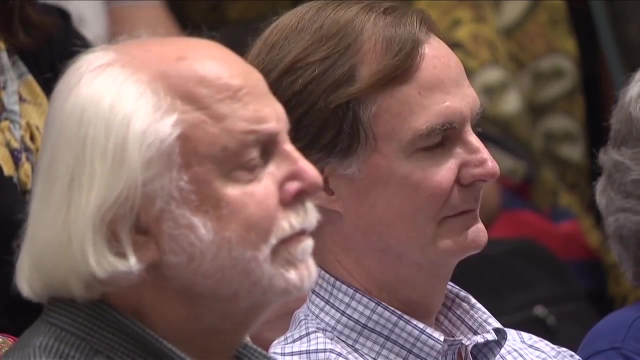 is roughly three meters per second. three meters per second means now must adopt a speed very uncertain of the order of three meters per second, which is ten kilometers per hour. so the moment that the professor puts the triangle over there, they won't see one billiard ball anymore. 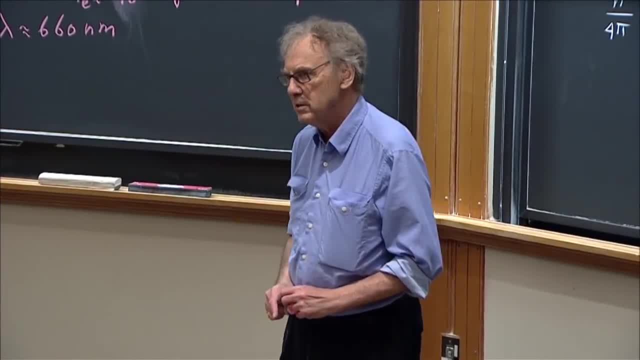 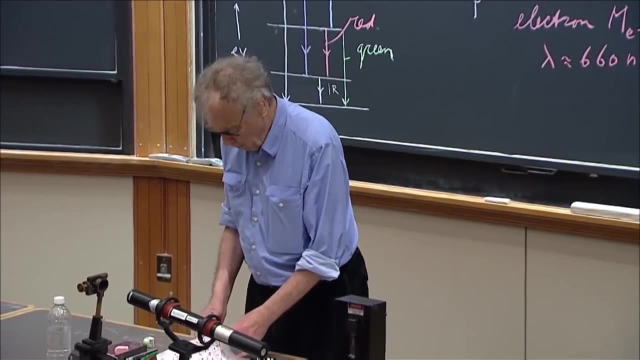 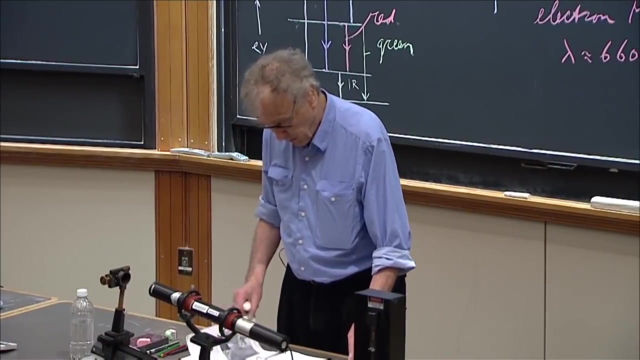 but they see the billiard ball going in all wild directions. it's beginning to move. that is the result of Heisenberg's uncertainty principle, because the billiard ball is now drained in its position and the price you pay for that is that delta p becomes very large. 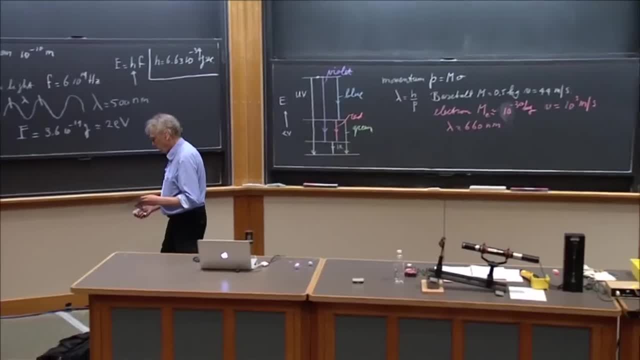 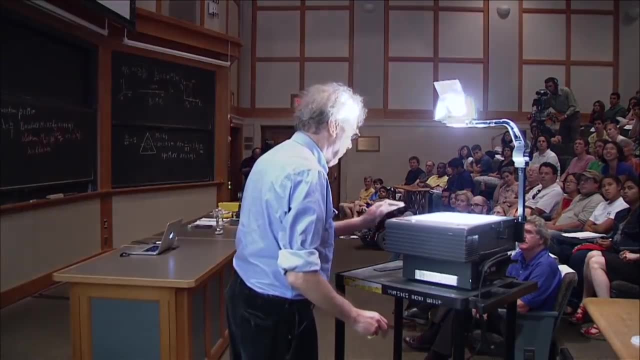 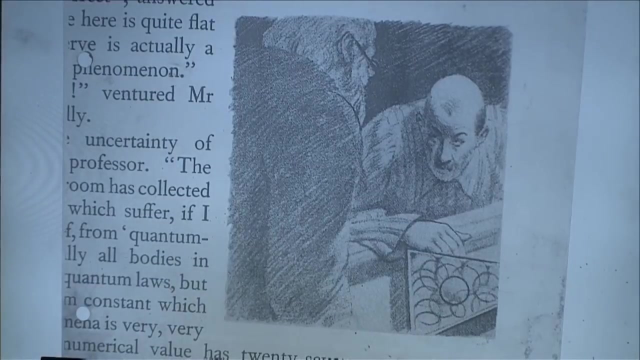 and the object starts to move. and I will show you here the picture of the dream about the billiard ball whereby h divided by four pi was arbitrarily set to be one. all professors have beards, as you know. the professor also has a beard. Tompkins is always in pyjamas. 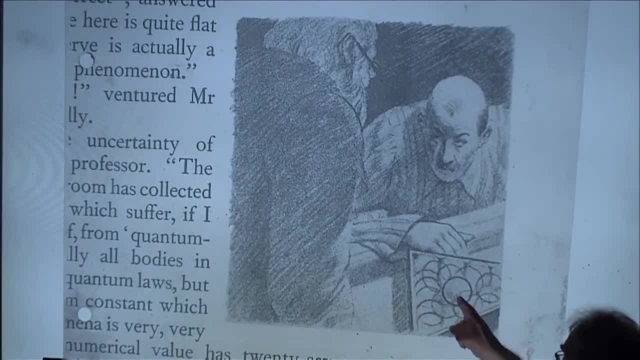 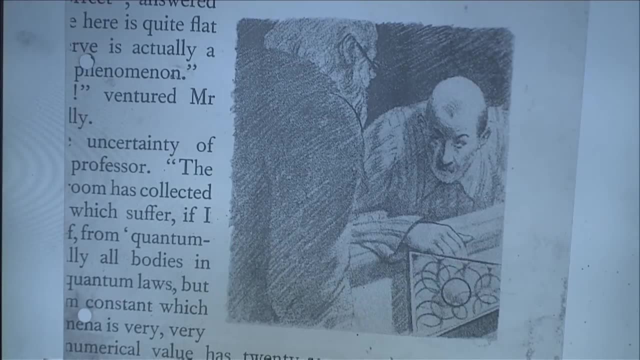 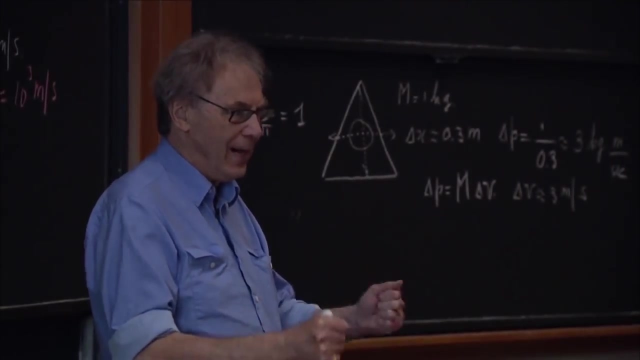 because he's in a dream and you see here that this one billiard ball is now going like crazy because of Heisenberg's uncertainty principle it's contained. delta x is small, the price you pay. then, if delta x is small, delta p must be large. 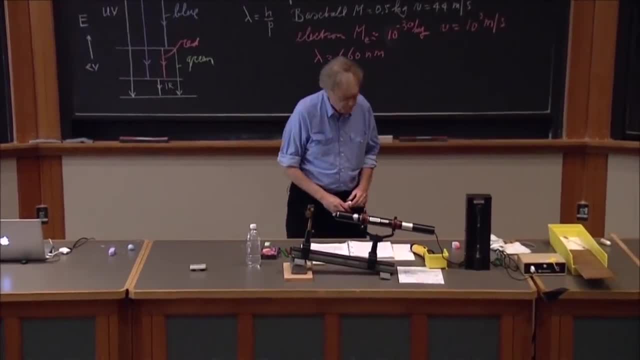 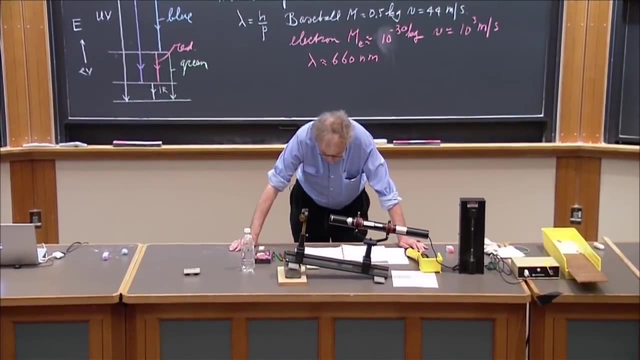 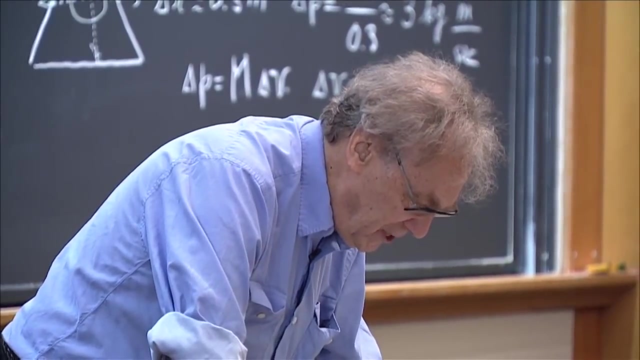 and the thing begins to move from the book, if you give me the lights again. the book says: as soon as the ball was placed in the enclosure, the whole inside of the triangle became filled up with the glittering of ivory. you see, said the professor, I defined the position of the ball. 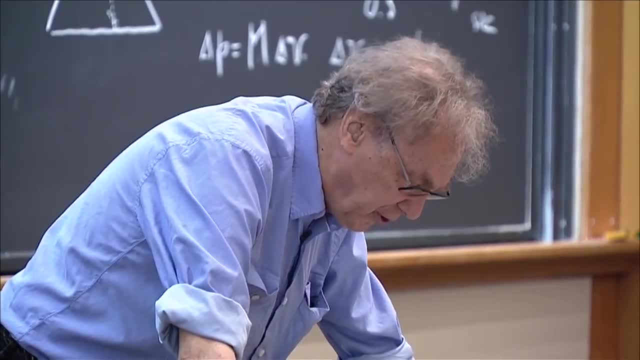 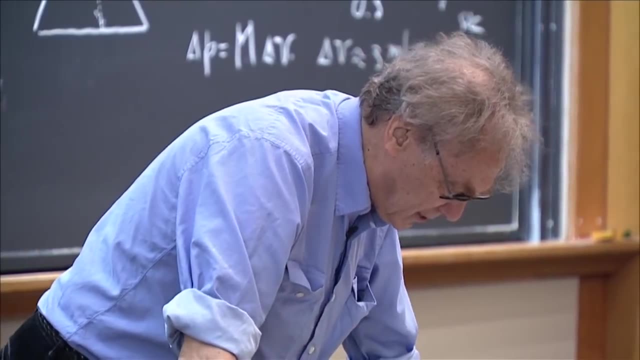 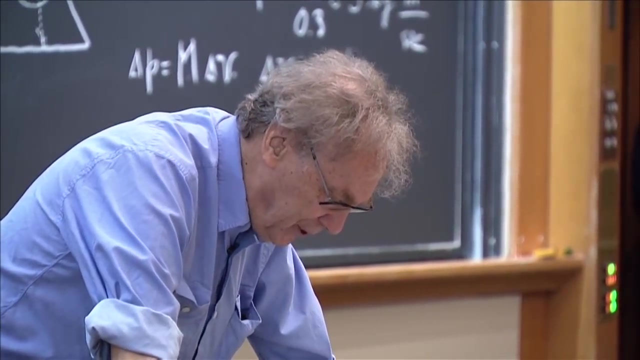 to the extent of the dimension of the triangle. this results in considerable uncertainty in velocity and the boundary. Mr Tompkins says: but can't you stop it? oh, said the professor, it's physically impossible. anybody in an enclosed space possesses a certain motion, and we physicists call it. 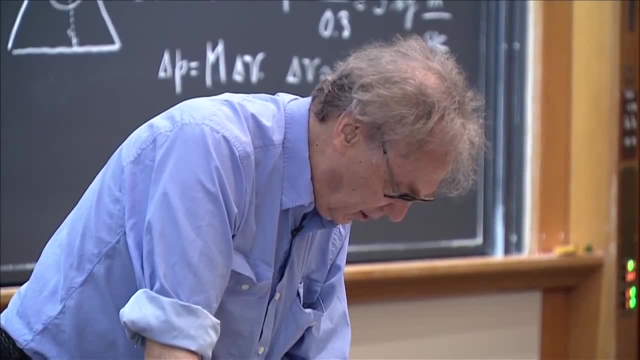 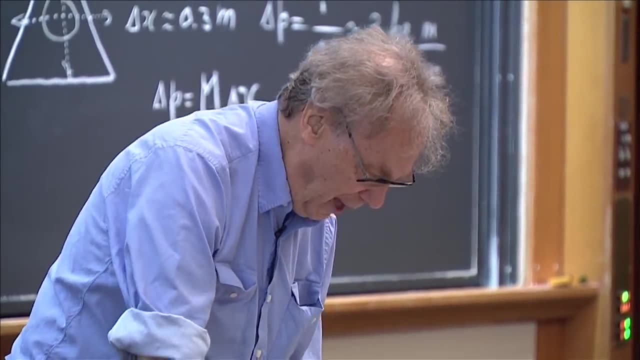 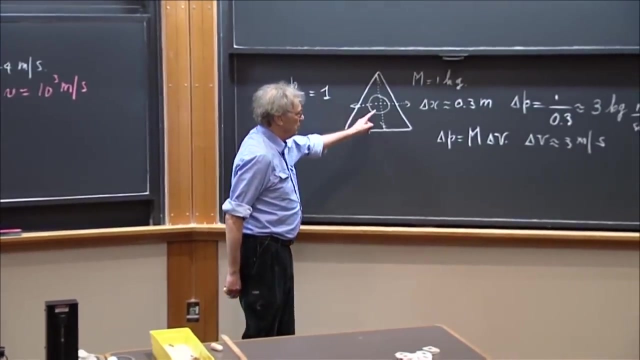 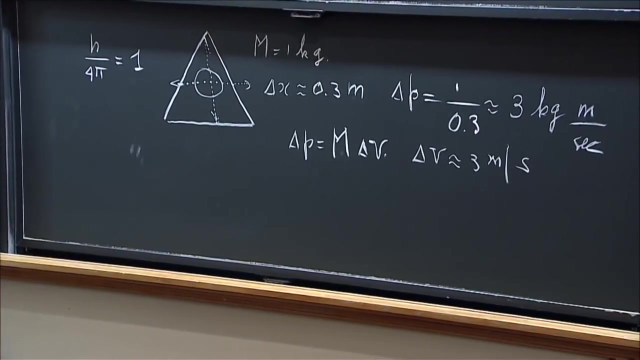 zero point motion, such as, for instance, the motion of electrons in any atom. now I'm going to the real world. I use the billiard ball from the dream, but I'm not going to take h divided by four, pi is one. I'm going to take the real value. 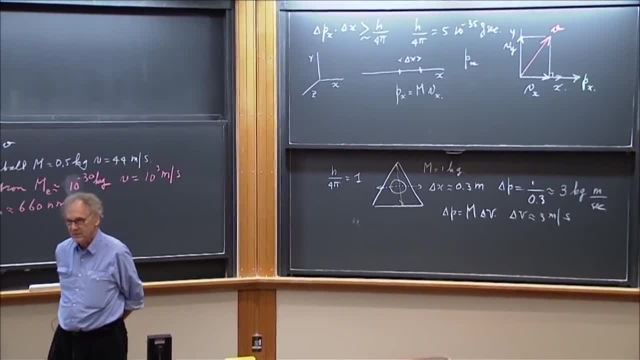 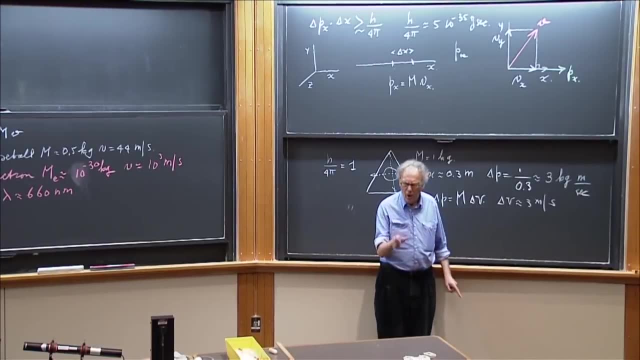 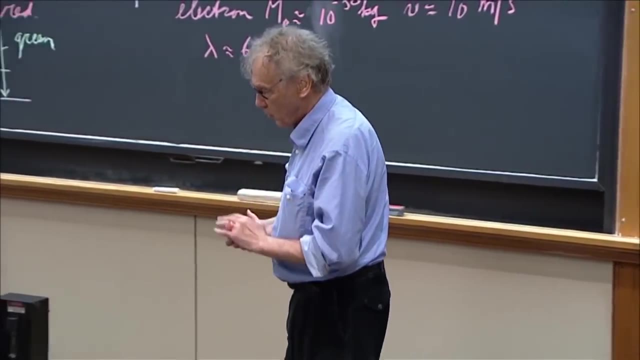 five times ten to the minus thirty five, and I go through the same calculation and now I want to know what the velocity is of that billiard ball- something I could do at home- and I make the calculation and the result is that in ten billion years the billiard ball would have moved. 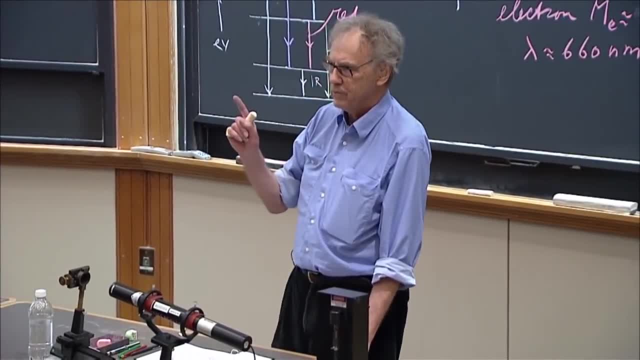 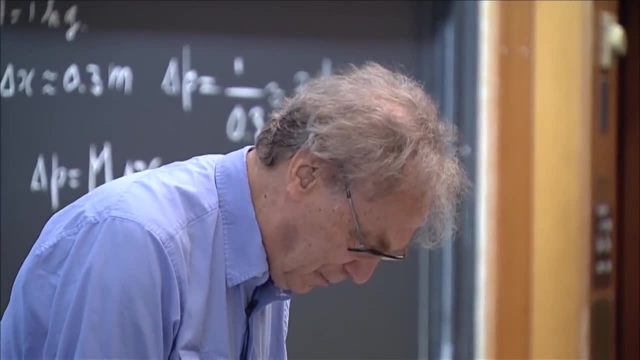 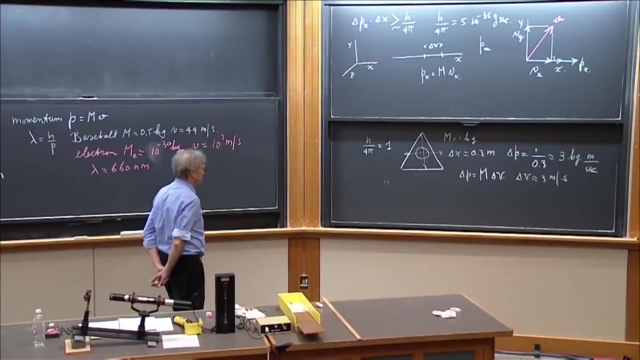 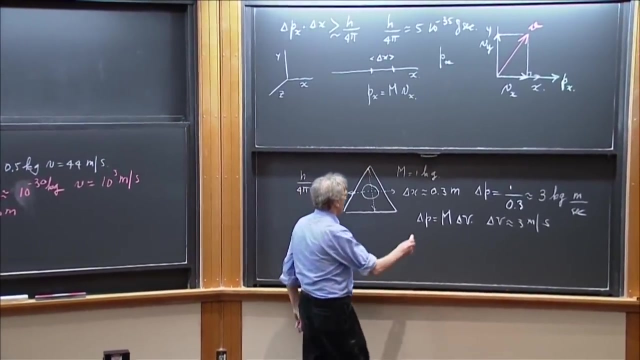 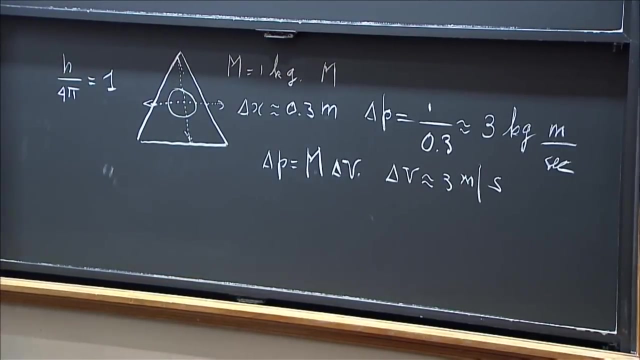 a distance, one twentieth the size of a proton, which is meaningless. quantum mechanics has no effect on our daily experiences. now we go to hydrogen, now we take the hydrogen atom, and the hydrogen atom has the dimension that we already know: ten to the minus ten meters. and in the hydrogen atom, 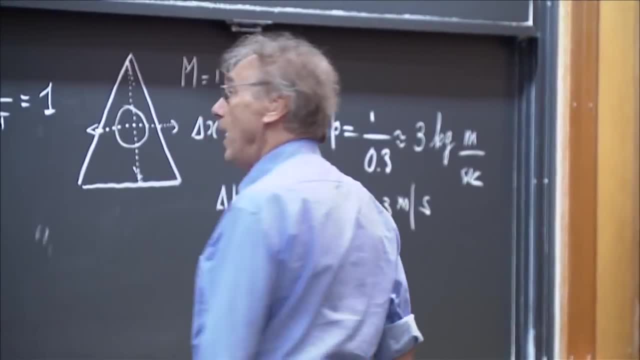 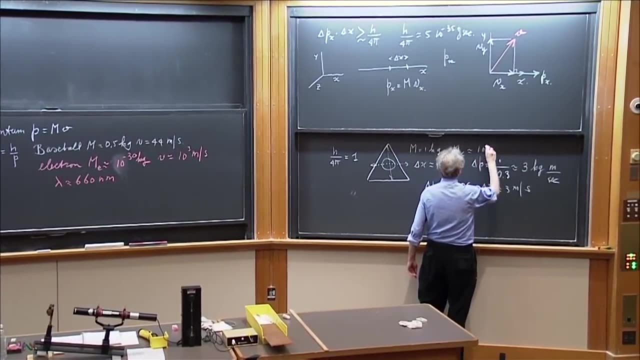 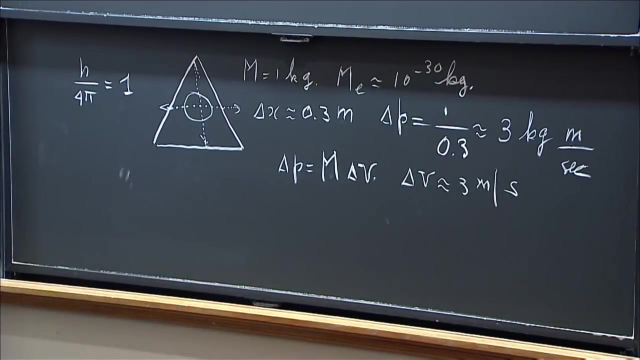 is one electron and the electron. I also wrote down the mass of the electron somewhere. if it's lost I will write it again. it's ten to the minus thirty kilograms. and now I ask myself the same question that the professor asked. it's not a billiard ball. 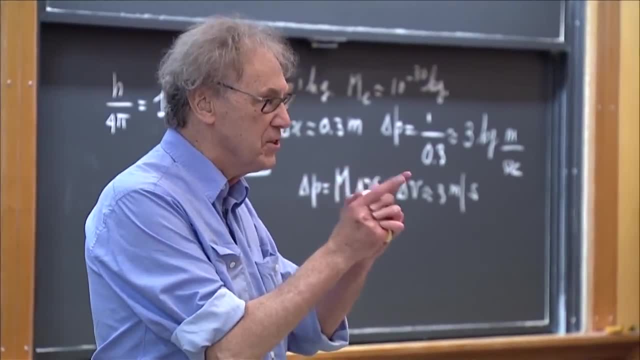 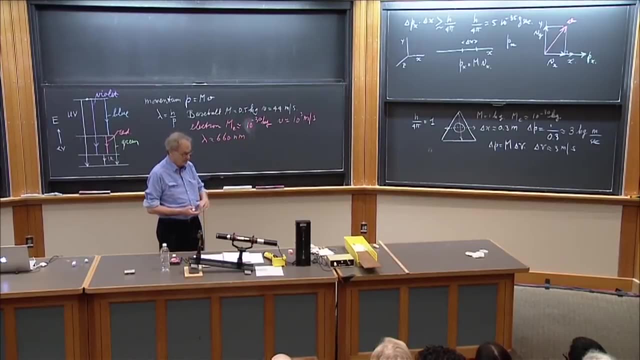 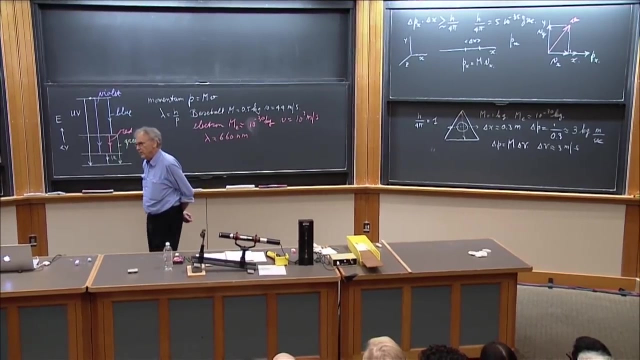 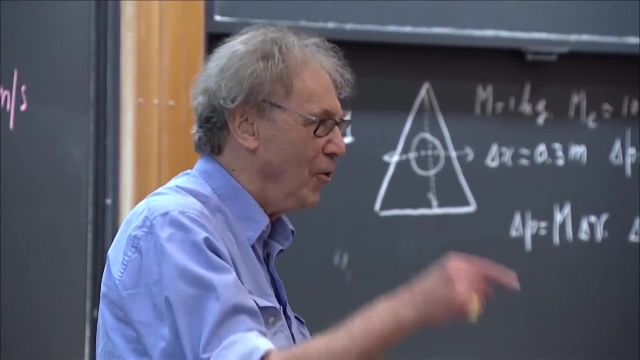 in a triangle, but it is now an electron in an environment which is only ten to the minus ten meters in size. and I do exactly the same calculation using, of course, the correct answer, the correct number of kilometers per second, and that gives the electron energy. think about it. 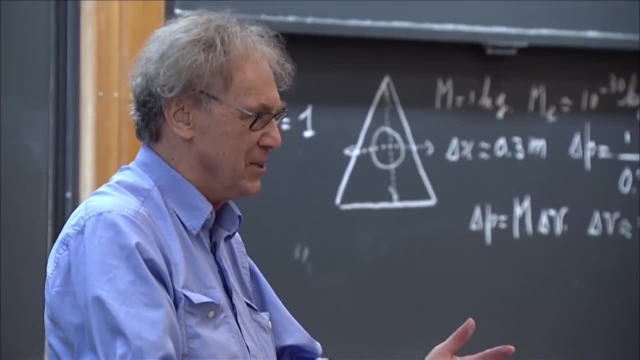 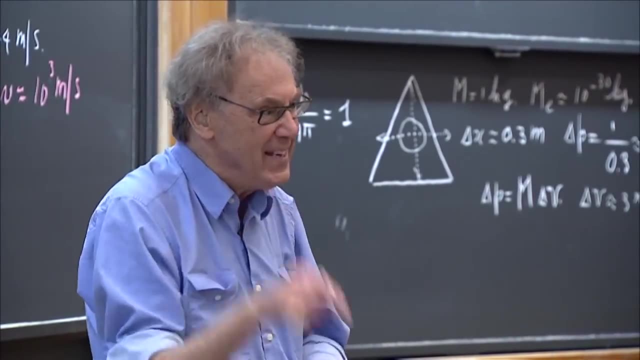 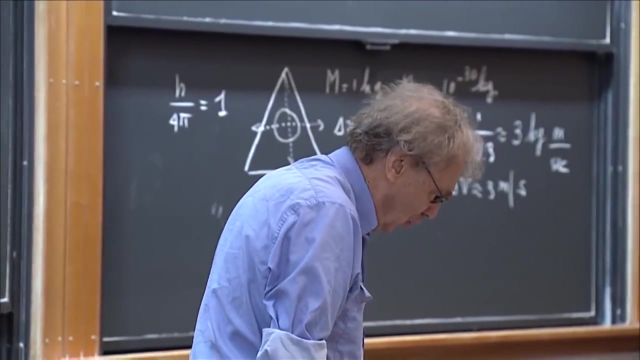 it is Heisenberg's uncertainty principle that says to the electron: you got to move, I will give you energy. the energy of the electron is only because of Heisenberg's uncertainty principle, which is an amazing concept when you think about it. so the entire behavior. 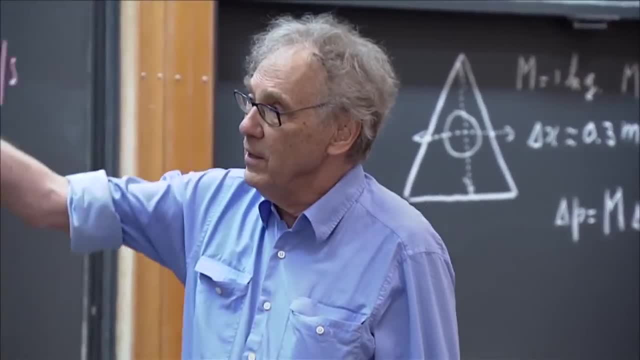 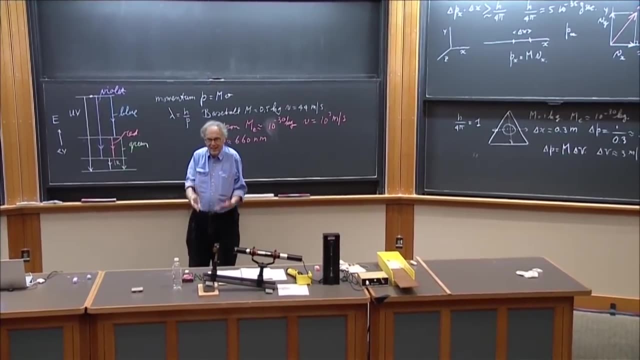 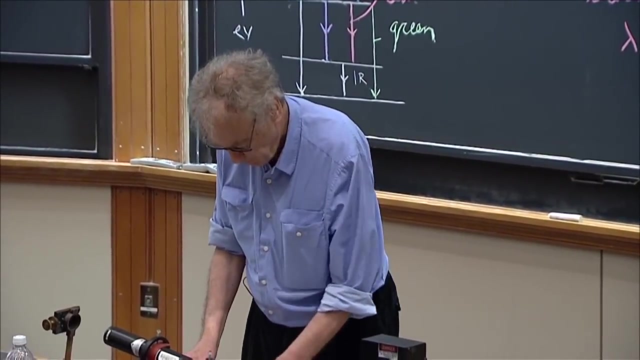 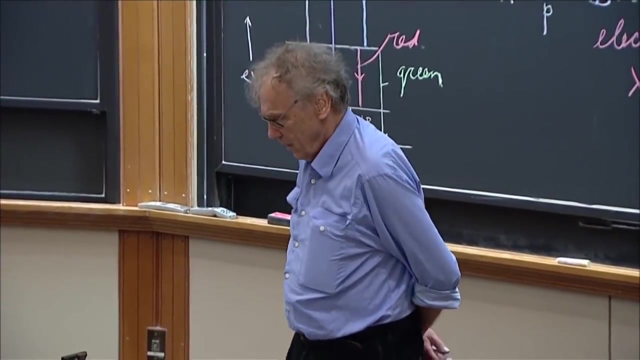 of the atom is dictated by quantum mechanics. the lines that are emitted, the energy levels is quantum mechanics, but the simple fact that the electrons have energy inside the atom is also the result of quantum mechanics. now I'm going to try to demonstrate this and, of course, I already told you. 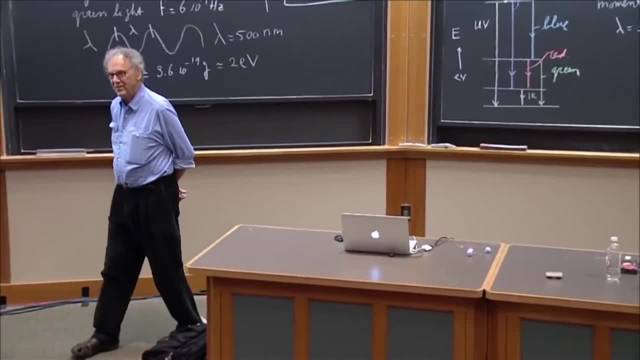 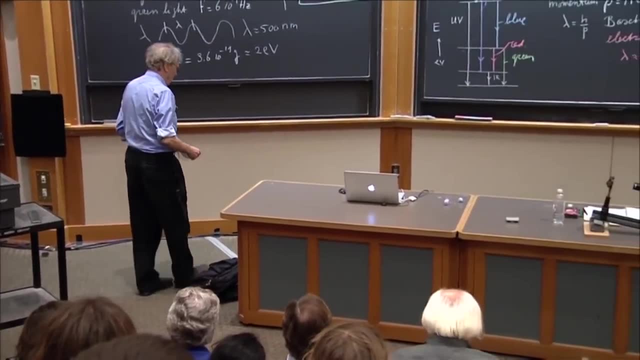 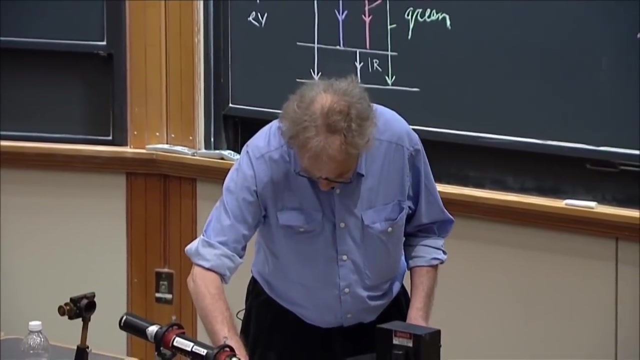 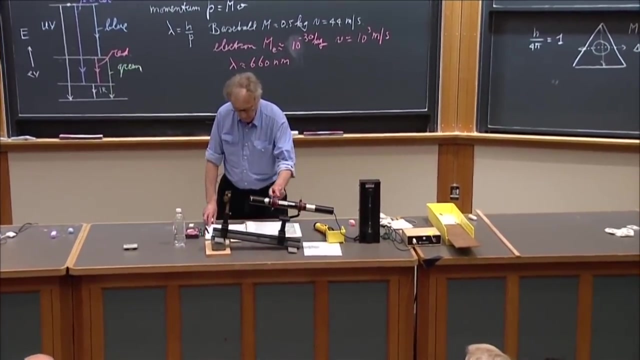 you can't demonstrate any of this in real life because quantum mechanics doesn't work for baseballs and for tennis balls. so I've been breaking my bones for years how I could possibly show this to my students in the classroom convincingly and the way I'm going to do that. 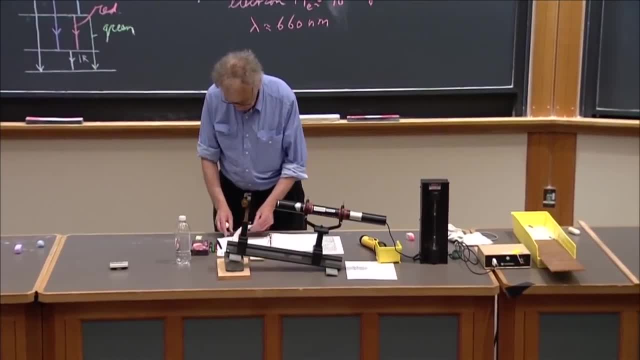 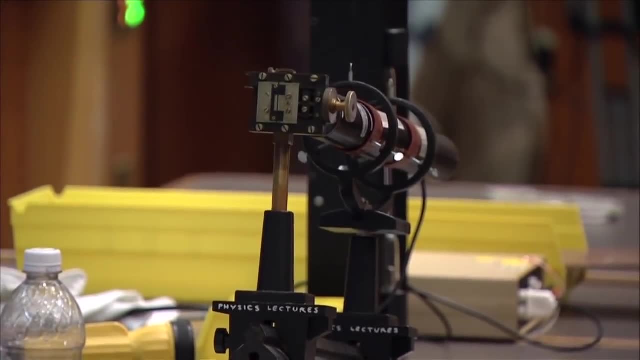 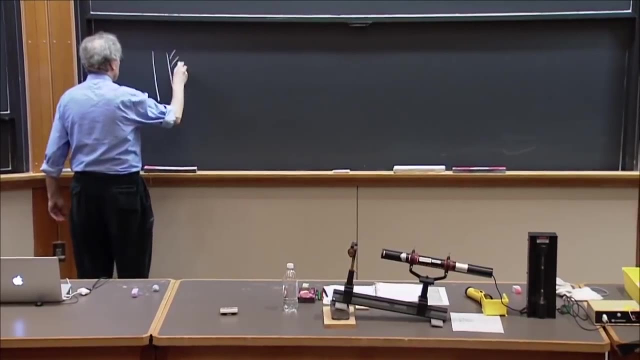 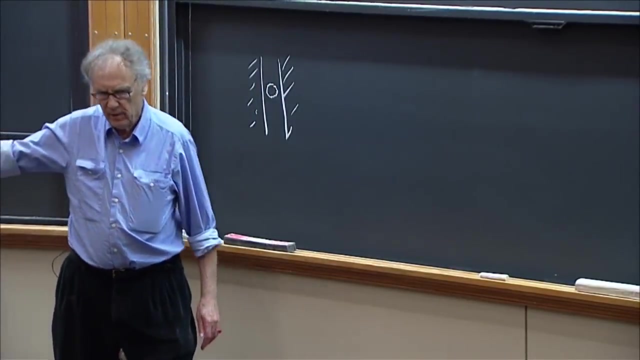 is as follows: I have here a green laser and the green laser is a slit, so this is the slit, so this is opaque and this is opaque, and I shine the green laser through the opening and you're going to see it right there on the screen, no problem. 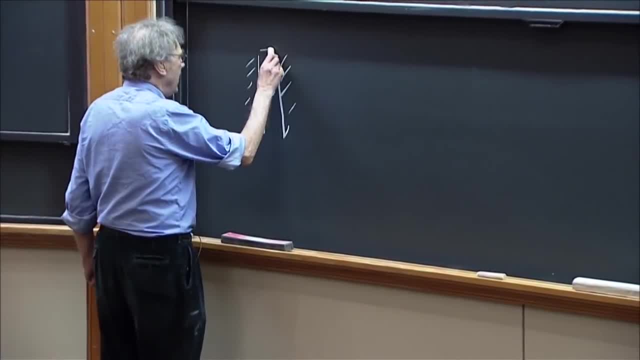 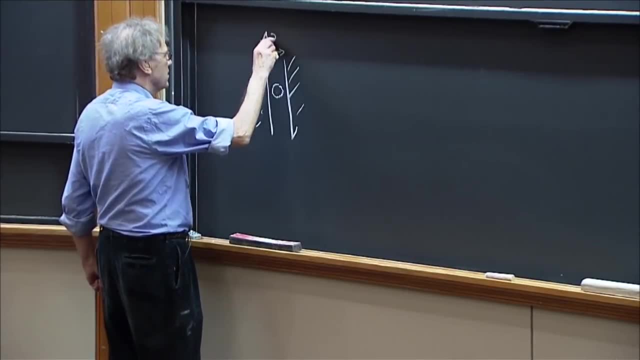 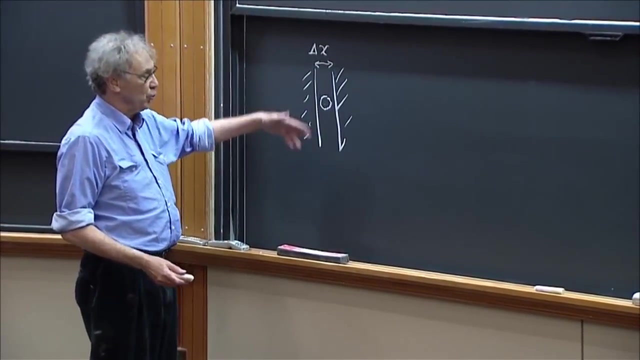 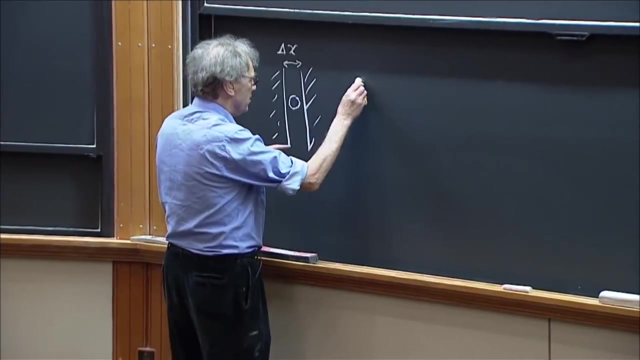 but of course in this direction this beam is a little bit restricted. so I call this delta x. in this direction it's not restricted at all, so I don't even have to think about Heisenberg's uncertainty principle in this direction. this direction is going to become a concern. 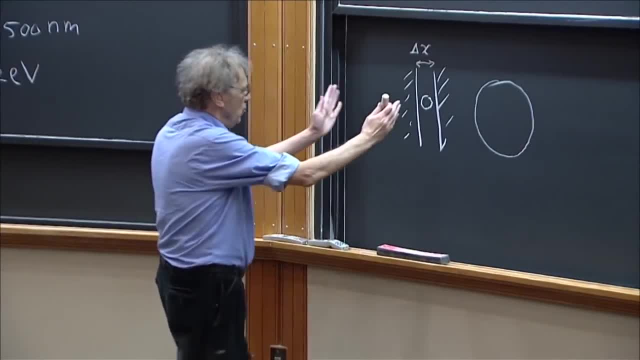 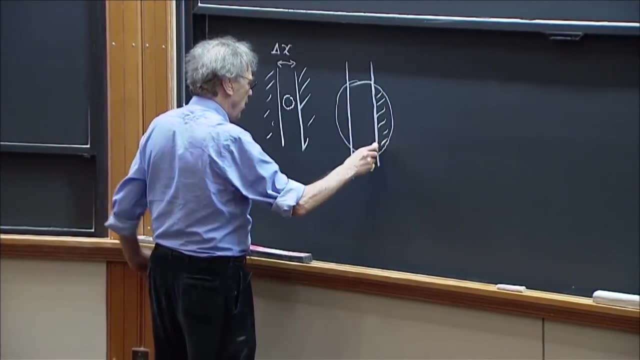 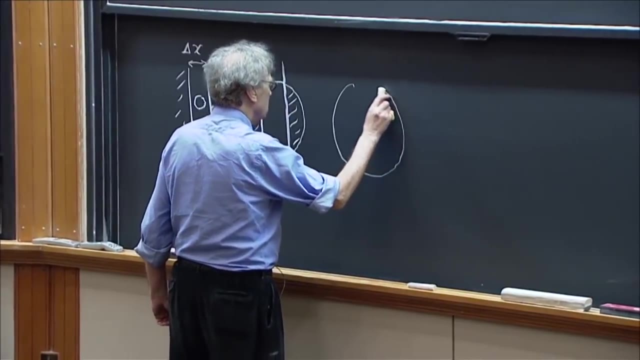 I will blow this cross-section of the light up, because now I'm going to make the slits narrower, so this part of the light you will not see there and this part of the light you will not see there, and then I continue that I make it even smaller. 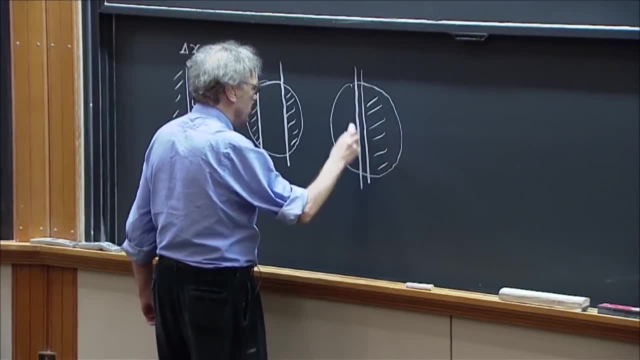 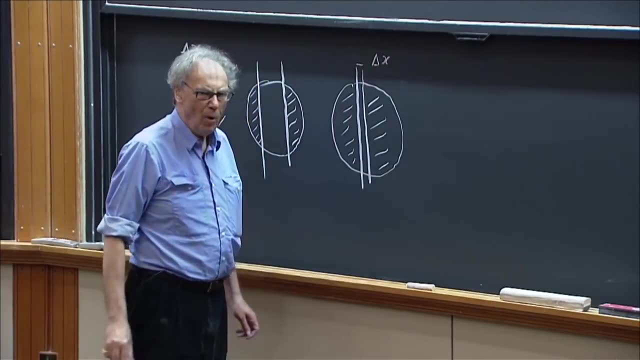 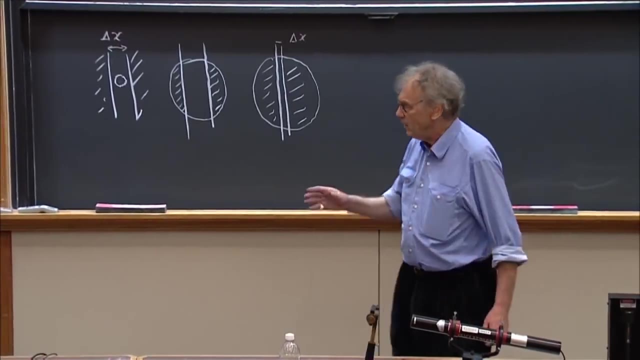 and so this part of the light you will not see, and this part of the light you will not see. but this delta x has become so small that Heisenberg says, uh-uh, you can't do that if x is going to be this small. and this is the x direction. 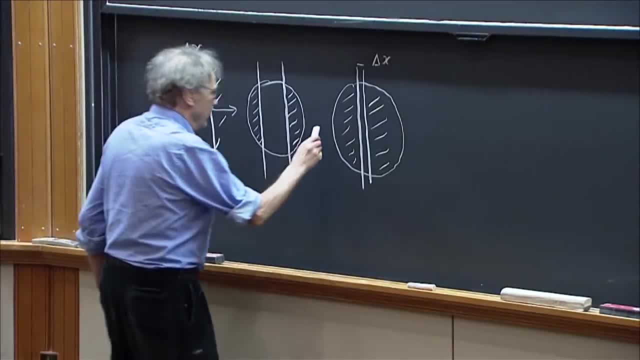 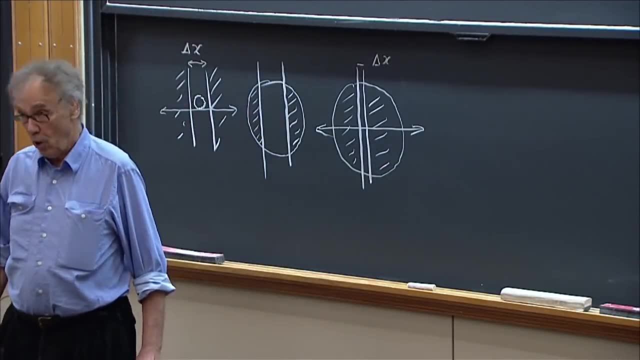 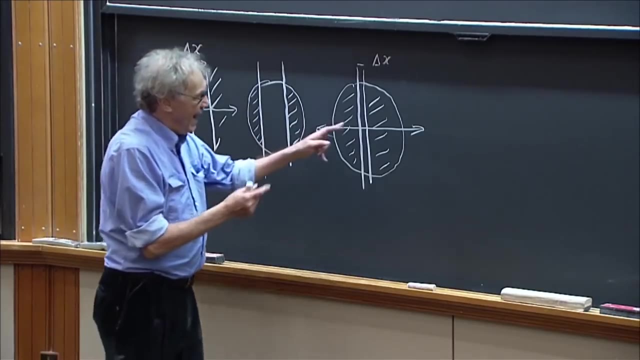 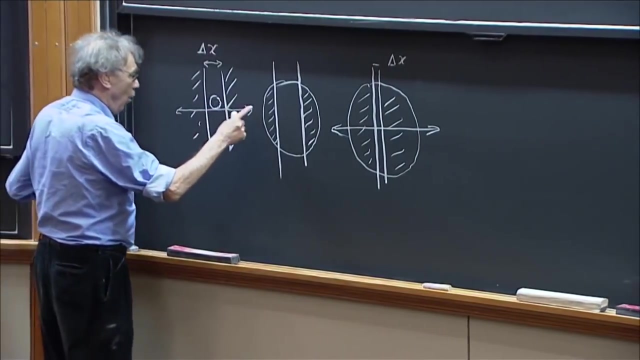 then the momentum of the light in this direction is not well known. and so if the momentum of the light in this direction is uncertain by a large amount, then the light that goes through the slit might easily spread on the wall, but it may come out here or there. 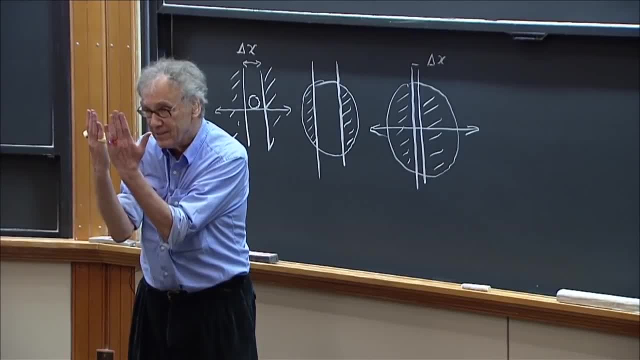 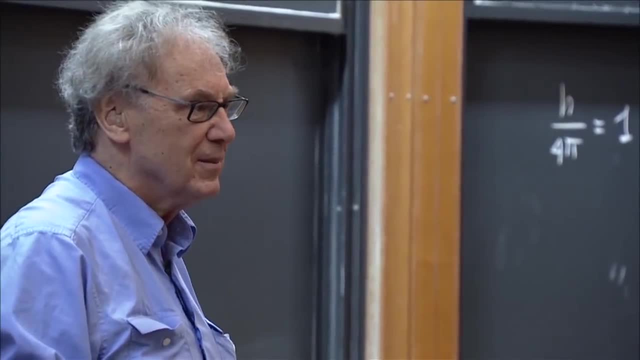 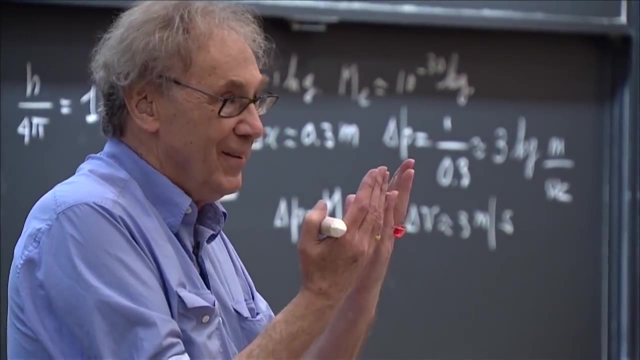 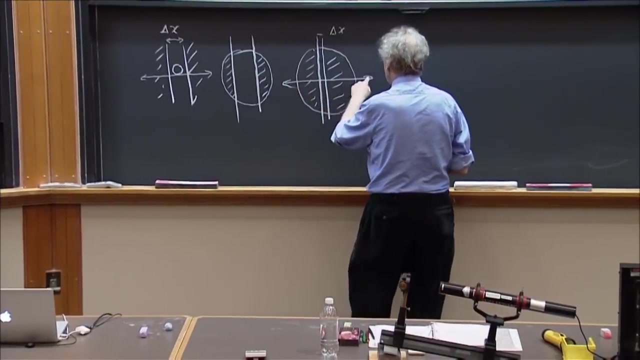 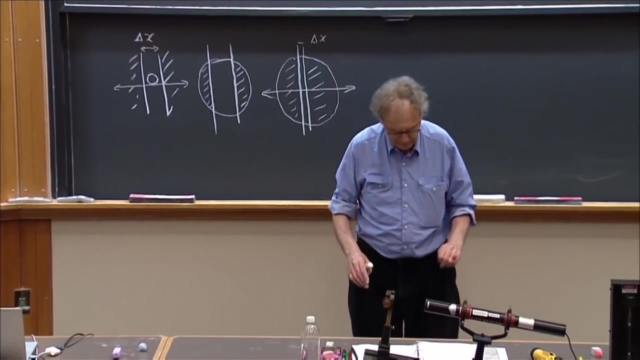 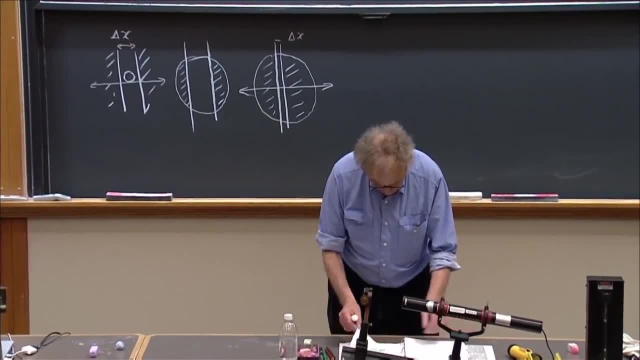 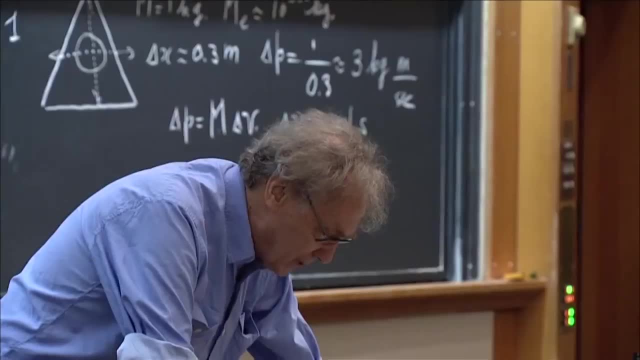 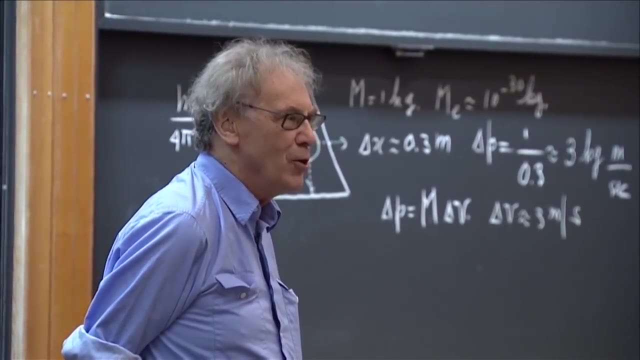 Before I show you this experiment, you may want to ask yourself a reasonable question, and that is: can we apply Heisenberg uncertainty principle to light? In other words, does light have a momentum? And now, looking at John, my friend, who asked me this by e-mail Of: 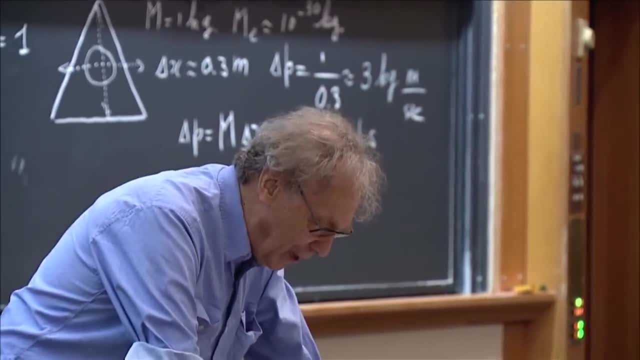 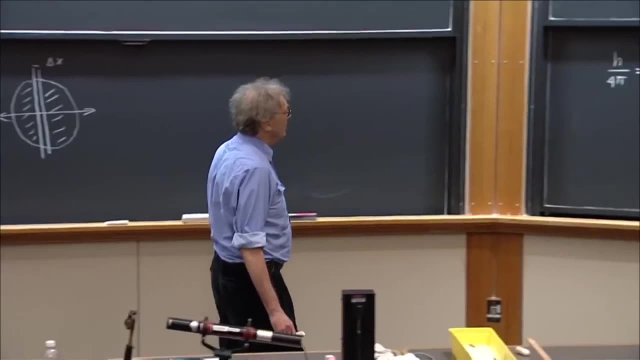 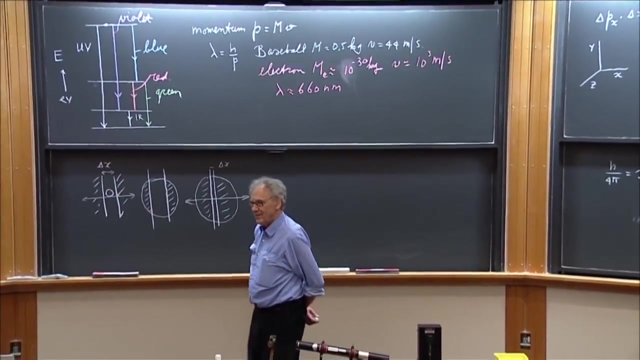 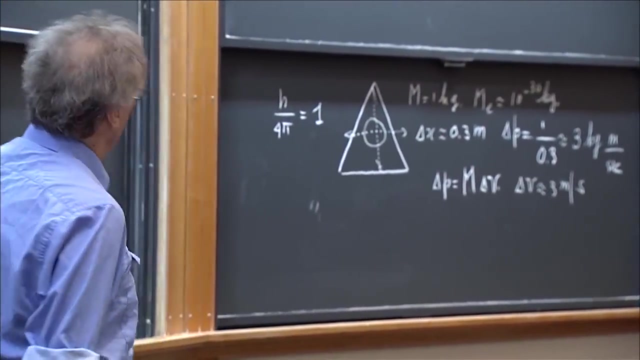 course it does, because light can behave like a particle and all particles have a momentum. But the momentum is not mv, because the mass of a light photon is zero. So now you will say: no problem, the mass is zero, the velocity is the speed of light. 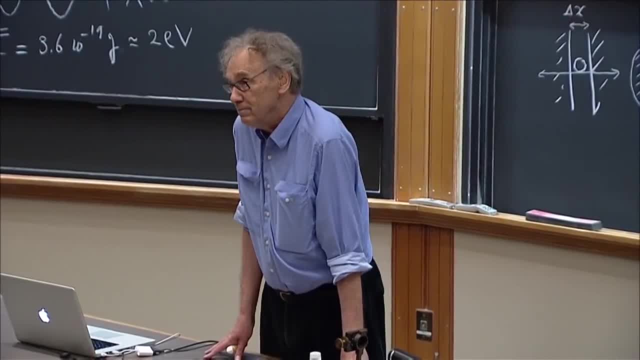 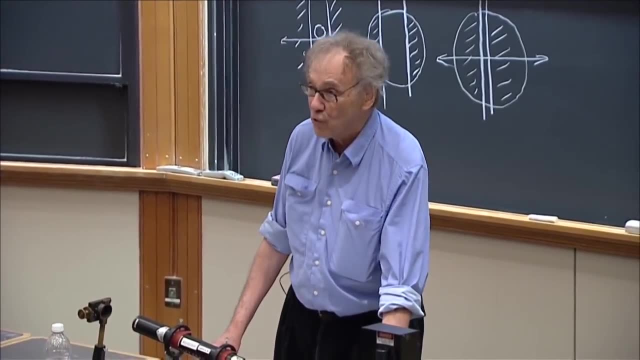 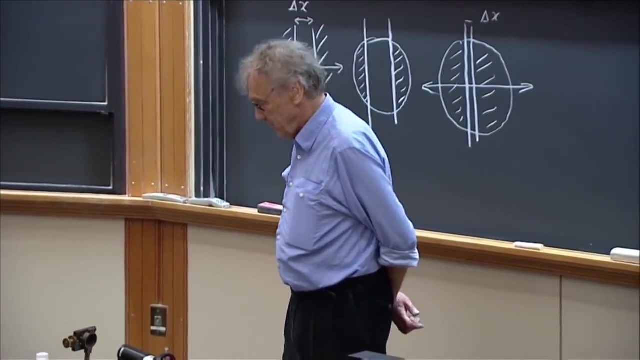 Well, zero times. the speed of light is still zero. However, a light photon does have momentum And I could show you the equation. but I said to myself, why should I? Because you learn nothing. you will see just one other equation. 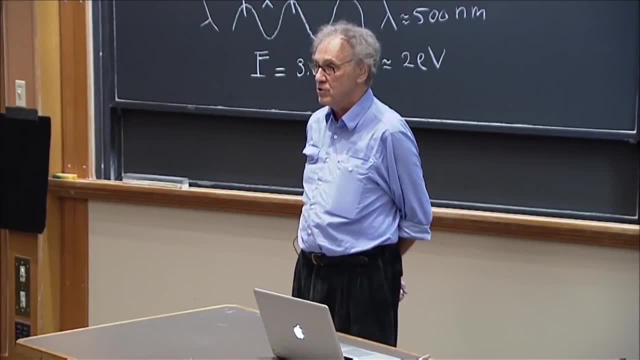 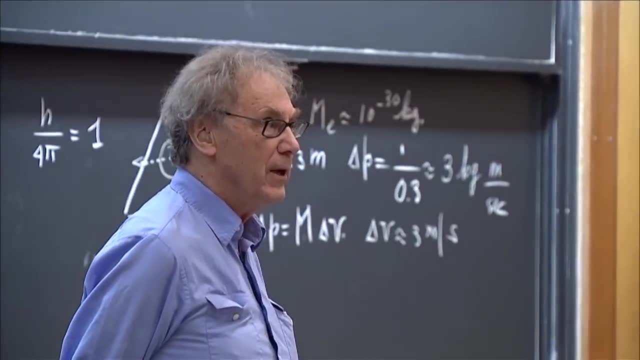 and you have nothing already seen so many, so you get even more confused. So it should be enough for me that you accept the fact that light does have a momentum, And if you want to know what it is, you can come to me after this lecture and I will tell you what it is, Because my 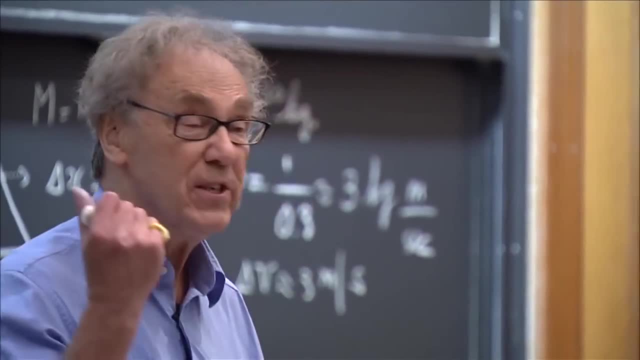 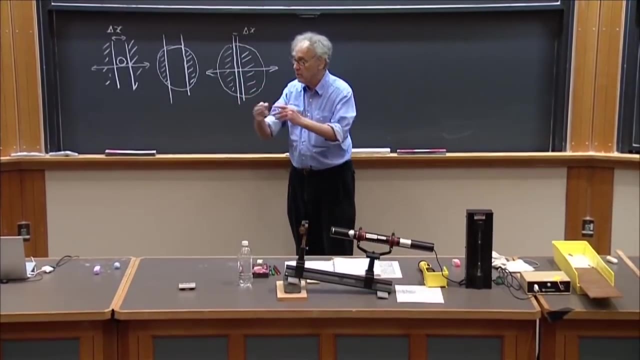 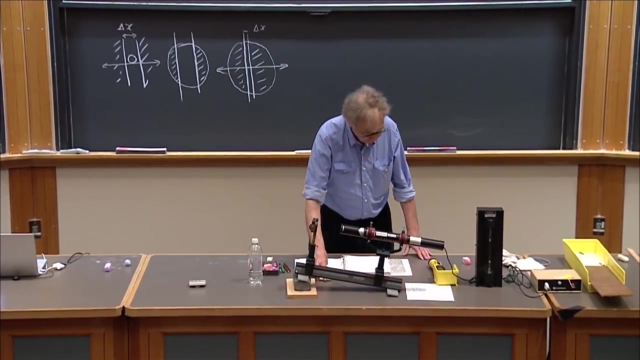 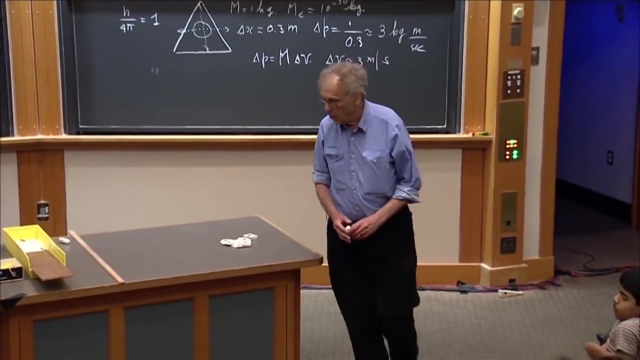 conclusion is: yes, you can use this experiment. Light has a momentum And therefore what I just told you- the narrower the slit, the wider the light will spread- is going to be realistic. So I'm going to move to the other side of the table and I'm going to turn on. 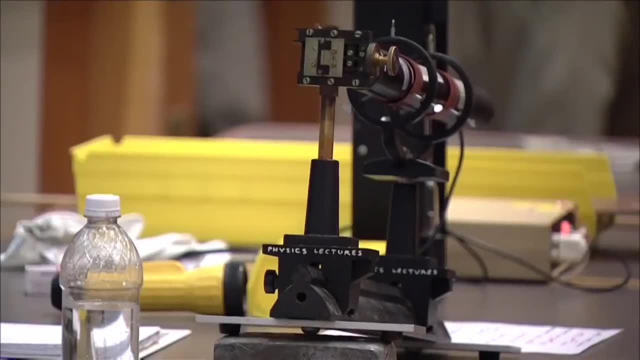 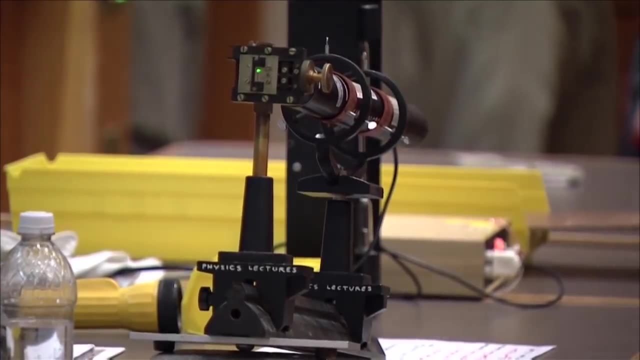 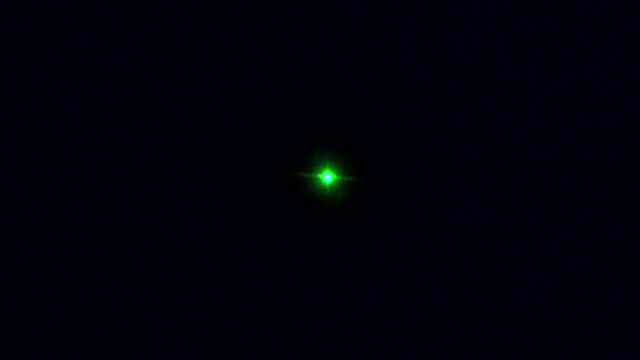 the laser It's supposed to show up. There it is. Turn the lights off, Bill, I think. Okay. So now the slit opening is enormous. The slit opening is a few millimeters And if you do your homework with Heisenberg's uncertainty principle, there's no effect yet of the spreading. 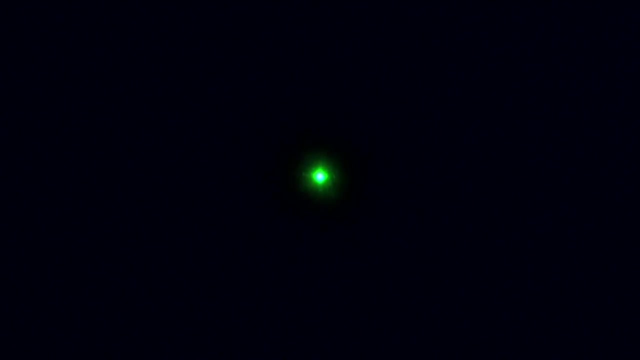 of the light. But now I'm going to make the slit narrower And in the beginning you're going to see some dashed lines On the left and on the right And I would like you to ignore those dashed lines for now It is really the center bright point that I want you to concentrate on, That center. 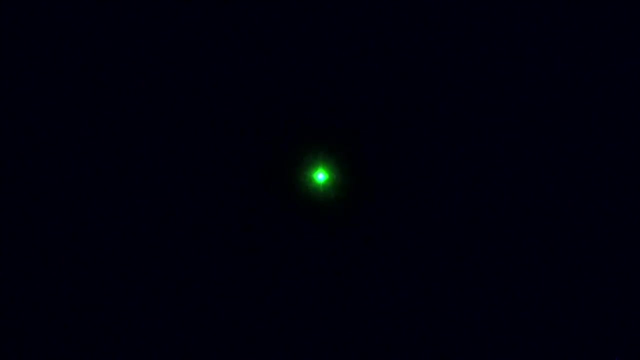 bright point. I am making the slit smaller and smaller and smaller and smaller. I hope I turned in the right direction. Did I open it Okay? Yeah, Do I go clockwise or counterclockwise? Okay, there we go, There we go. 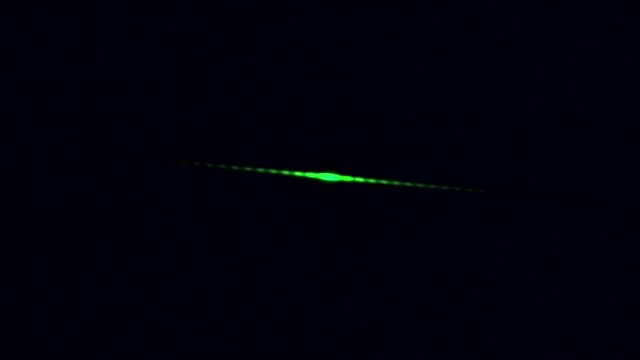 Look at the center portion. Look that the center portion is now going out in horizontal direction. You see it's getting bigger. You're seeing it's getting bigger, it's getting wider. Heisenberg is having lots of fun. now He knows this has to happen. 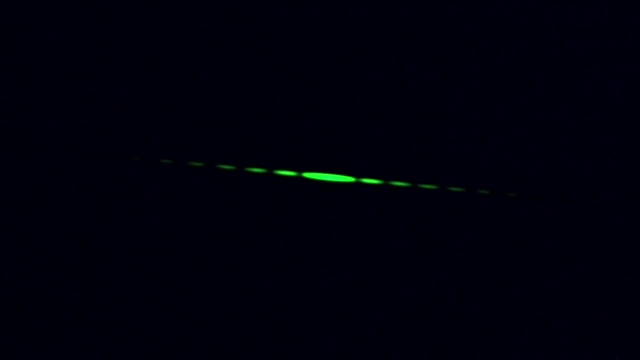 I'm making it smaller And I'm making it smaller, And that center part gets bigger and bigger and bigger. Forget the dashed lines, right, It's now almost ten centimeters. I've made some changes, I've made some calculations. 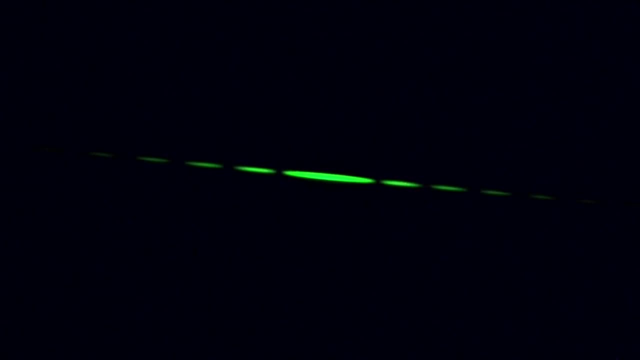 And they show that if the slit opening is five microns, then the central portion of the light on the wall is about ten centimeters. So the opening must be approximately five microns now, And yet what you see on the wall is about ten centimeters. 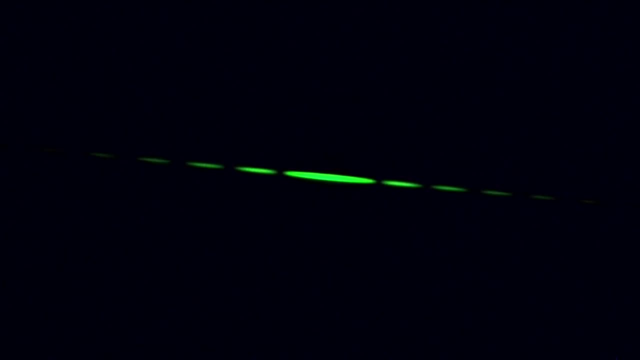 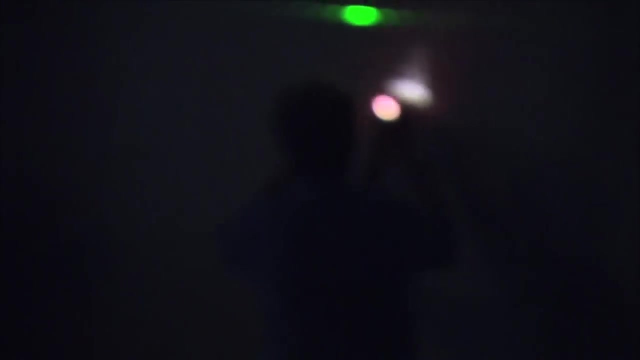 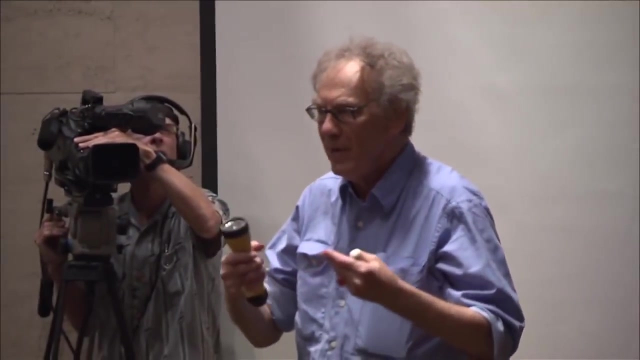 which is about 20,000 times larger than the five-micron opening of the slit. I've made some calculations. It's this wide- I hope you can see it- And that is the result of the fact that you are now limiting this light. 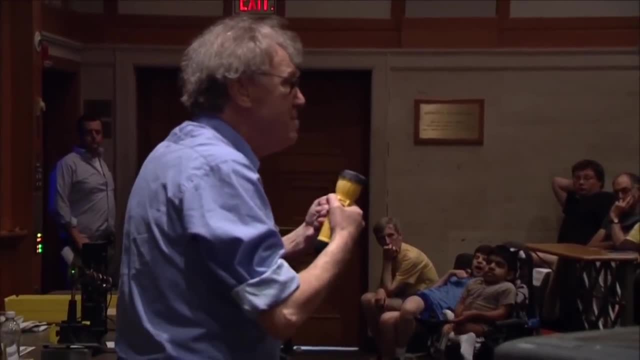 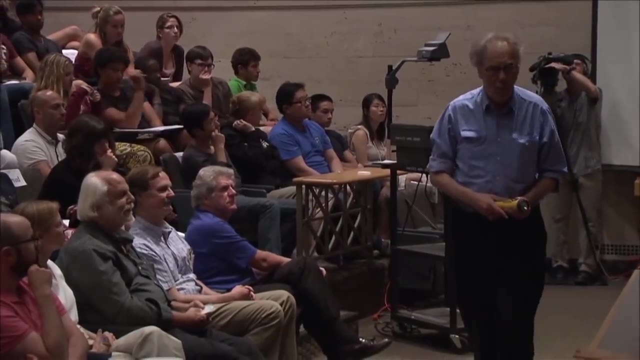 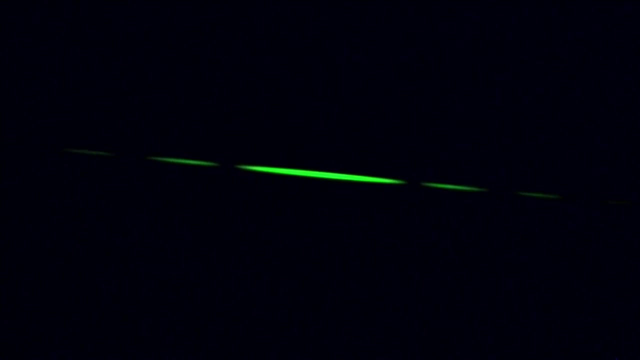 in the x direction to go through an extremely small opening, and the price you pay that the momentum of the light becomes uncertain. I can even go one step further and I need to go to make the slit about one micron. Look at that central portion. 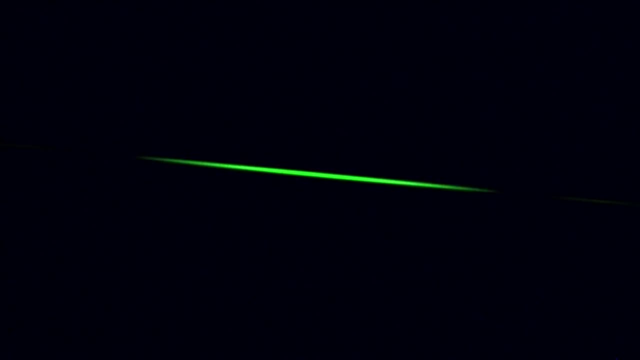 One micron. I calculated, if it is one micron, that that middle part should be about 25 centimeters. Oh sorry, 50 centimeters. That's right, Should be 50 centimeters, And I think I can reach that point. 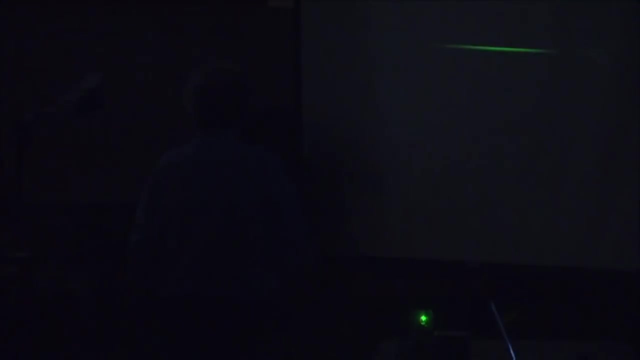 and you can still see it. This is about 50 centimeters. Don't accuse me that it is so faint. Can you imagine that any light goes through a slit which is one micron wide? That has nothing to do with Heisenberg. 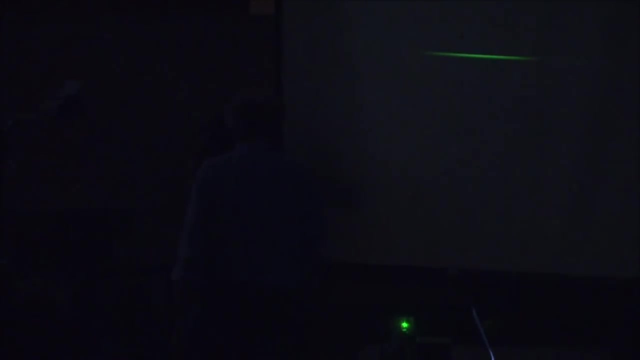 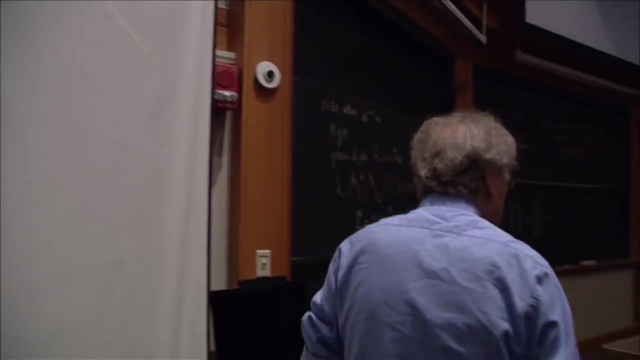 That's simply the fact that I don't let much light through. But you see, now that that central point is now this big, It's about 50 centimeters. 50 centimeters Only because it's being squeezed through a one-micron opening. 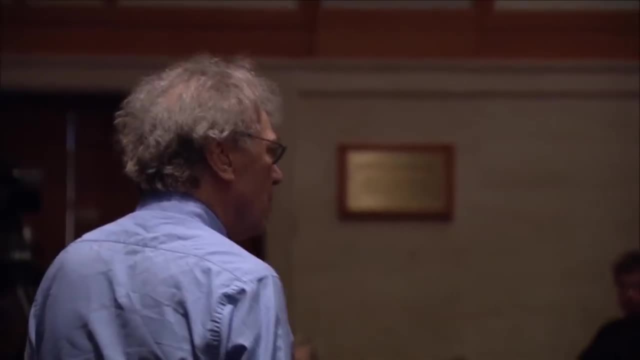 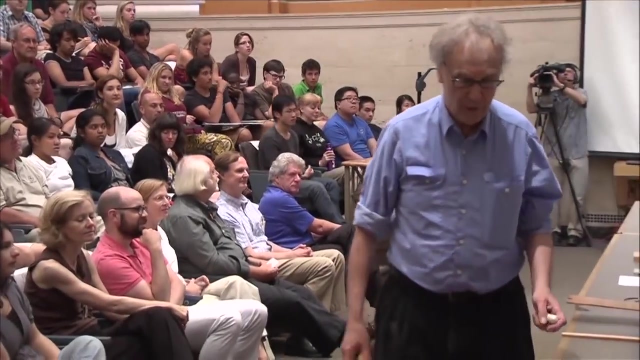 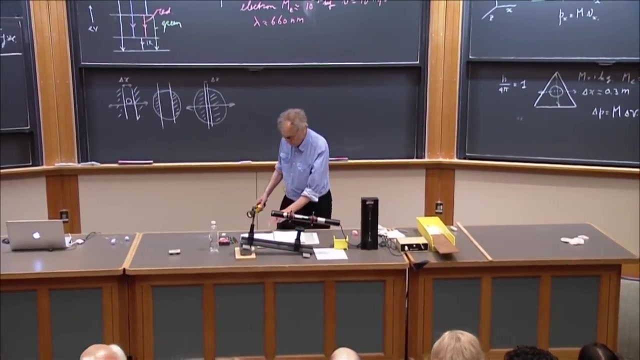 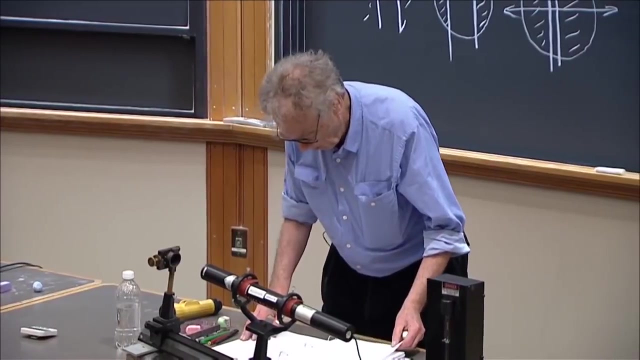 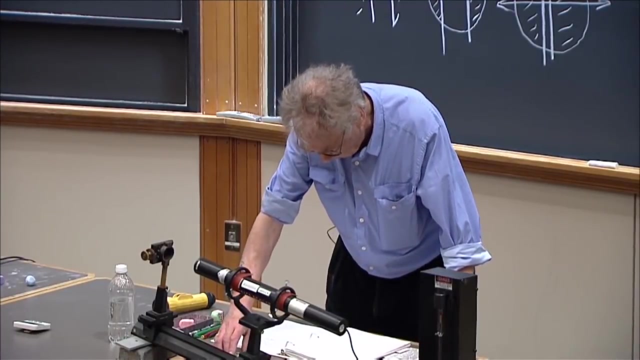 That is Heisenberg's uncertainty principle, An amazing and very non-intuitive consequence of quantum mechanics, Because he derived his uncertainty principle from the equations of quantum mechanics. So you've seen the quantization of energy levels and you've also seen Heisenberg's uncertainty principle. 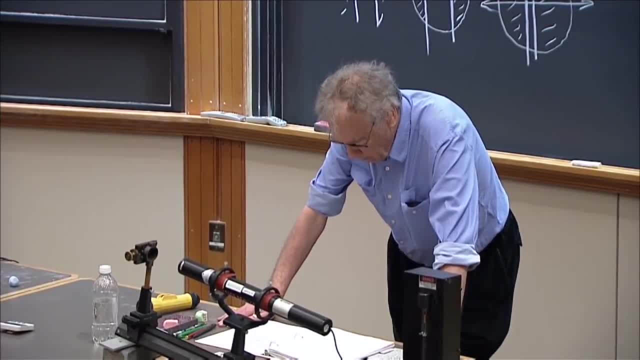 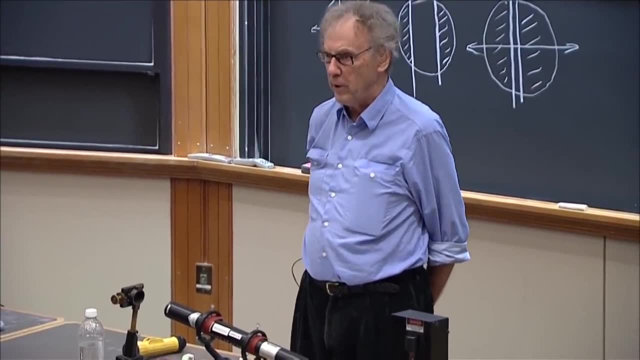 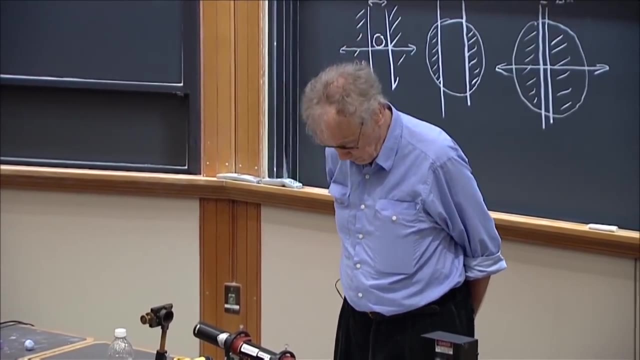 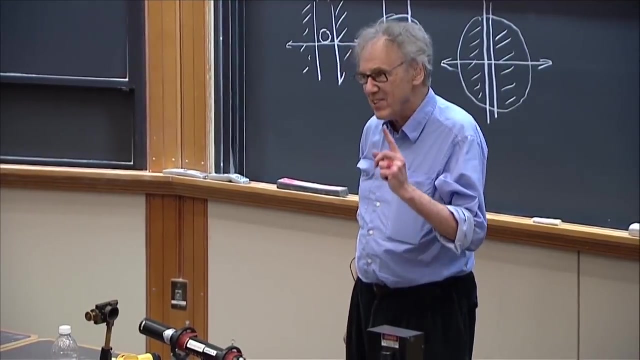 The spreading of the light that I have shown you was already explained in the 19th century with classical physics, way before quantum mechanics, And we do that using the technique of what we call diffraction. Yet all I wanted to show you is that the spreading of the light is entirely consistent. 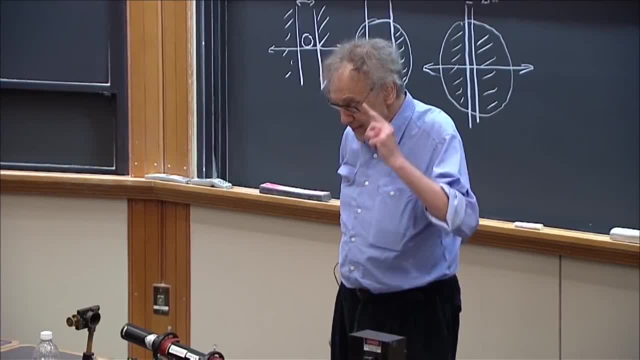 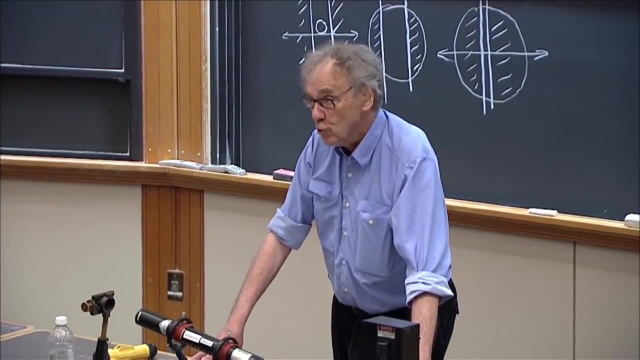 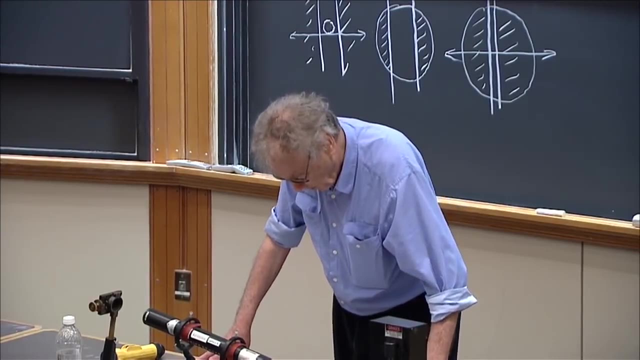 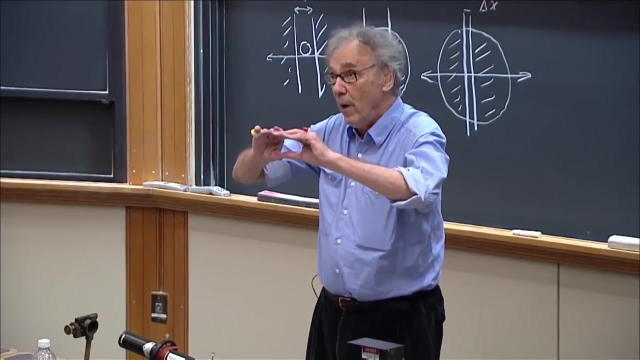 with the uncertainty principle, And it better be, Because you could not construct any experiment that would violate Heisenberg's uncertainty principle. Quantum mechanics cannot predict where a particular photon will end up on the wall, But it can predict if you make long exposures, one photon at a time. 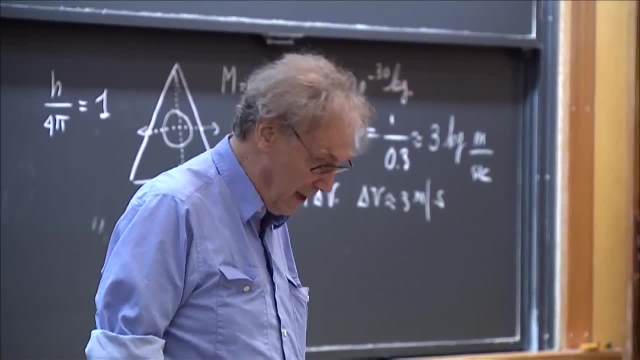 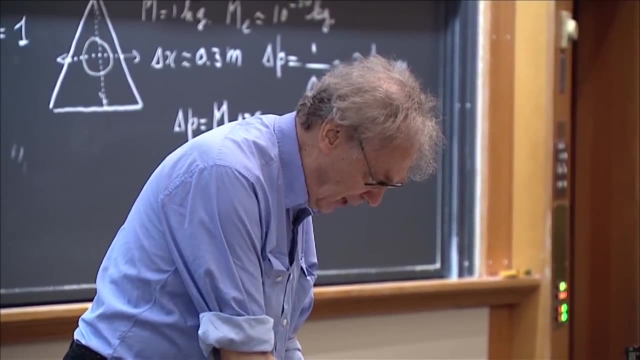 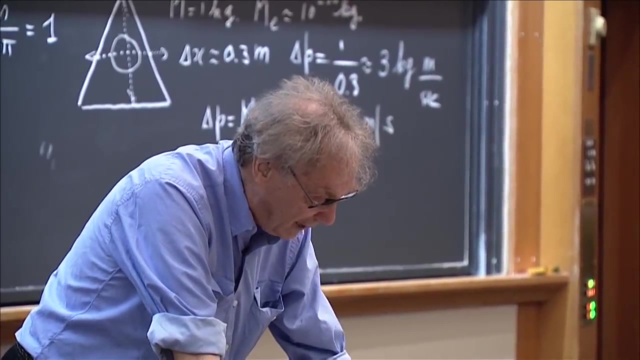 what ultimately the shape will be that you saw on the screen. But you cannot predict where an individual photon will land, And this idea that you cannot in advance predict what a particular photon will do is a very non-classical idea And it drops off the wrong way. 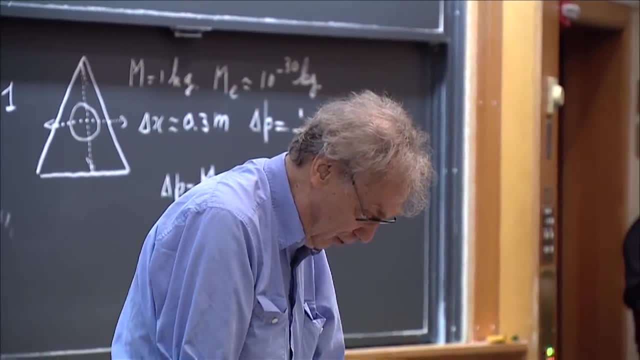 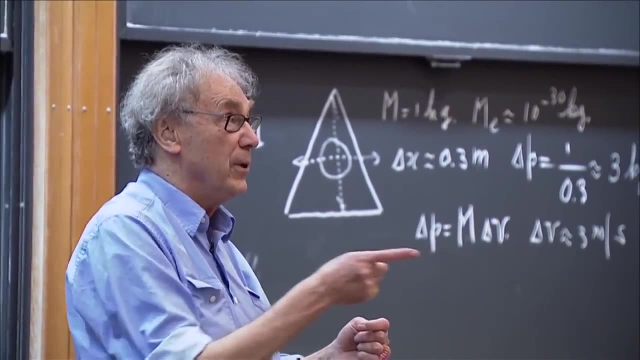 Our classical way of thinking- not only yours but also mine, of course- is that if you do an experiment, the same experiment a hundred times, you would expect the photon to always end up at the same location, And that is not true in quantum mechanics. 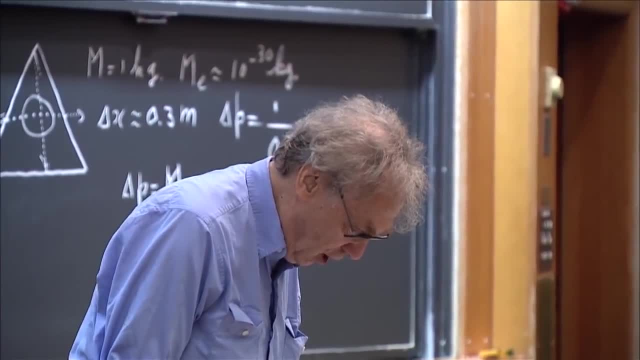 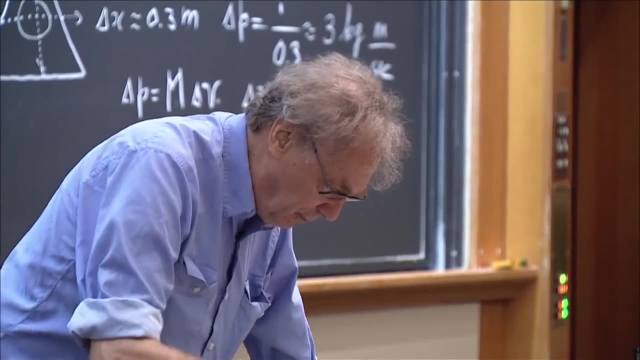 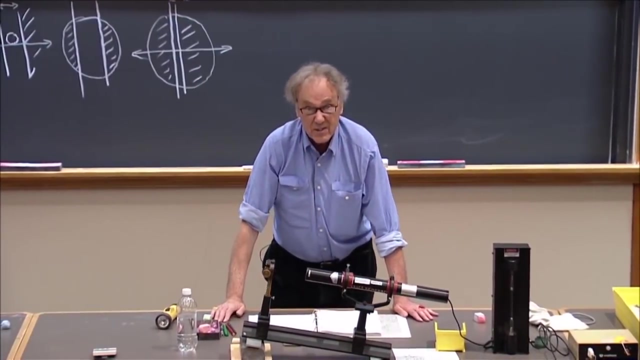 And Einstein had great problems with this idea of not knowing precisely what would happen, And he had endless discussions with Bohr and others to convince them that there must be something wrong with quantum mechanics. And his famous words were: God does not throw dice. 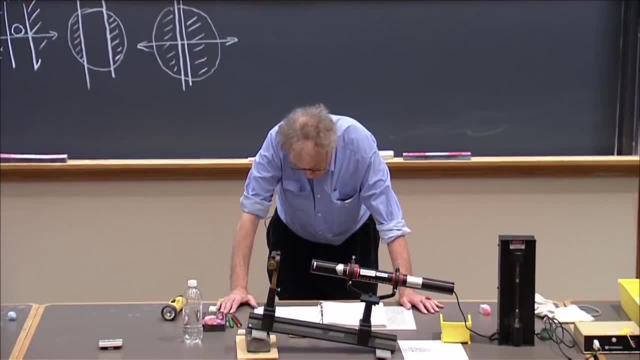 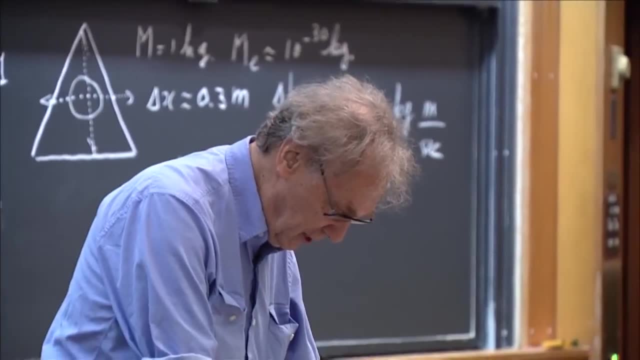 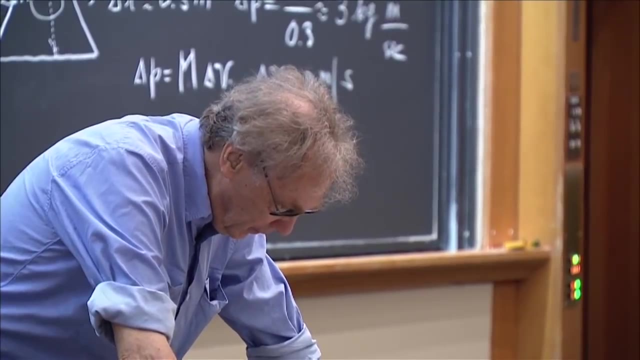 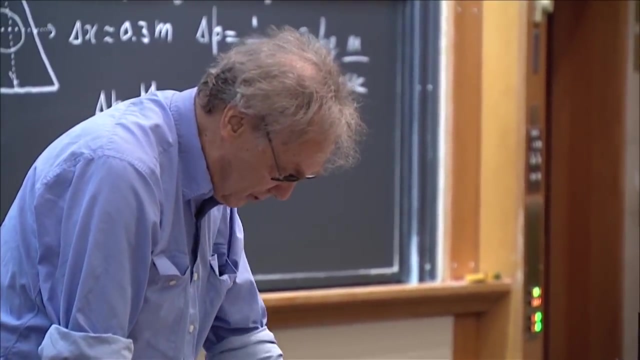 And this was his way of saying. it is ridiculous that the outcome of a well-controlled experiment is uncertain. It's now a hundred years since quantum mechanics was developed And we know that God, if there is one, does throw dice. However, God is bound to the rules of quantum mechanics. 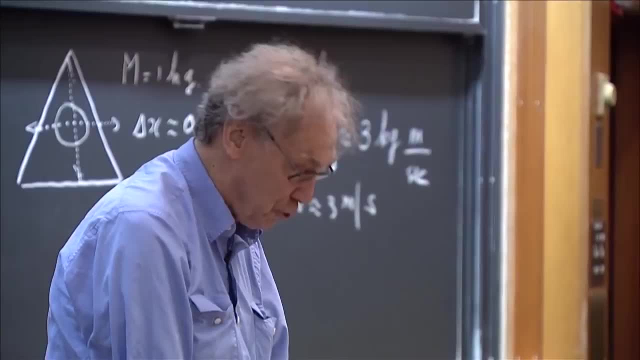 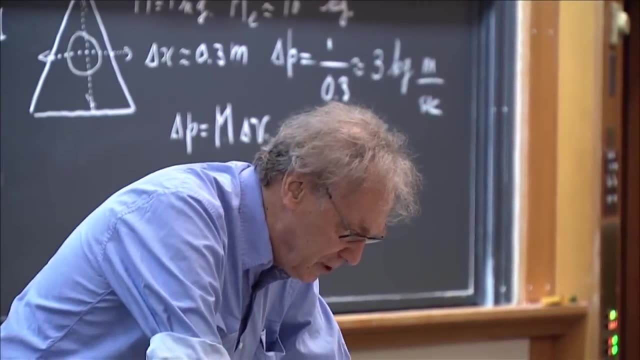 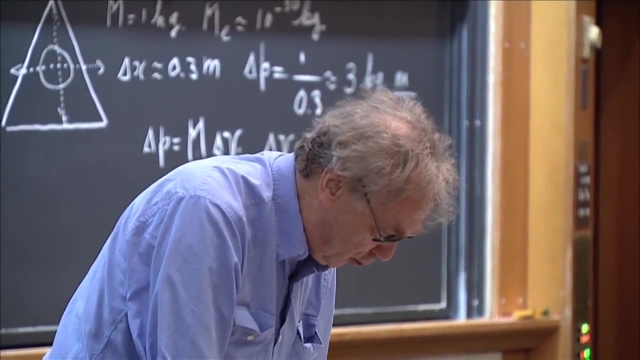 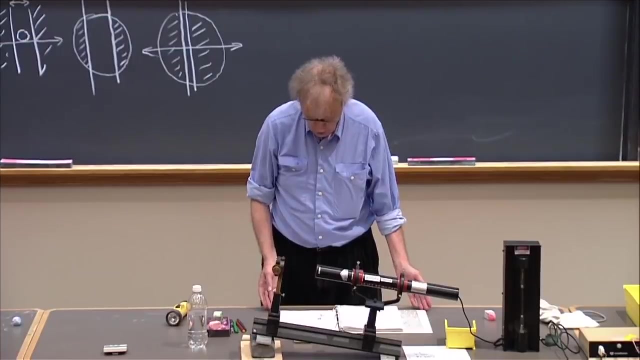 And even he cannot violate Heisenberg's uncertainty principle. Quantum mechanics is a bizarre world that we rarely experience in our daily lives. Yet that is the way the world ticks, And atoms and molecules can only exist because of quantum mechanics. Therefore, without quantum mechanics, 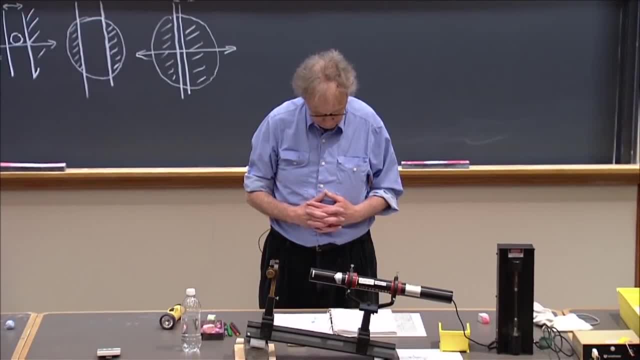 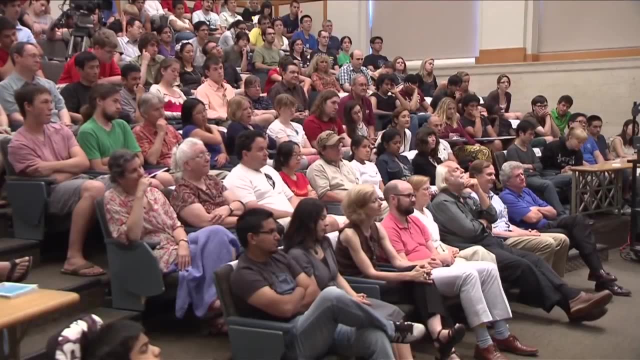 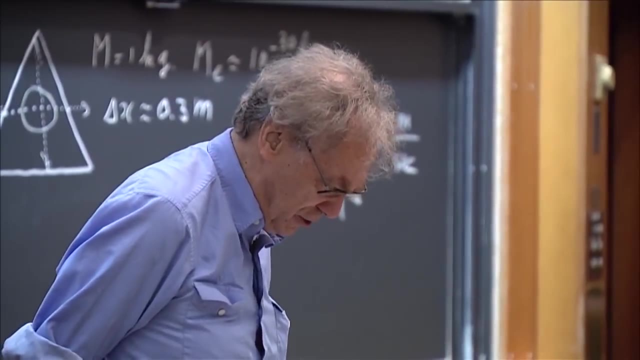 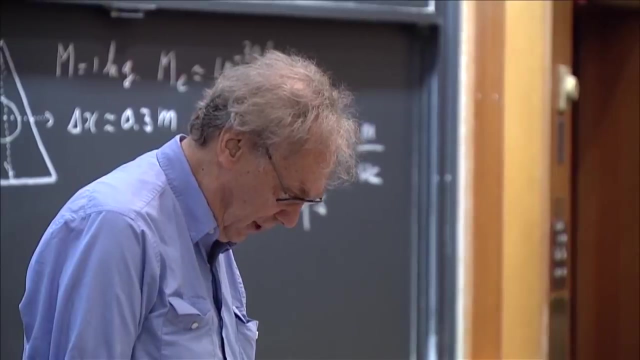 you and I would not be here. I hope this will give you something to think about, But I warn you because thinking about it may give you sleepless nights and headaches- It has given me countless. But that may be necessary if you want to eventually evolve. 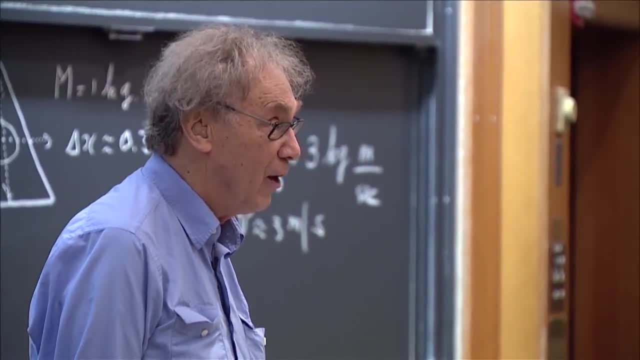 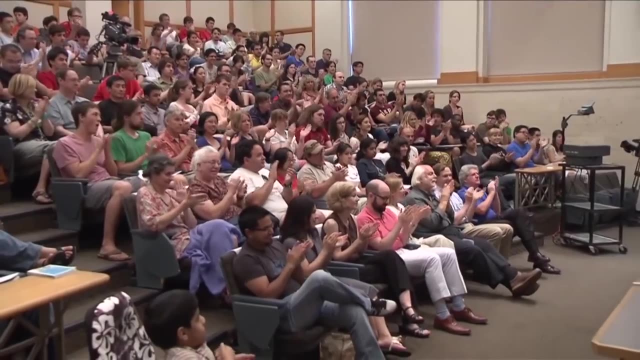 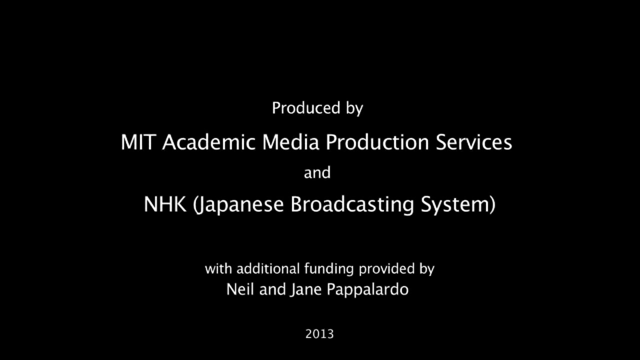 as independent thinking scientists, And I hope that someday all of you will Thank you. Subtitles by the Amaraorg community. 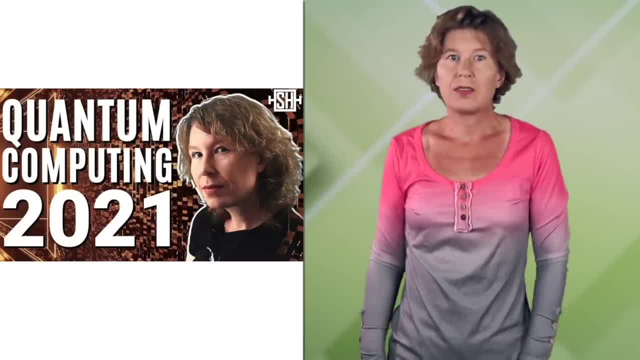 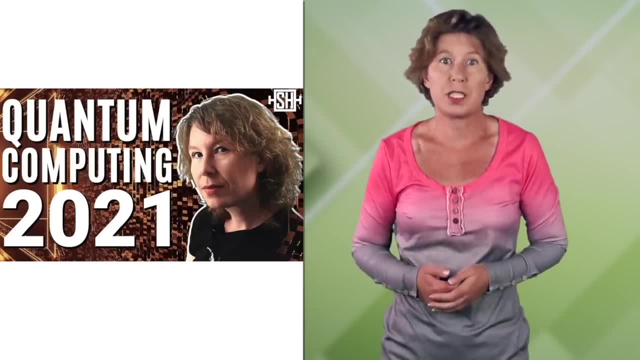 It's been a while since we talked about quantum computing. The last time I did an overview video was in 2021, but that might as well have been in the stone age. so much has happened since. What's going on, What's new and who's saying what? That's what we'll talk about today. 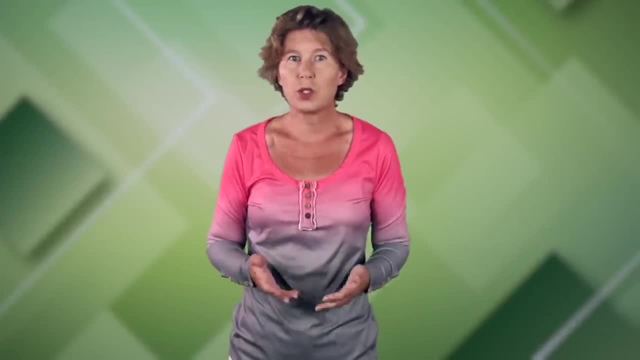 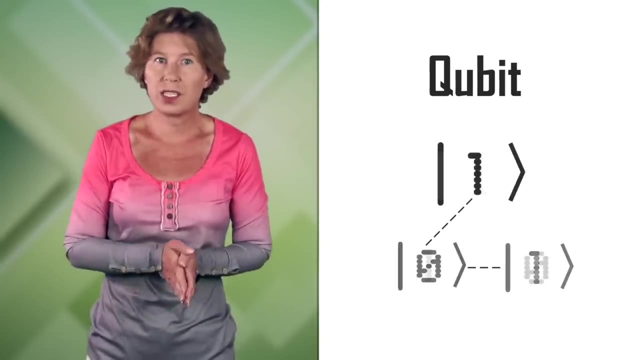 First things first. quantum computers calculate with quantum bits- qubits for short. that can become entangled. Entanglement is a type of correlation, but one that requires quantum effects. So you can't build a quantum computer with legos. I'm sorry, But with 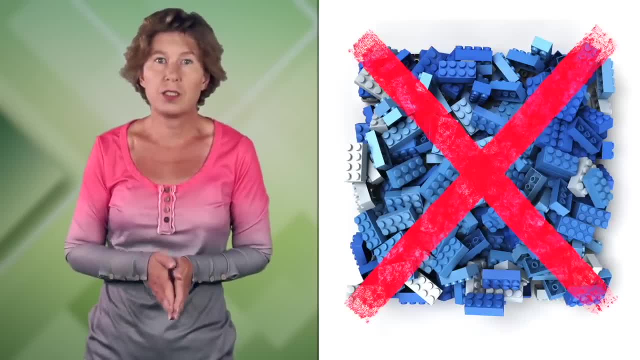 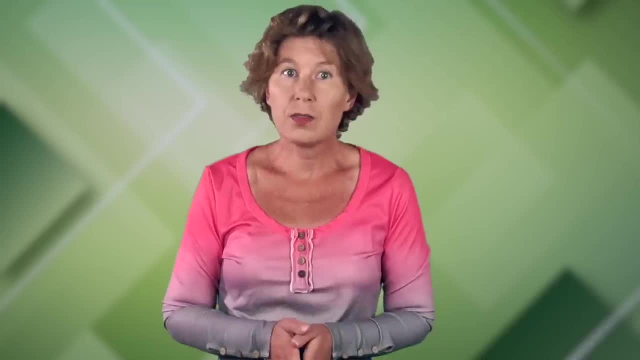 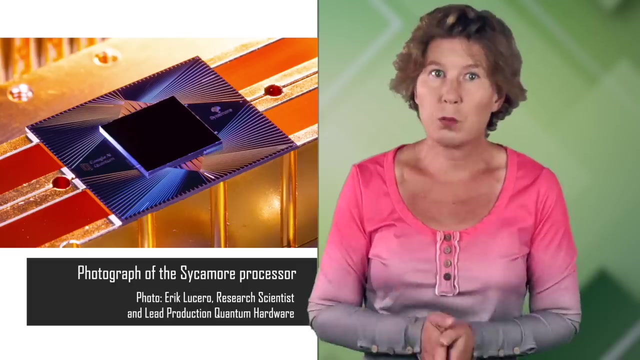 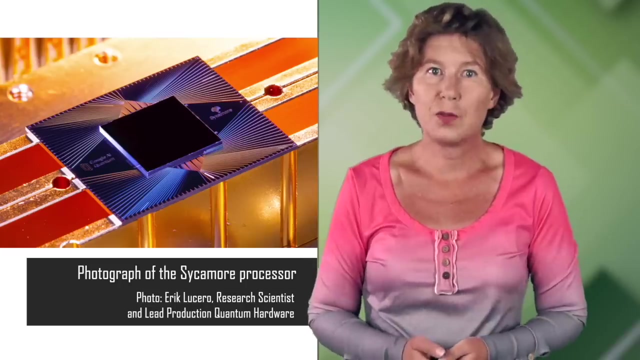 entanglement you can encode a huge number of states into the qubits and that can speed up the solution of certain mathematical problems. The relevant word in the previous sentence is certain. Quantum computers only bring an advantage for certain mathematical problems. The most important ones are in the areas of quantum chemistry, logistics, finance. 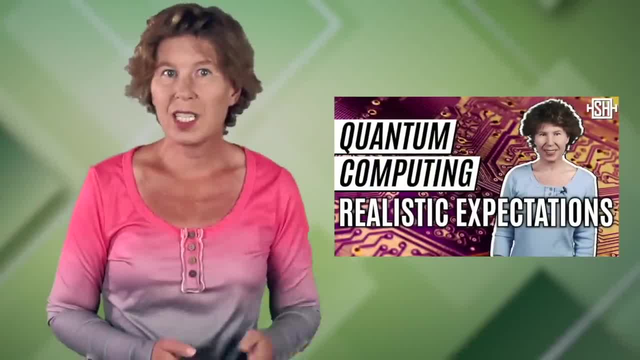 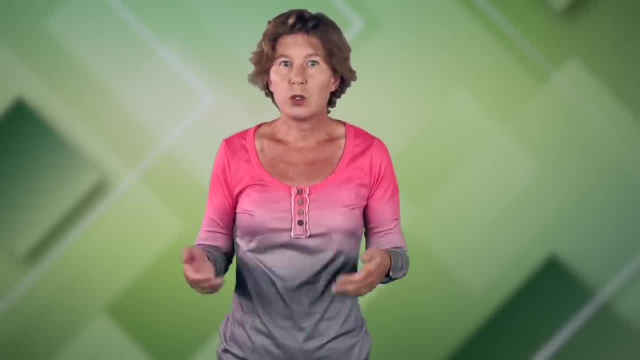 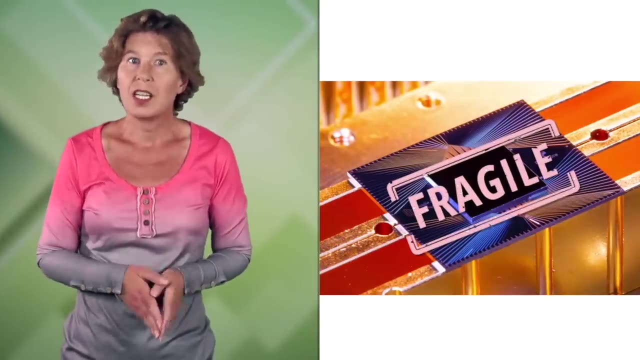 and code-cracking. I made a video about just what type of problems those are previously. The other relevant thing you need to know about quantum computers is that those quantum states are really fragile. They get destroyed easily by the smallest perturbations. 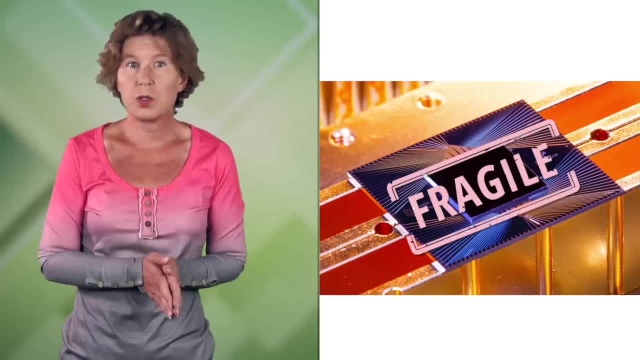 and you need to get the calculation done before the quantum states have been destroyed. It's kind of like this: If you're doing something with quantum computers, you are not going to get anything right. You actually need to get your heads around the work. 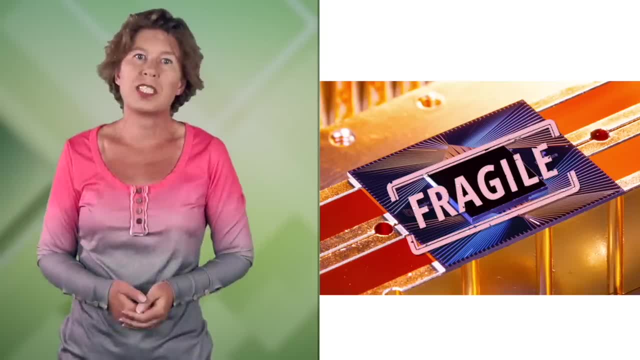 what and what you're doing is the most important part of it. But in any case, don't take too much of it, like when you have to talk very fast to get out what you want to say before you forget about it. Now, what was I about to say?